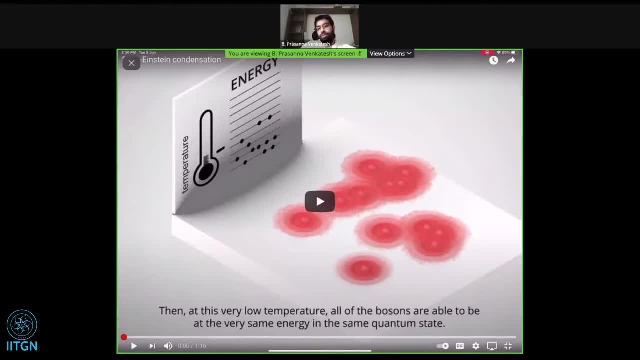 right. So yesterday we began with a very cartoonish picture and we went into a little bit more details. We went into a very specific way to describe a Bose-Einstein condensation for a non-interacting ideal gas of bosons. So I thought today I would want to remind you of 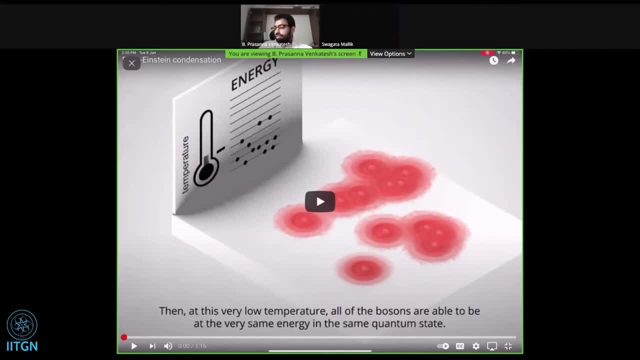 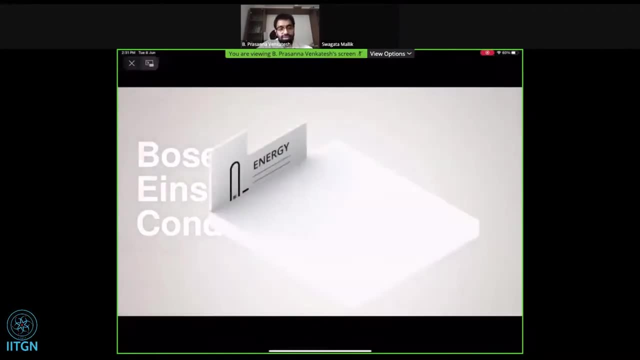 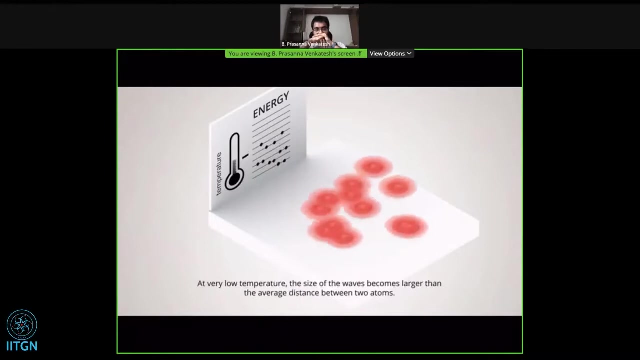 the cartoonish picture. to begin with I thought, instead of words, here is a very nice video that I found of a Bose-Einstein condensate- a cartoon. yeah, so i guess this is a very nice. 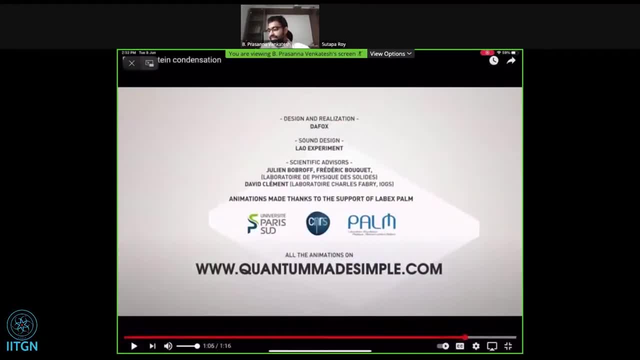 uh, production of this video. this is done by cnrs. uh, some people from france have been doing it. it's very cool. i there are many such sort of basic quantum stuff. they explain using such videos. you might want to check out more of this, but i hope this really captures in some sense. 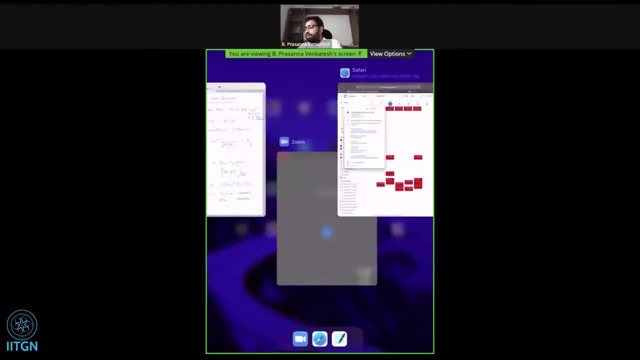 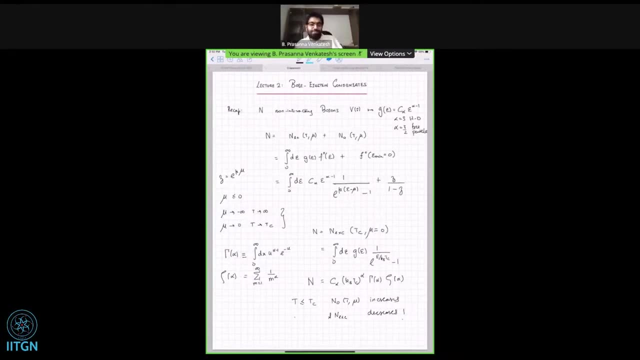 the idea of a boson strain condensate that i was talking about last day, and and- and i don't know if you heard the sound, but they've also, uh, in the sound it was very clear they were actually also making the pitch of the sound. 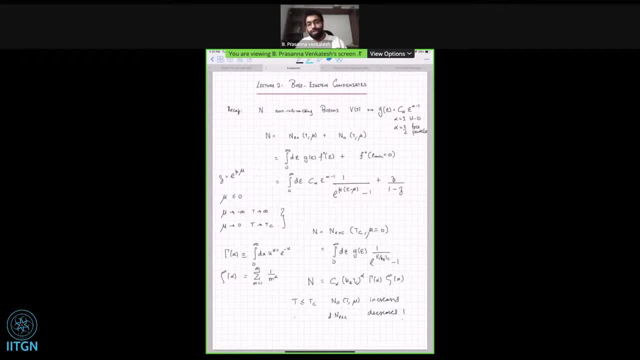 that the atoms were making uh more and more. the frequency was becoming lower uh as the atom settled down into the lowest states, and so on. so it's very well done video, but i hope that was the cartoonish picture we started with and then we moved on to something a little bit. 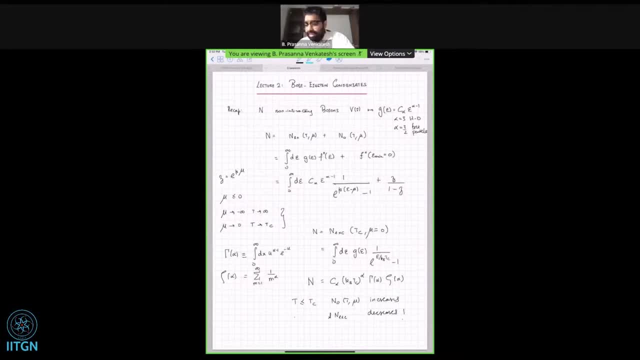 more mathematical, the idea we said we'll describe things for an uh situation of n non-interacting gas of bosons which are in some external potential v of r. this potential could be essentially no potential, just a box that means it's a free particle, or it could be a harmonic oscillator with some non-isotropic 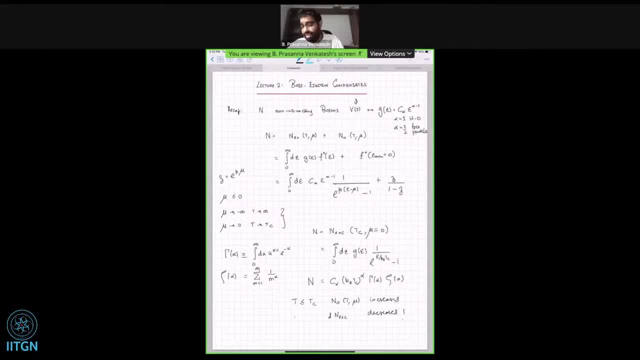 frequencies in xyz. and either way, basically we found out that the key quantity that we get from the single particle potential is the single particle density of states g, of e, which goes as c alpha e to the alpha minus one. and alpha takes the value of c if you have a harmonic oscillator and it takes the value three by two if you have a free. 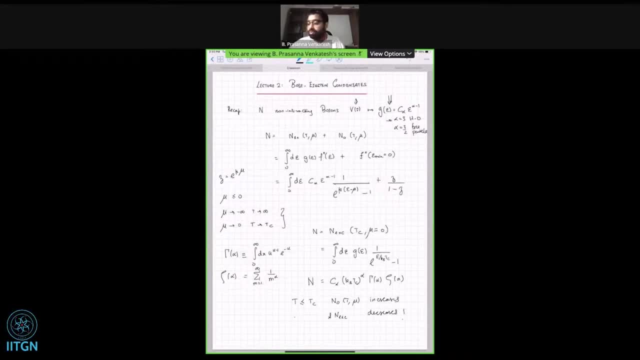 particle in three dimensions. okay, using this, we built up the right equation to describe the total number of particles that we have using the bose distribution function, and one can split up the total number of particles in the right way into basically all the particles that are in the 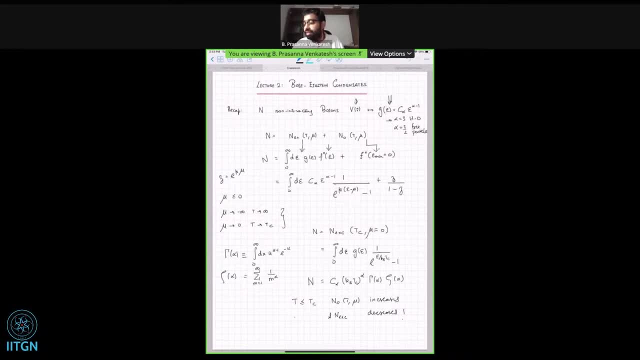 excited states versus all the particles that are in the ground state or the lowest energy state of. so we have taken the lowest energy state to be zero for simplicity, which is exactly valid for free particle, for harmonic oscillator. we are ignoring the vacuum energy. and because this bose function has to be positive, because it just counts the number of particles in a given single, 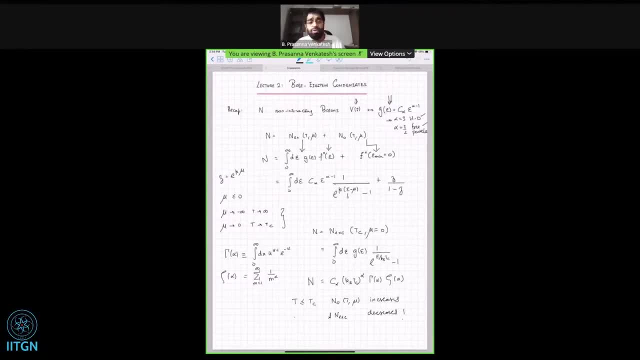 particle energy level. our mu has to always be less than or equal to the lowest ground state energy in the single particle potential, in this case zero. and what is boson stein condensation? basically the following phenomenon: when your temperature is very large, your chemical potential is very small and as in magnitude is large, but value is small and negative close to. 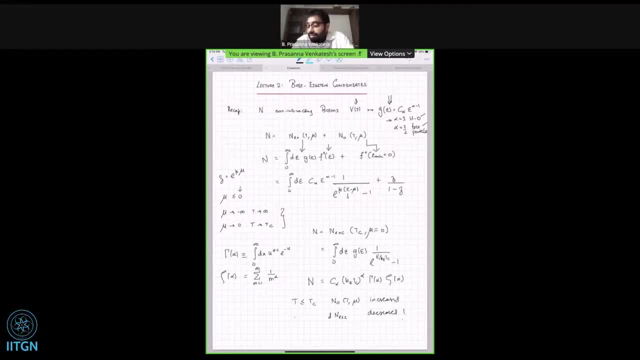 minus infinity in some sense, and basically all of your particles are distributed amongst the excited states. so essentially there is no occupation in the ground state because z is e to the beta mu, and you can see that z by one minus z when mu isept, and you can see that there is no. 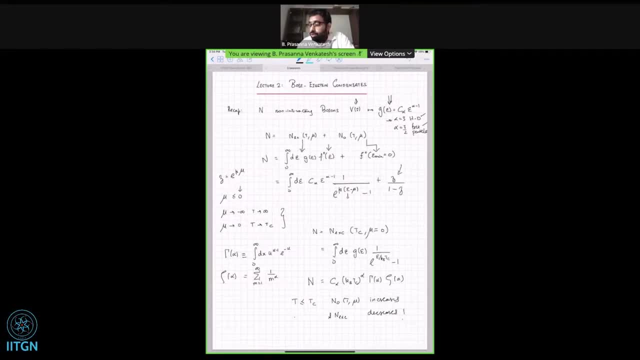 occupation in the ground state, because z is e to the beta mu and you can see that z by one minus z minus z when mu is with. so basically, what happens is that the Correcteon is rule in. unlike van Gaeko, I want to be like an irish linguist, like understand how he holds right andsta tem or الم ton, and it is a ri. 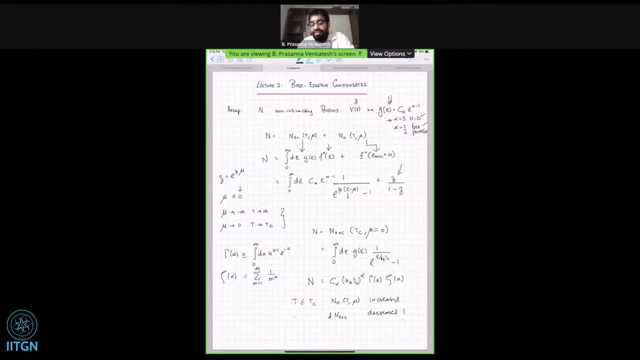 letters of mu. they are in the uniltywhoether when mueth byty is the poquito which determines the plane versus, or the very, very negative, and large is just zero. So there are no particle occupation in the ground state. But as you keep going to lower and lower temperature, 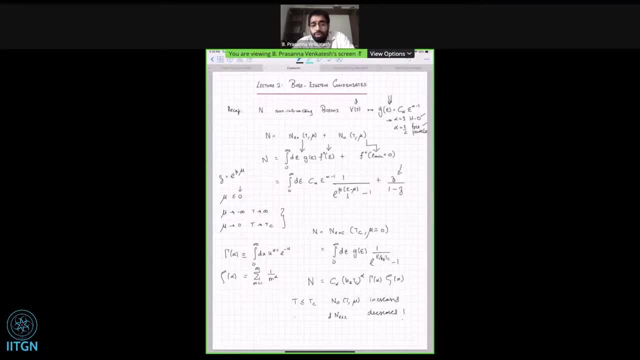 something interesting happens, as we saw yesterday, Beyond a temperature Tc, at which point mu goes to its maximum possible value of zero, you are not able to accommodate all the particles in the excited state. OK, so now you can find this interesting temperature Tc by setting the total number of particles. 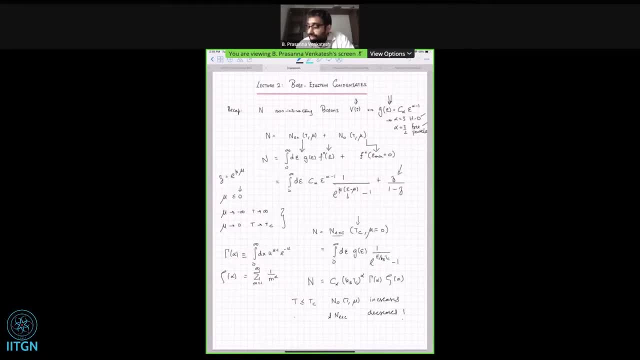 as basically putting all the particles into the excited state, taking mu equal to zero, All right, And below this temperature scale of Tc. what happens is you cannot maintain the particles in the excited state and the particles start occupying the ground state And this happens suddenly at this temperature Tc. 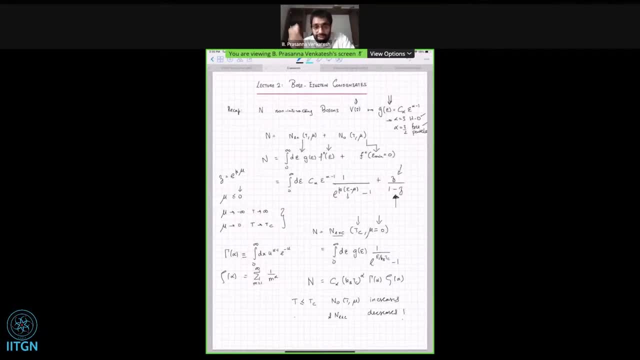 And essentially after a little bit lower. once you get a little bit lower than Tc, there is a macroscopic fraction, N0, of the order of N of particles occupying basically the ground state. Basically, as Z gets closer and closer to one, this number becomes essentially very, very large. 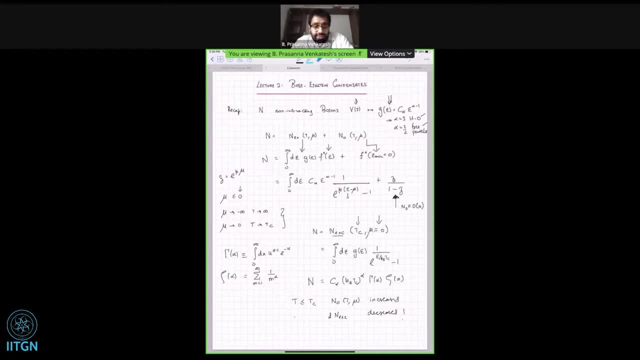 And that is the Bose-Einstein condensate. OK, that is the idea of Bose-Einstein condensation. And now, mathematically, we can write this expression for the N, excited at Tc and mu equal to zero in terms of this integral. 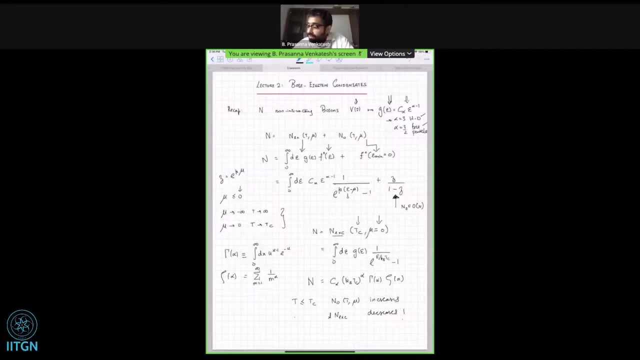 And taking this form for the density of states, we can do a simplification and write the N as C, alpha, KB, Tc to the alpha, gamma of alpha times Zeta of alpha. So gamma of alpha is just the well-known gamma function, which is a generalization of the factorial to continuous variables. 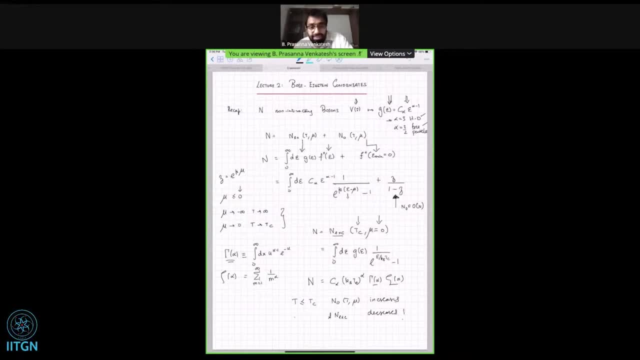 And Zeta. is this even more famous Riemann Zeta? It is a function whose values are known and tabulated and you can use them. It's actually something I didn't remark yesterday. It's quite cool that Riemann Zeta function. 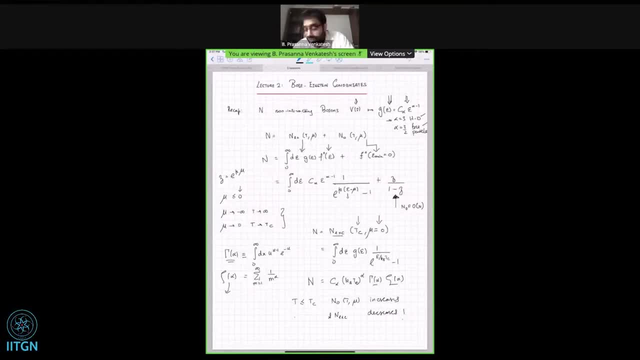 which is a very, very important function in mathematics, in number theory and so on. it has deep connections to the distribution of primes. Somehow nature seems to know about it, at least in terms of Bose-Einstein condensates. There is this very interesting line of research about distribution of primes and statistical mechanics. 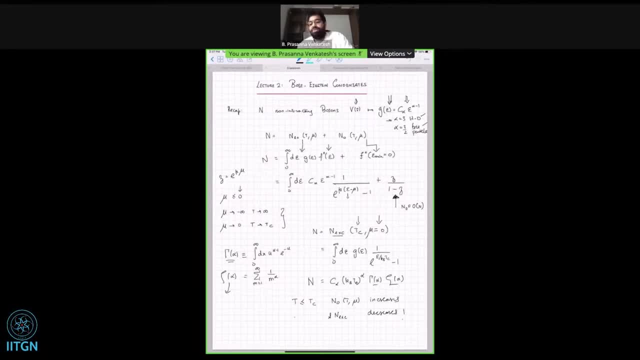 We can talk offline if you're interested in that. I can point to some references later. OK, so now. the idea then is what happens when T becomes less than Tc, This N0, as I said, this thing keeps increasing and basically, this quantity keeps decreasing. 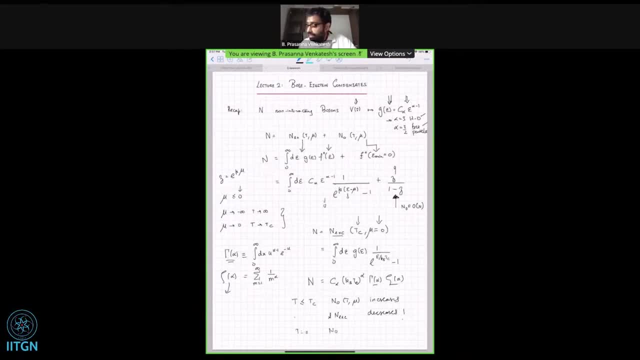 Eventually at T equal to zero. in this non-interacting case, you basically have all of your atoms in the ground state. OK, so basically the entire cloud goes into the ground state and you basically have all the atoms in the ground state or whatever potential you have. 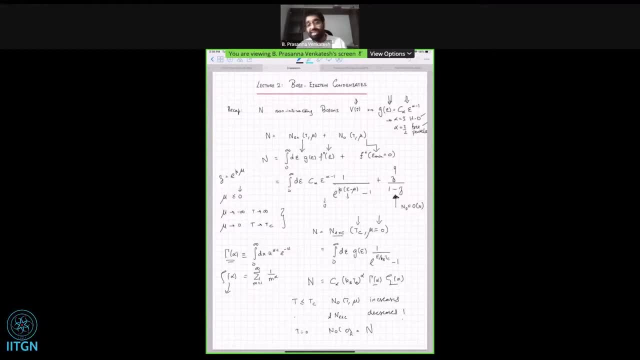 If you have no potential, it will just be in the momentum zero state. If you have a harmonic oscillator, it will go into the Gaussian ground state of the harmonic oscillator. OK, so that is the idea. Inverting this expression very nicely, one can get what is Tc for, basically a Bose-Einstein condensation. 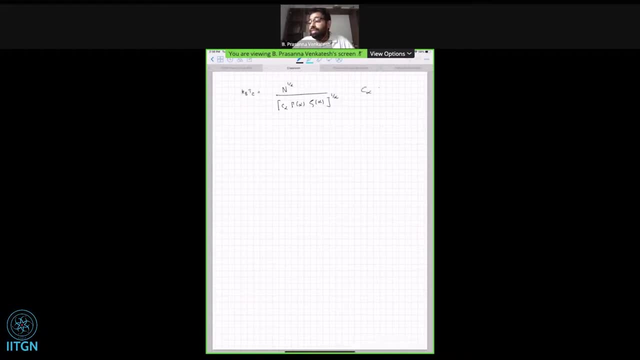 In some arbitrary potential that we have taken. all that we need is C alpha e to the alpha, minus one g of e. One other small detail that we needed was that this integral by itself does not converge if alpha is less than one. 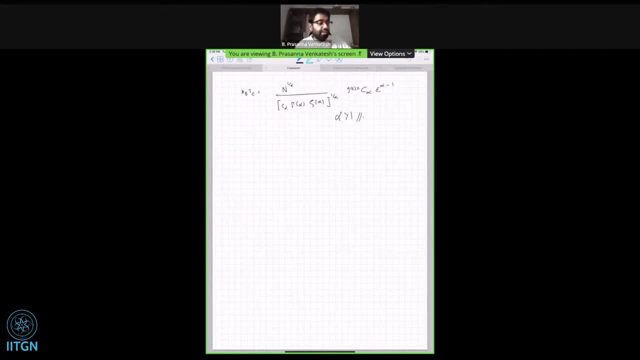 So we are also assuming alpha is greater than one. OK, so that's the idea that we have Before we proceed further. one thing that we want to I want to do is I want to actually now understand how does the fraction- I told you that- at T- equal to zero? 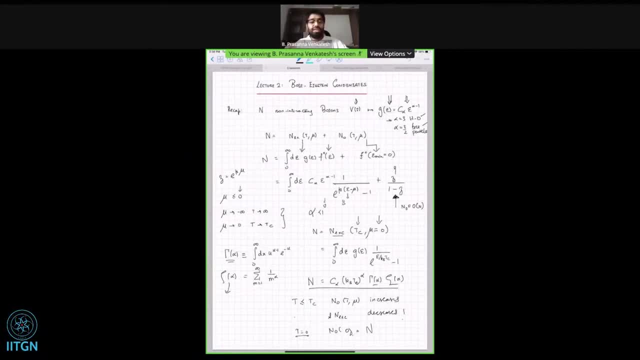 I get all of this, All the atoms in the ground state, But I want to see how, as you lower below Tc, how does the distribution between the excited state and the ground state evolve? Like how many? what is the form of that? 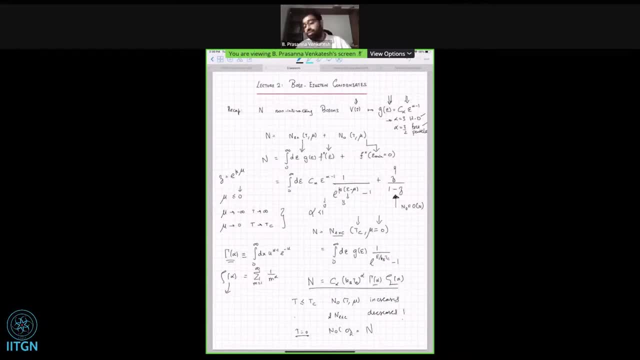 It turns out that that really just depends on g of e, And so it's very easy to derive it. We'll derive it in a moment, But before we do that, let's just plug in some numbers and see what exactly are these Tc? how big is Tc? 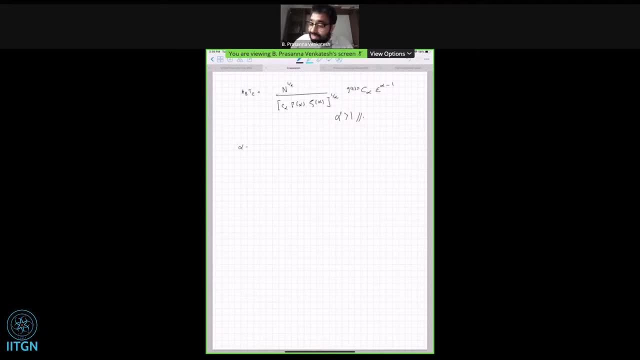 How is it going to be So? for that, let's take one of our examples, Which is alpha, equal to three, and this harmonic oscillator potential. You remember this? C3 in the g of e, equal to C3 e squared, The C3 is one over two times h bar, omega bar, whole cube, where this omega bar is just the geometric mean of the three frequencies. 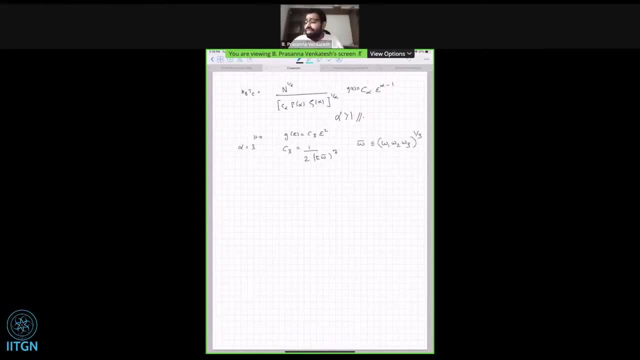 Right, so these three frequencies in principle can be different, but the Tc only depends on the geometric mean of them. Then when you plug that Here, what happens You get KBTC is precisely h, bar, omega, bar n to the one by three, zeta of three, whole raised to the one by three. 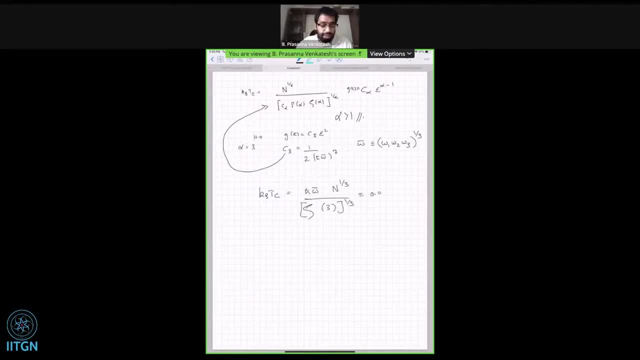 So after a little bit of algebra this is just 0.94 n to the one by three, h bar, omega bar. OK, so now one can write this also in terms of typical numbers that we have right, So a typical Trap that we make. 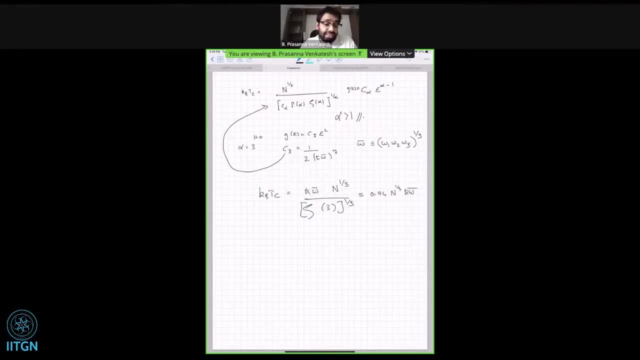 I'll talk about it a little bit later. Traps we make with magnetic fields or using lasers in these traps. The typical trap frequencies are of the order of hundreds of Hertz And with that in mind we can also write this Tc bringing KB to the other side as some number of the order of one times the frequency in units. 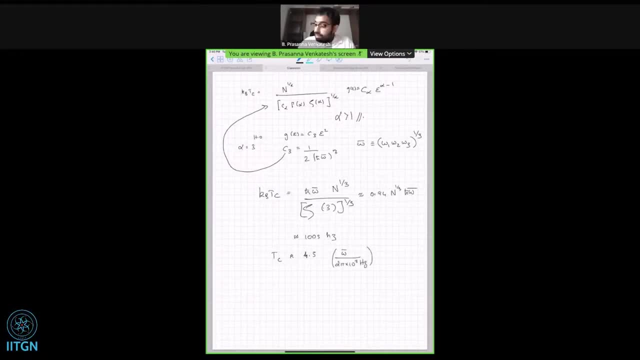 Of two pi times ten to the three Hertz Times n The number of particles to one third times in, And this is written in nanokelvins. This many nanokelvins gives you the Tc. So this is why, if you take, for example, a trap precisely of one kilohertz like, or point one kilohertz, let's say: 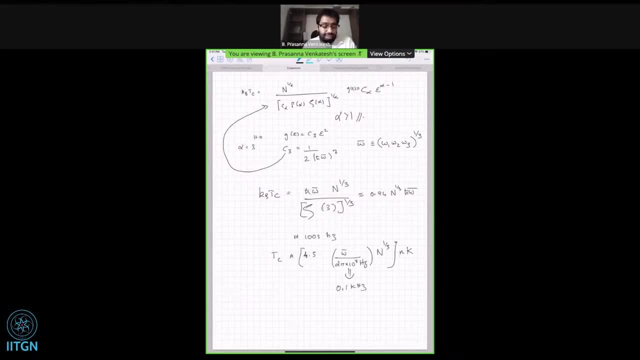 Then you can actually show very simply. if you just plug in these numbers, this Tc comes to about Four point five into ten squared nanokelvins. OK, so for a gas Of atoms, If you are taking this gas of atoms that are non interacting particles and you trap them in basically, 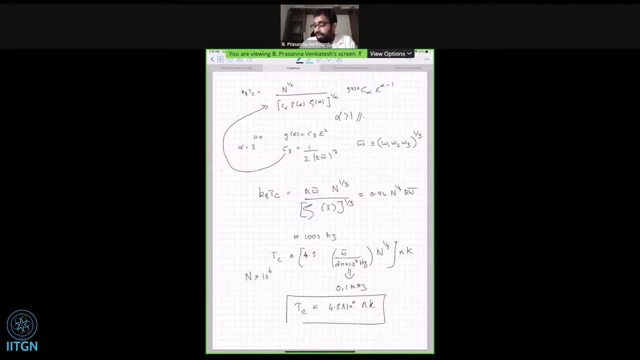 Sorry, and I also should say n, So let's say n of million atoms. OK, so if you take a million particles, bosonic particles, point particles that are not interacting with each other, and you put them into such a trap of hundreds of Hertz, if you somehow manage to cook up this trap at a temperature below hundreds of nanokelvins, you should see a. 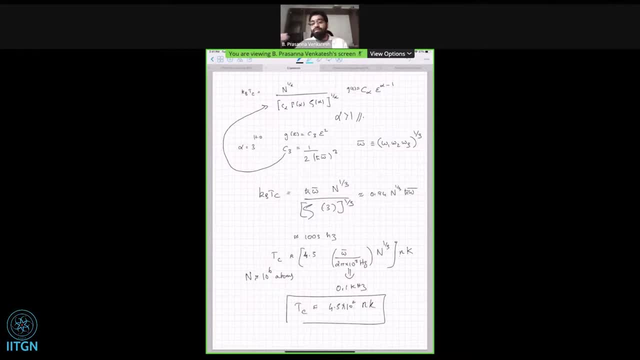 So that's what we are learning from this calculation. OK, so now let's proceed and study a little bit the properties of this condensate. One of the things, as I said, I want to talk about is: what is the distribution? 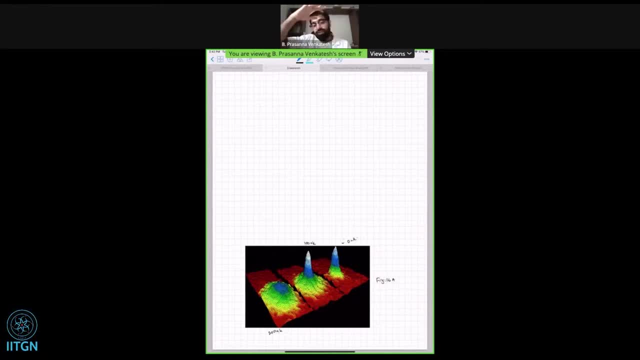 How many of these atoms, once we see both Einstein condensation sets in, how many atoms are in the condensate? How many atoms are still in the excited states? Let's, let's find that out, to find that. it's very simple. We can. 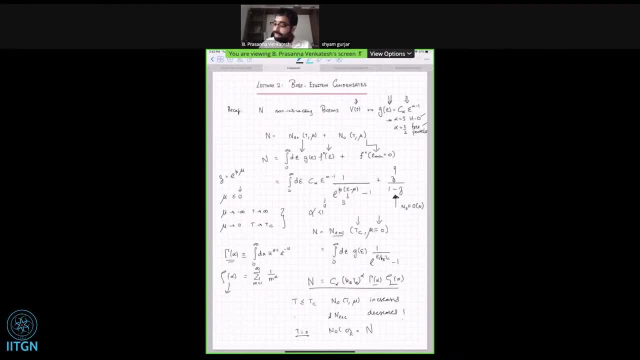 Go back to our expression For this and excited right, and then take mu equal to zero right and actually just evaluated that evaluation is very simple. except it is already here. except instead of DC we will have a T. OK, so we can just write this and excited. 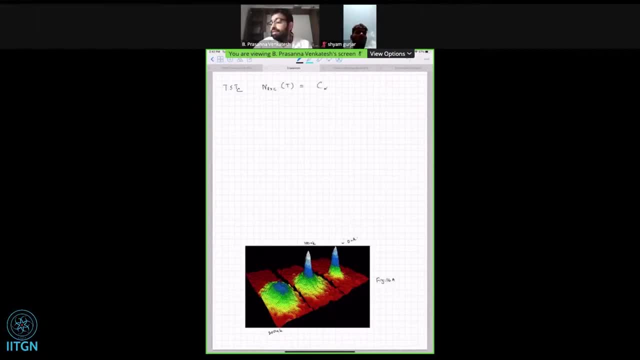 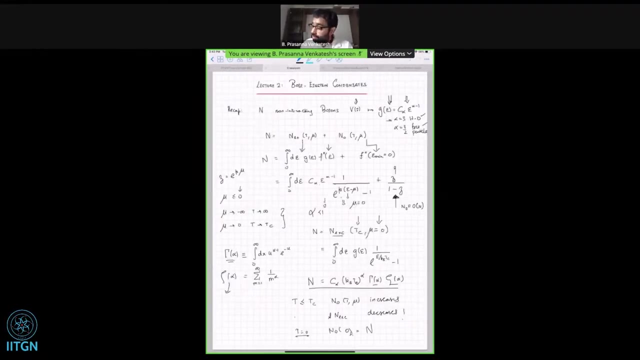 At some temperature T below TC, as C alpha gamma of alpha Zeta, of alpha KBP raised to the alpha. OK, now this is useful, but we can make this into a very nice form by using this expression we have for KBTC to the power alpha, because this constants, which are system dependent, are not really important and we can simply write: 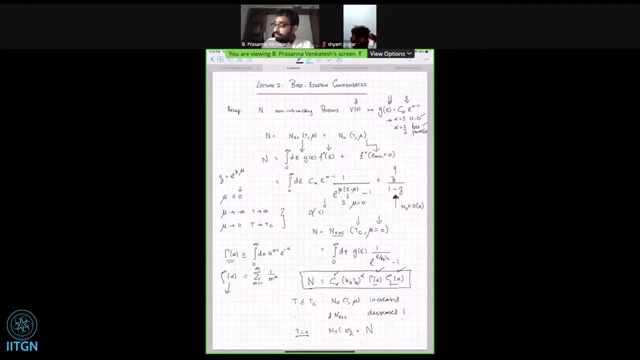 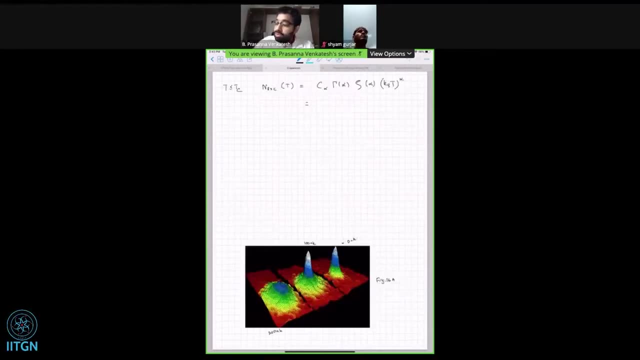 KBTC to the alpha. we can write this: C alpha, gamma of alpha, Zeta of alpha, as just N over KBTC to the power alpha. So then we can do that And we end up with a very nice expression That tells us about the excited fraction. 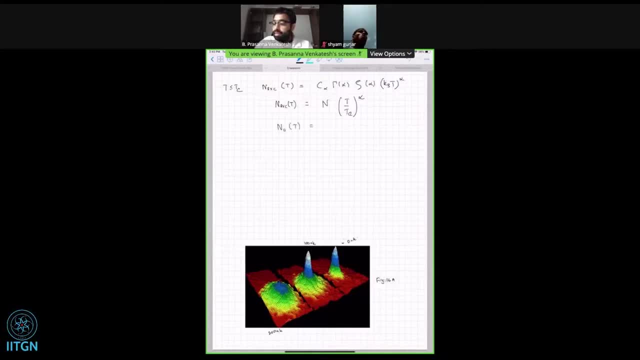 And similarly it tells us that in zero the condensate fraction is N minus N, excited of T, and that goes as one minus T over TC to the alpha, So which is very beautiful. So this number of atoms in the condensate, 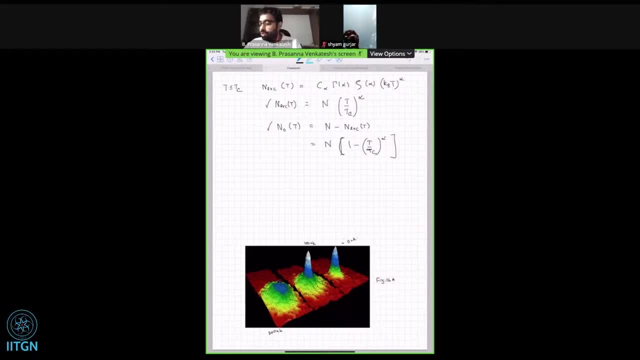 Precisely. It becomes a very neat universal function that just is decided by how your density of states goes as a function of energy, OK, and it does not depend on other details once you have a condensate. OK, so that's very useful. 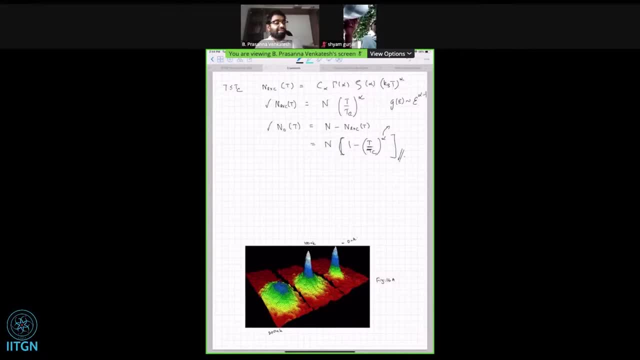 And one of the things that we want to talk about next is: how exactly do we know that we have a condensate? How do you, for example, we have a few predictions here. We said all of the atoms go into the ground state and this number of particles in the ground state has some marked behavior as a function of temperature. 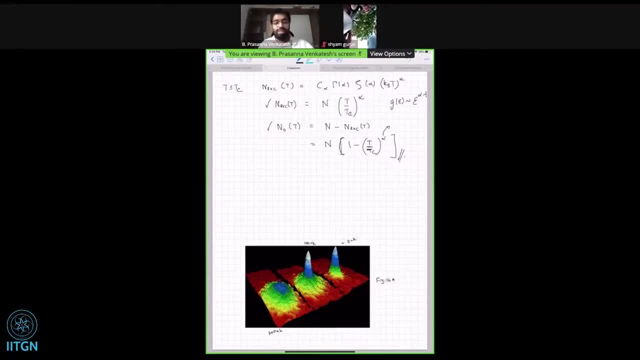 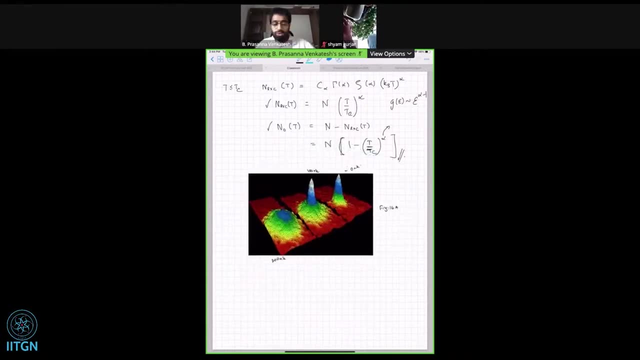 Can we verify this? How did people verify this in the experiments? Because I claimed in the beginning that they made an experiment, and this is sort of the most iconic figure that was produced from one of these experiments, which shows the density distribution of a Bose-Einstein condensate as a function of temperature as it undergoes Bose-Einstein condensation. 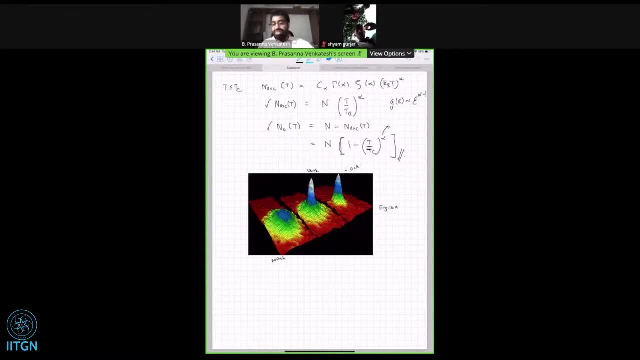 How do we read this figure? What are we seeing in this figure? So let me just describe. how do you image an ultracold atomic gas? Basically, this gas- even here it's at about temperatures of 200 nanoKelvin, and then it just crosses into the BC, here in the second picture. 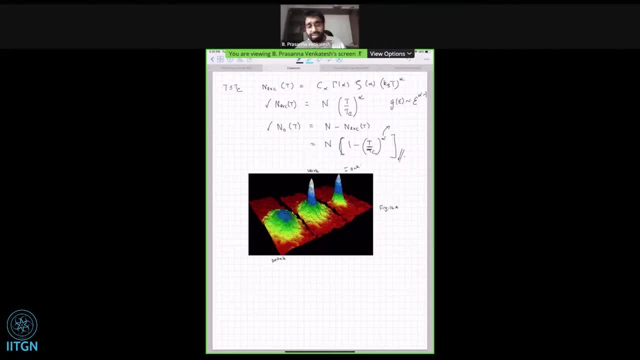 And then this is almost as good as being at zero temperature right. At these temperatures you cannot use, basically in these systems, and at these temperatures you cannot use very cold temperatures. So there is this thing called the. So I've not taken care of interactions at all in my theoretical discussion. 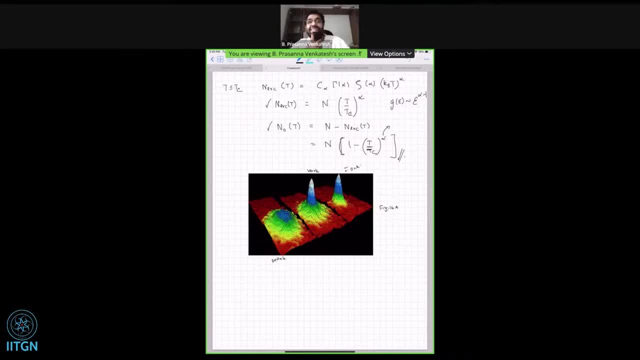 in my theoretical description yet, but they are, in a sense, interacting atoms and they, as a result, the these bosons and condensates that people produce. they are metastable states, so they have some lifetime. so you create a bc. it will be inside this trap for a very long time, but still finite. 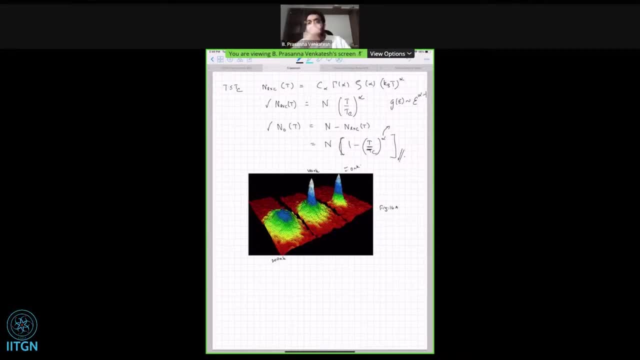 amount of time. so you have to find probes that work on the time scales. that is convenient for the atoms, okay. so one obvious probe for such things is laser light, okay, so in order to understand basically how laser light is used to take such pictures, one has to first understand. 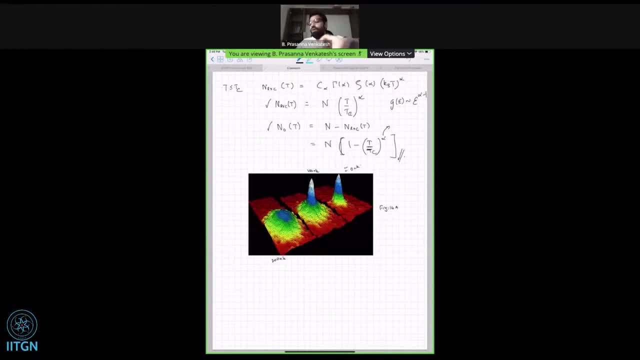 that i have been talking about bosons as point particles. right, all of this ideal gas particles. i've been talking of them as point particles. now, the idea there is that this is not true if you have a, an actual atom. in principle, actual atoms have, uh, basically rich internal levels. 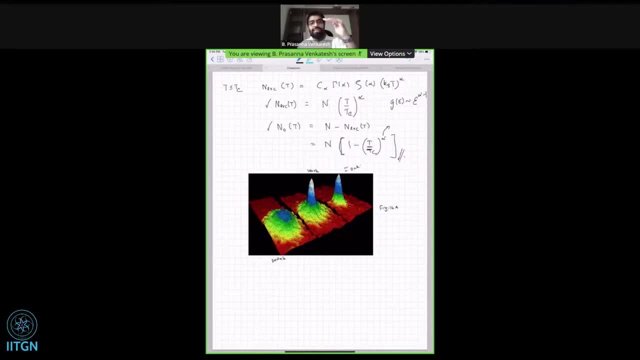 structure and, more importantly, typically one can find resonances with some sharp optical transition in these atoms. so there will be some. these are the things that you learn in hydrogen atom, lyman series lines and optical transition. so these optical transitions then you can actually address by shining a laser. so in order to take a picture of such a such a distribution, 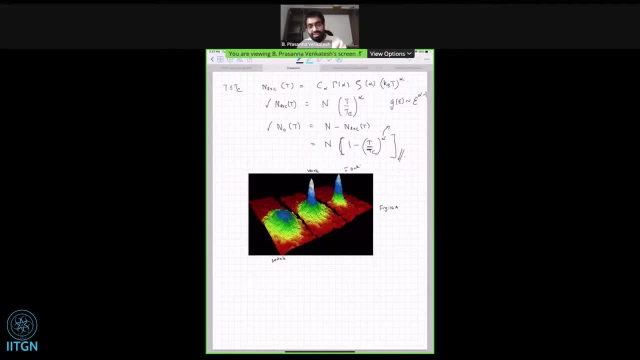 of atoms. all that one does, then, is one shines a laser resonant with one of these optical transition and, as a result, the atoms absorb this light and they make a shadow, and this shadow is basically then imaged onto some ccd camera, and this is precisely what is. 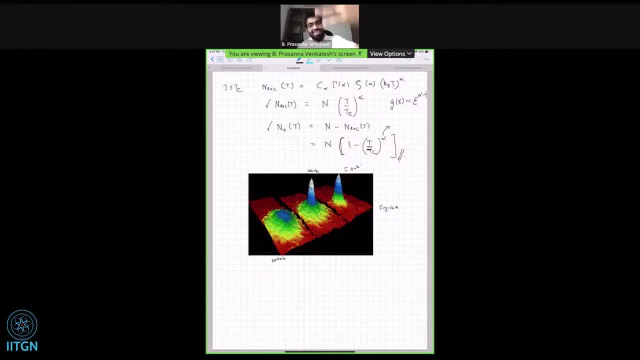 called absorption imaging, and with this you can essentially get a two-dimensional picture of the density distribution, and that is what is being plotted here. so this is basically this: uh, the, the plots, these contour plots. this third dimension is density, and this is x and y direction. it is integrated over the direction in which the laser is being 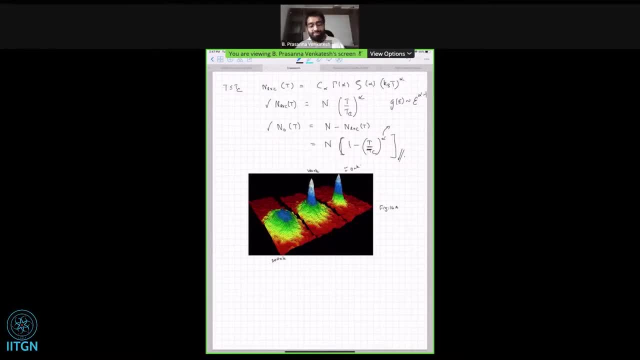 applied, but otherwise it's a two-dimensional picture of the density. okay, so now the idea is that that is so. it's basically a picture of the density of this ultra cold gas. but then how do you know that there is- essentially you have- a boson stand condensate. so, in order to understand that, 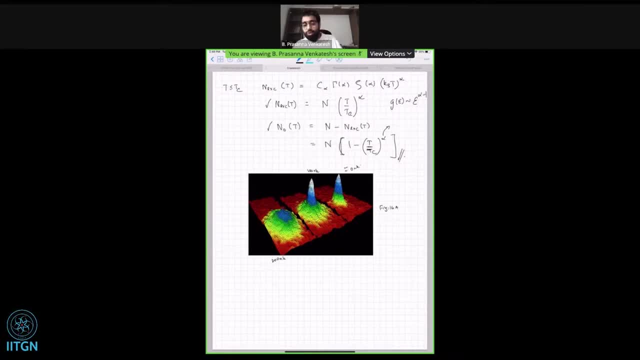 there is one other subtlety that one has to understand about how such pictures are taken with cosine stand condensate. the first subtlety is that i told you that these atoms have these. you need the trap. all of our discussion was in a harmonic trap, right? so once you have made a harmonic trap and somehow, 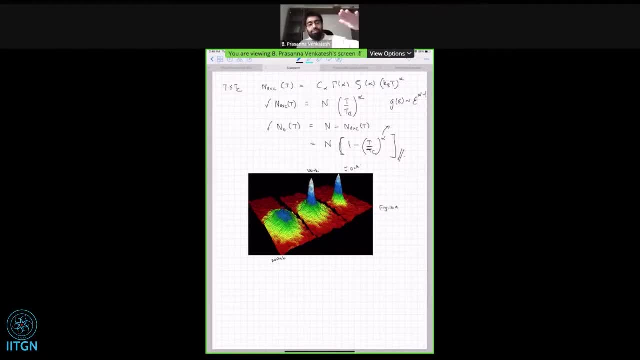 cooled the atoms below the transition temperature. what one does before taking a picture is one turns off these traps. okay, once you turn off the traps, the atoms, the cloud starts expanding because there is no potential. it's just going to expand. for example, think of a gaussian in p squared by 2m. 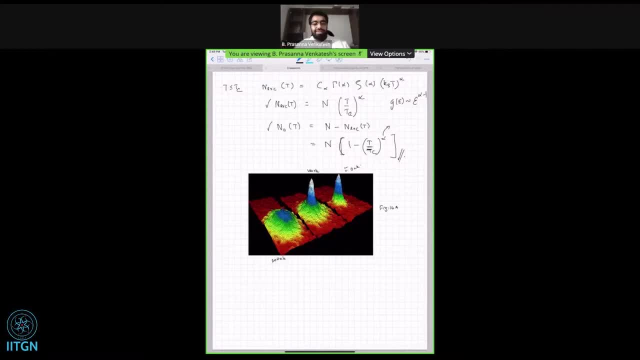 potential. it's square by 2M Hamiltonian. it's just going to expand. So this is pre-expansion of a cloud. But interestingly enough, if you look at the position at some later time, the position distribution, this is density in position space. 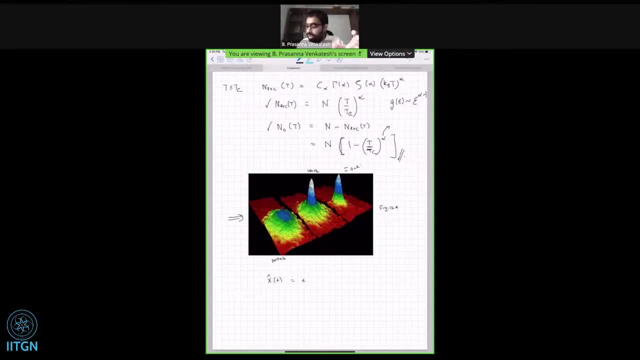 When you look at the position space distribution after you turn, you basically turn off the traps at some time 0, and you then take a picture at some time t after basically a time of expansion tf. Then what happens is basically the position distribution. 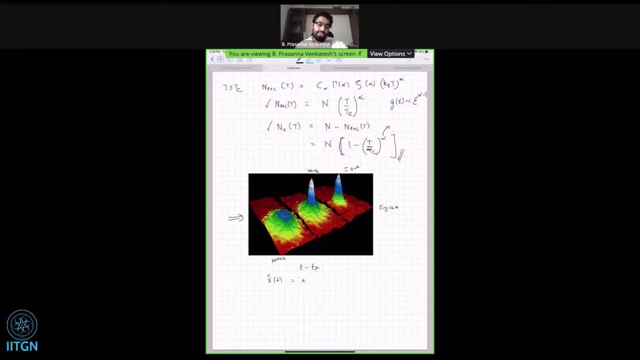 at this later time actually reflects the momentum distribution at an earlier time. So this is really a very simple consequence of Newton's laws. So if I just write the position evolution, position evolution, Operator evolution at some time, t, it is the position distribution at t minus tf. 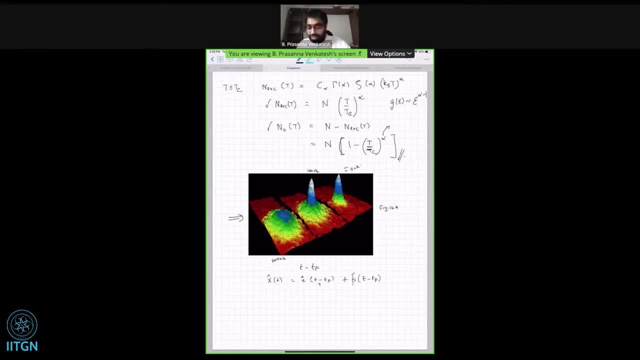 plus the momentum distribution at t minus tf, tf over n. So having a density distribution is just having a density distribution at this time t. So the position space density distribution at time t is precisely related to the momentum distribution at some time t minus tf. 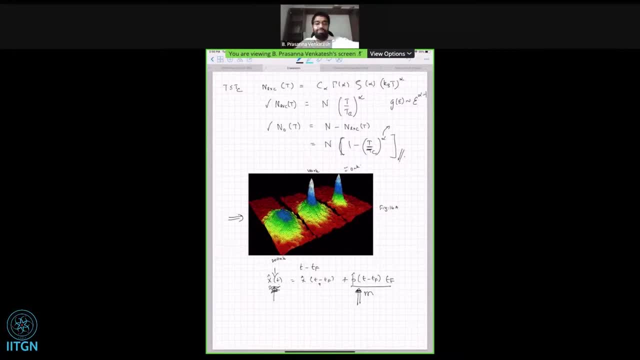 And this tf is called the type of flight where the atoms have expanded, And this kind of absorption imaging is called time of flight absorption imaging And this is what has been used to make these pictures. And these pictures precisely reflect the momentum density distribution of a gas of atoms. 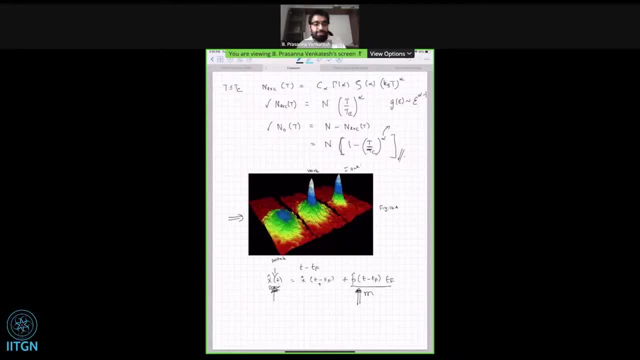 as it undergoes a Bose-Einstein condensate phase transition. That is the idea. With that in mind, now let us look at how to read this picture. Because this iconic picture, at least if you get nothing out of these series of lectures, since this picture is always. 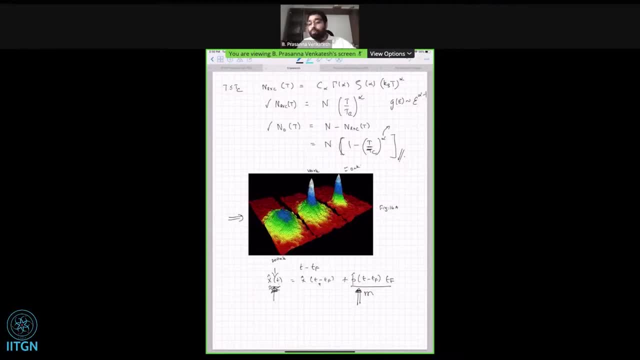 displayed when people talk about Bose-Einstein condensates. I hope you will at least leave with a better appreciation of what sort of physics this picture is telling you. So with that, let's now look at. what should we expect for the momentum distribution. 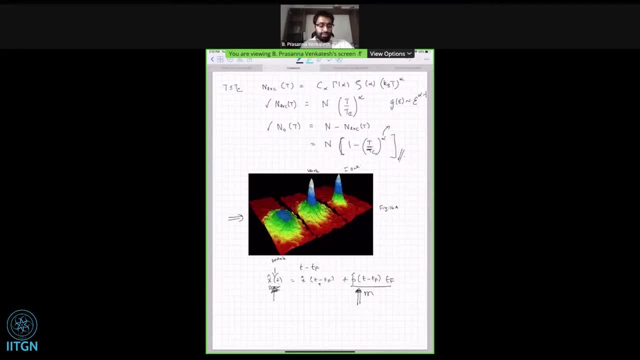 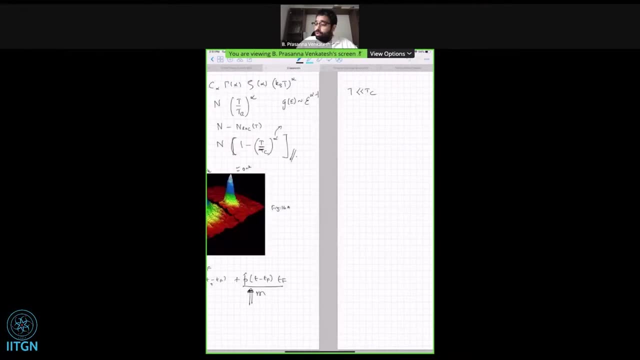 as we undergo a phase transition into a Bose-Einstein condensate. You see that it's very simple When you are at temperatures much below Tc. so when you are somewhere here, then of course all of my atoms, n atoms, all of them, my condensate fraction. 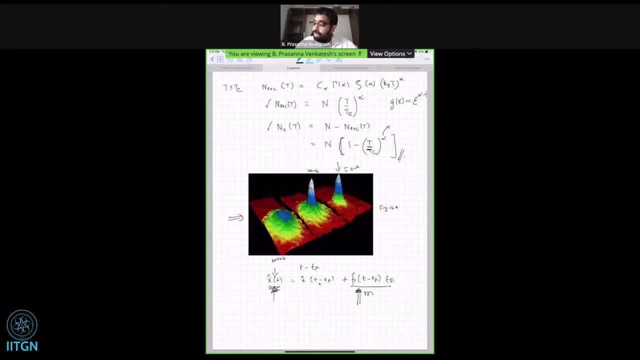 basically becomes from this equation here: if I make, p goes to 0,, n0 becomes n, So n0 equal to n when temperature is close to 0. And in this limit I said basically that all of my atoms are going to be. 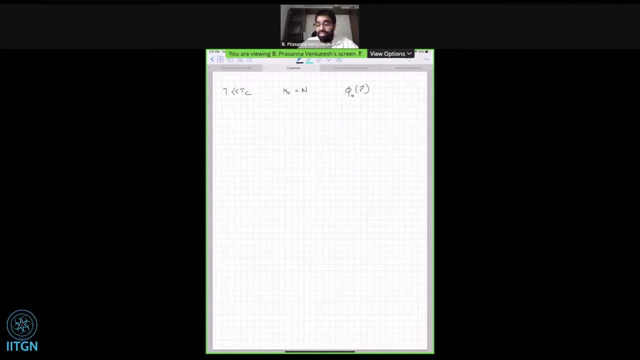 in the ground state of my harmonic oscillator potential. Let me call phi0 for the ground state wave function of a three-dimensional harmonic oscillator. Then my atomic density distribution is nothing but n times phi0 of r whole squared. So once I plug that in, I basically 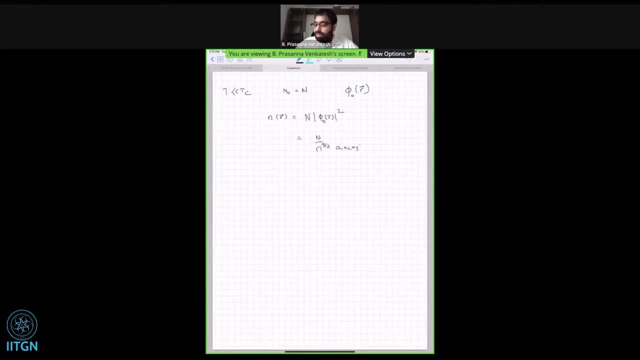 get this simple expression: phi squared by a2 squared, z squared by a3 squared. And these ai's are precisely the harmonic oscillator lengths in the different directions. So the first observation you make is that this density distribution is not isotropic in space. So it depends. It has a different length in each direction. If your trap is very tight, your distribution length becomes larger, So sorry, your distribution becomes smaller. So if you have a very weak trap, your ground state extent is larger. basically, 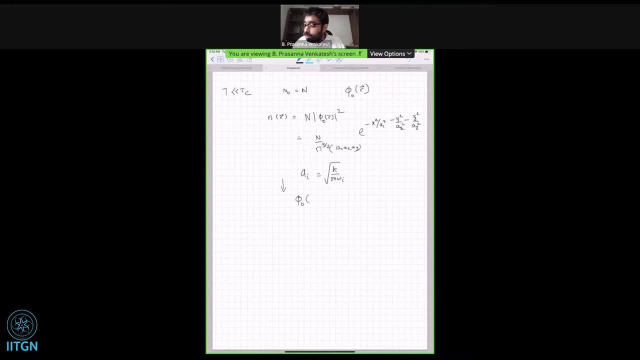 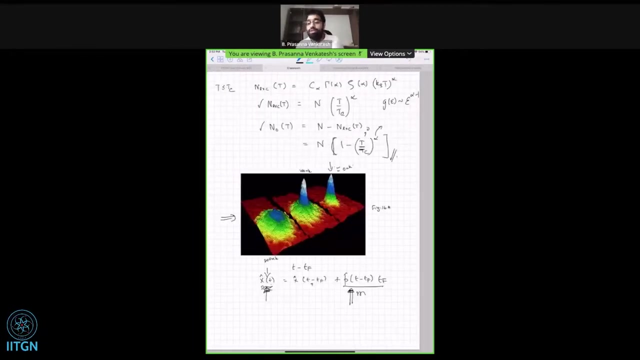 With that we can basically then use the momentum space wave function That is corresponding to this harmonic oscillator, which is simply a Fourier transform of this Gaussian, and write the momentum space distribution Because, remember, the pictures I said were really momentum space distributions. 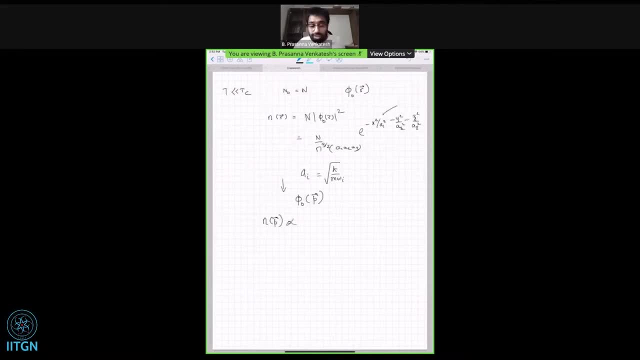 So n of p is precisely proportional again to e, to the minus px squared by c1 squared, minus py squared by c2 squared, minus pz squared by c3 squared. And the ci again are simply h bar over ai, and they are not. 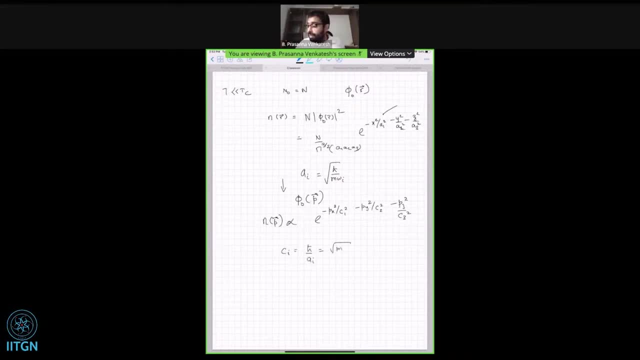 are not equal to each other And they depend on h, bar, omega, i, and they can be different in different directions. So it is an isotropic momentum distribution. Now, that is what you would expect once you have a Bose-Einstein distribution: Bose-Einstein. 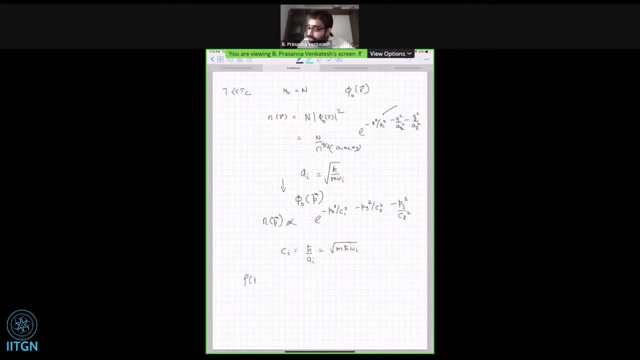 condensate in your trap. But now let's compare it to what happens when you have a thermal distribution of gas. So this is very simple: When you don't have a classical thermal distribution right of a classical gas which is not condensed, 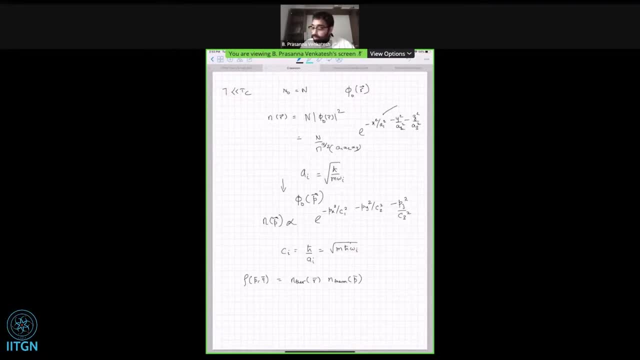 is simply product of r and p distributions in phase space, And this is just by what you know of classical statistical mechanics. This is proportional to e, to the minus beta h of rp. More importantly, the momentum distribution is precisely nothing but the Maxwell-Boltzmann distribution. 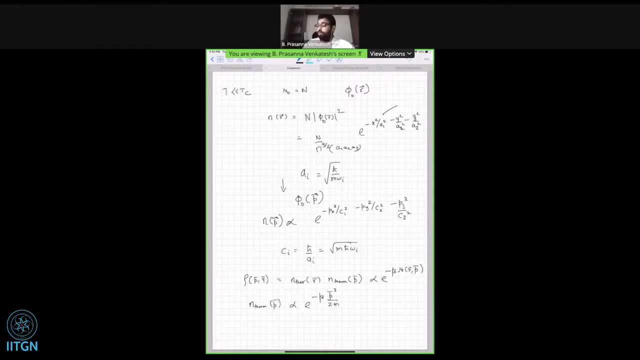 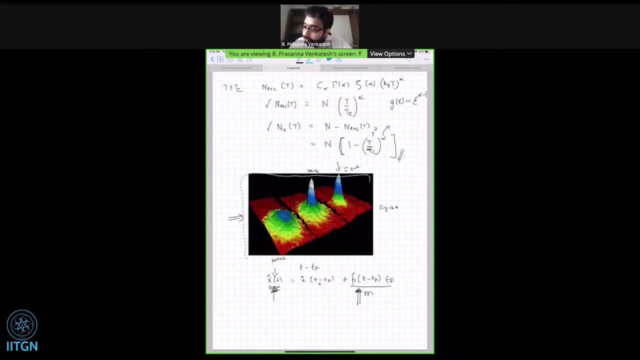 And one very, very, very important aspect of the Maxwell-Boltzmann distribution is it is completely isotropic in px, py, pz. So now we can read this picture very easily. Let me try and see if I can enlarge this a bit. 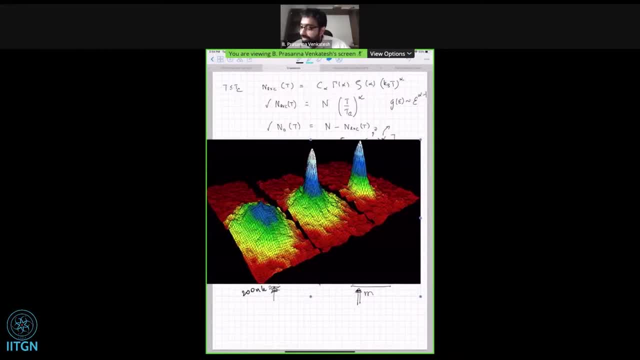 Now, if you can see, what is happening is as your temperature becomes smaller and smaller, at p, at very large p, we simply have an isotropic distribution in these two directions, called an x and y, And this is just a thermal cloud of atoms. 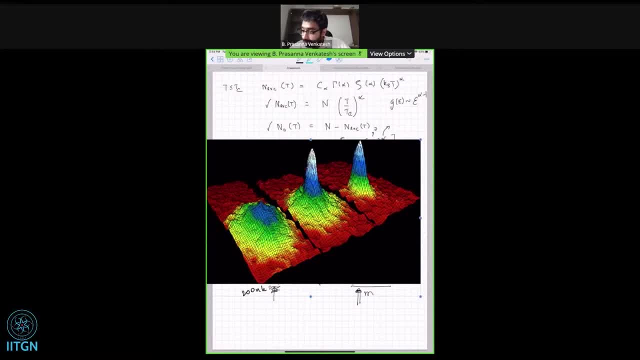 But as you go to lower and lower temperatures, this is a trap that is tighter in this direction, In the let's call this x and let's call this y. In the x direction, this is a tighter trap And you clearly see, once the temperature becomes lower. 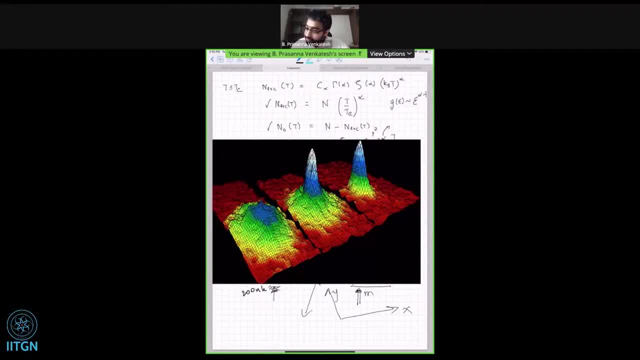 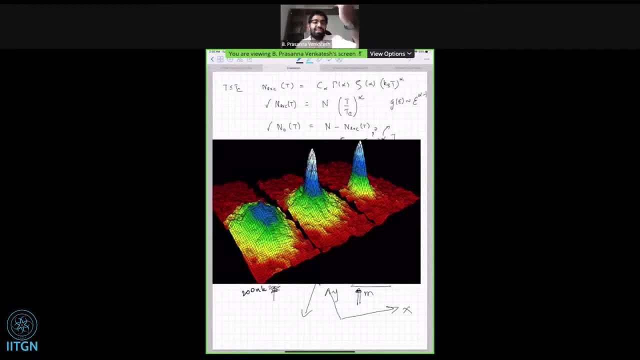 on top of this thermal cloud that is isotropic and an isotropic cloud of atomic density distribution and momentum space arises. So this tells you that we have a Bose Einstein condensate. So this anisotropic momentum distribution was the clearest signature that we 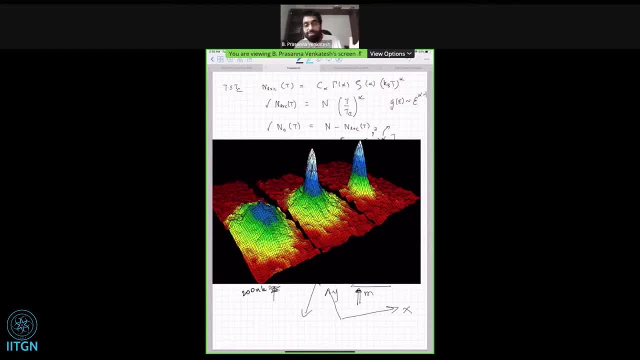 had this Bose Einstein condensate in the lab, And this was after work science, at least according to me, and so this is the clearest signature of it. the second sort of very nice experimental signatures that you can get is you can really, if i look at this absorption. 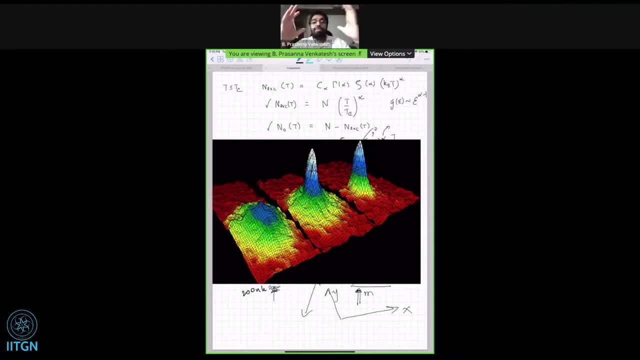 image. this absorption image also counts the number of atoms. if i integrate the shadow over the entire area of my ccd camera, this tells me this is a measure of the number of atoms. and now, since this part is actually uh and i also have position and spatial information, i can really count by taking. 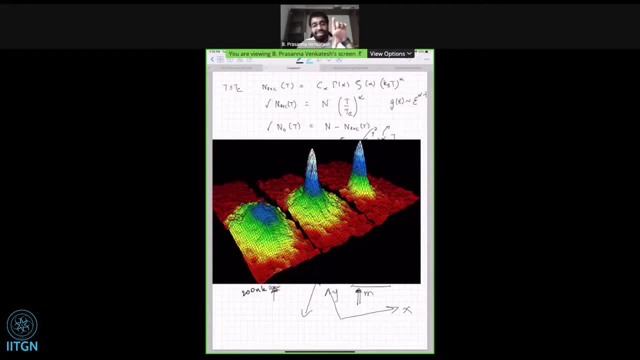 the ratio of the shadow with this anisotropic peak versus this isotropic peak. i can really take the ratio and really from the experiment, compute this fraction of condensed particles as i keep lowering my temperature, as a function of as i keep lowering my temperature, i can count. 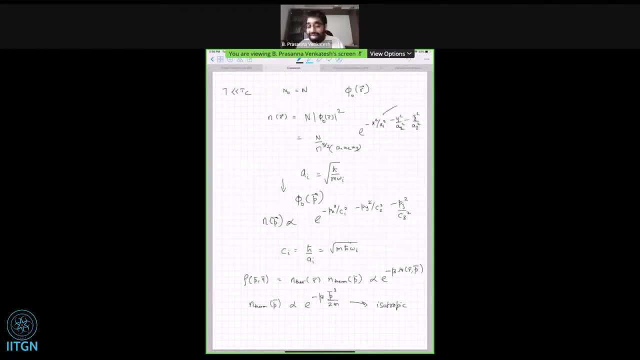 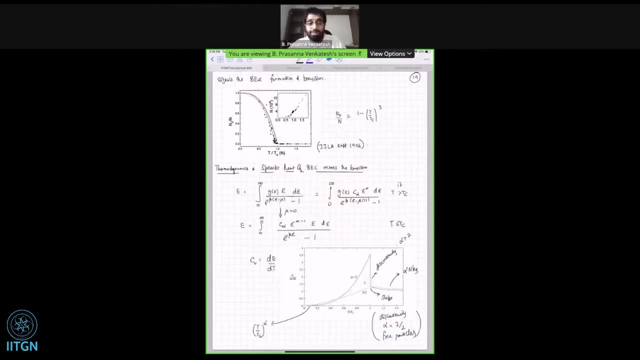 what my n zero is okay, and that was again done in experiment and that is another beautiful signature for the fact that we have a Bose-Einstein condensate. so this is a picture from the same set of experiments from eric corner's lab, who won the nobel prize for this. 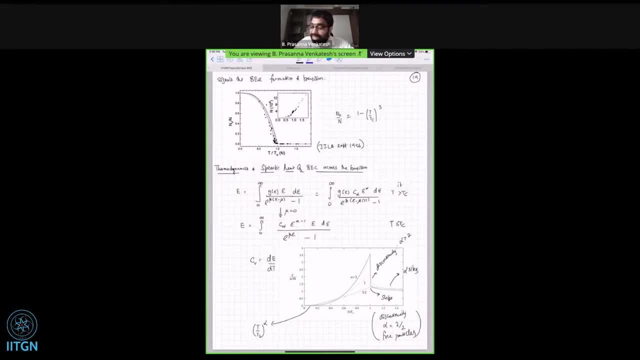 and you can see very beautifully these dots are precisely the experimentally measured fraction of condensate and it really very nicely follows this one minus t over tc cube, which is the solid line. okay, so really there's no doubt that this condensate was achieved in this experimentally very beautifully. okay, so that's. 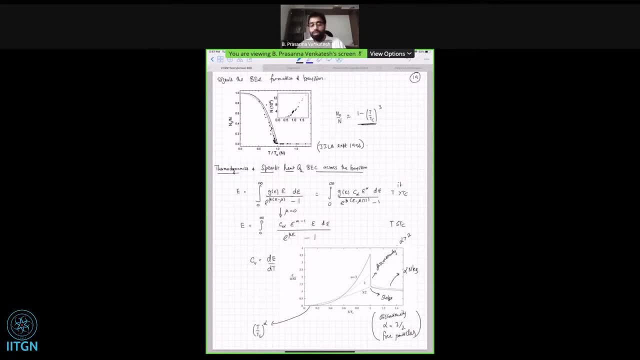 that's a couple of experimental details i want to talk about before i sort of wrap up essentially this way of looking at condensates with non-interacting gas of atoms. i just wanted to mention a couple of things that we discussed yesterday. one is: what is the nature of this phase transition? i won't have a lot of time to go into it. 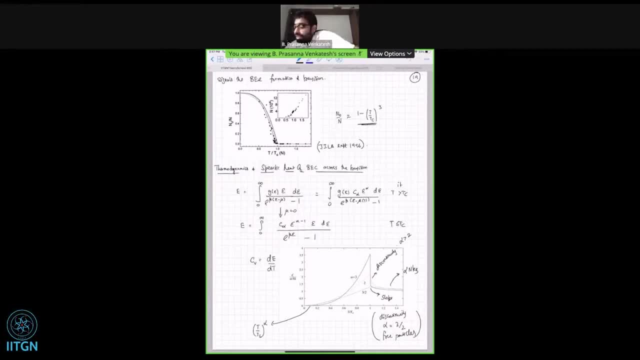 it turns out that the nature of such phase transitions. you can really discern that by looking at how thermodynamic functions, for example. in this case i'm looking at the specific heat, which is the change in energy with respect to temperature. one can write this e again using average energy, using this g of e and the pose function and i. 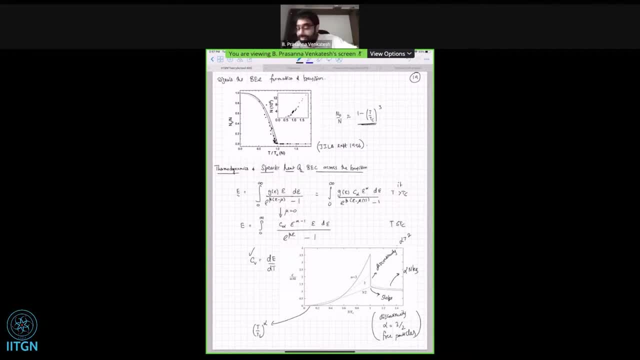 can see. one can actually theoretically calculate it for an ideal gas and one sees that, depending on what sort of alpha you have, depending on what sort of single particle density of states you have, you can either get a slope, discontinuity, for example, in this case, if you have three particles. 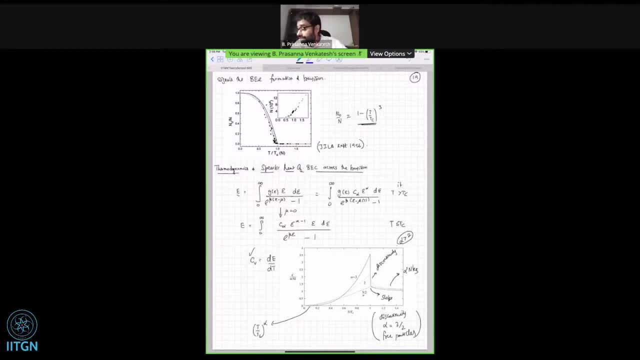 and alpha is three by two, you get a slope discontinuity. if it's actually um, if alpha is greater than two, for example, like a harmonic oscillator, you get an actual discontinuity in the cv. so as a result, since the response functions and hence whatever free energy that is underlying this, like energy is, has different kind of non-analyticities. 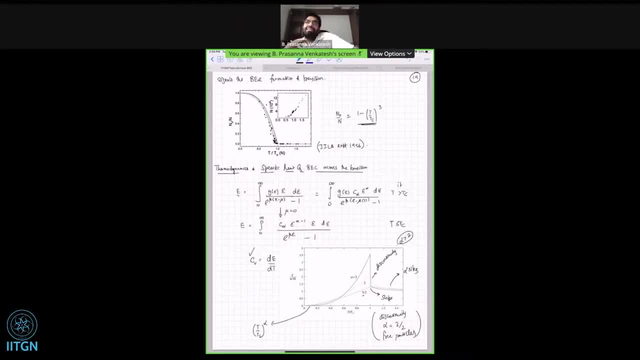 depending on g of e. one cannot very simply characterize a Bose-Einstein condensate transition as a first or second order, and it has aspects of both first and second order. but the very fact that thermodynamic functions are discontinuous right, or that they have some non-analyticity, tells us that 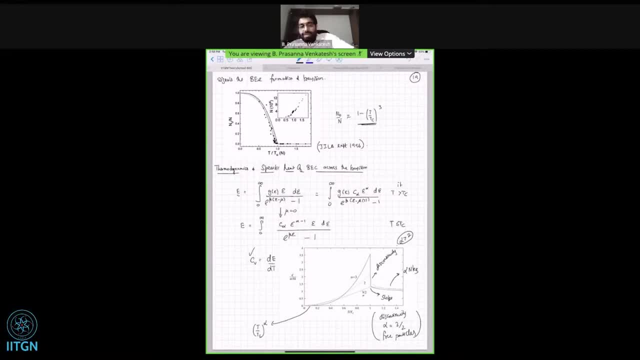 this is a bona fide phase transition, thermal phase transition that we are seeing okay. so that's one small thing i would like to point out, and then i would like to move on to the next slide, please. I wanted to talk about in terms of what is the thermodynamics of this BEC transition. now one last. 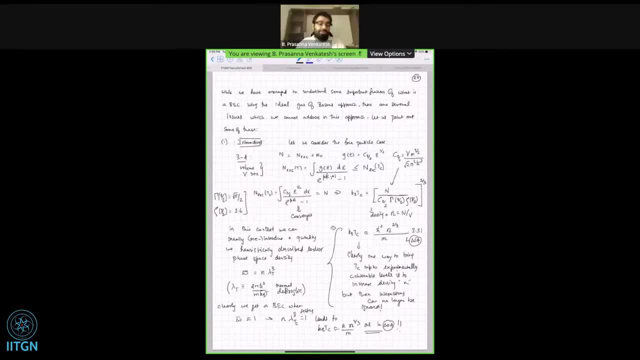 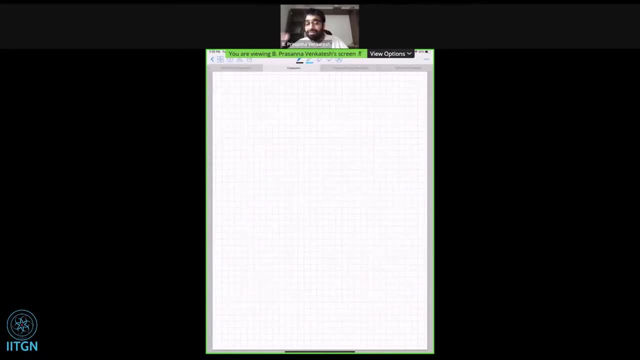 thing which is going to be the motivation for the second part of today's lecture is: okay, we talked about ideal gases and we really have talked about ideal gases and we have understood in one manner what is a Bose-Einstein condensate. but now i want to actually talk about Bose-Einstein condensate. 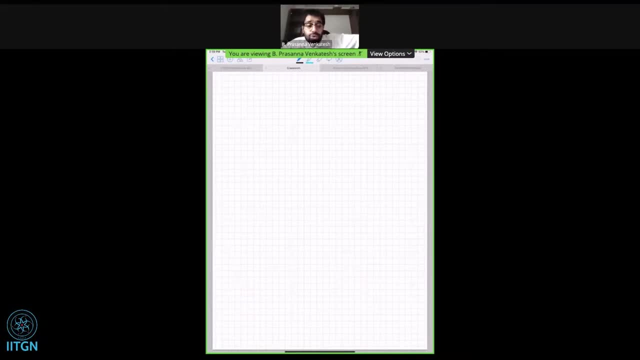 in a more sophisticated and general manner, and the reason i want to do it is because this ideal gas picture of Bose condensation is not enough. it has some deficiencies. one very simple deficiency, basically, is we cannot- there are no interactions included in this picture but any real physical 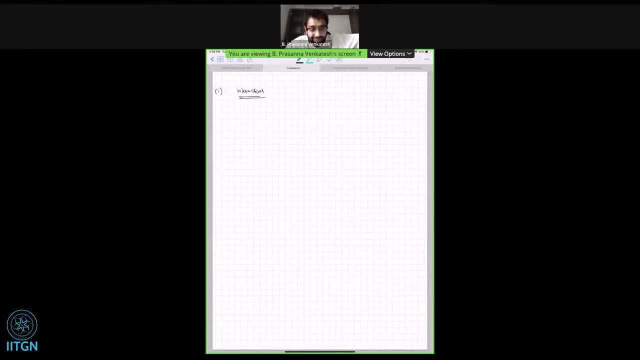 system that we have, we make with gases, they will have interactions, okay. so, for example, we have already faced this problem about the Bose-Einstein condensate transition and interactions a little bit earlier, right? so for example, if we take this free particle limit and take alpha equal to three by two and g of e is basically c three by two, e to the half, with. 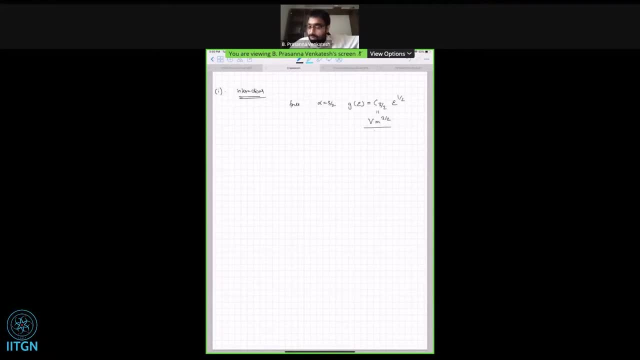 c, three by two, given by bm, to the three by two by h, bar cube. if we take this kind of form, we can actually work out, exactly using the same expression that we have for kVpc, the temperature transition temperature for a uniform gas of particles. for a uniform gas of particles, we get this transition. 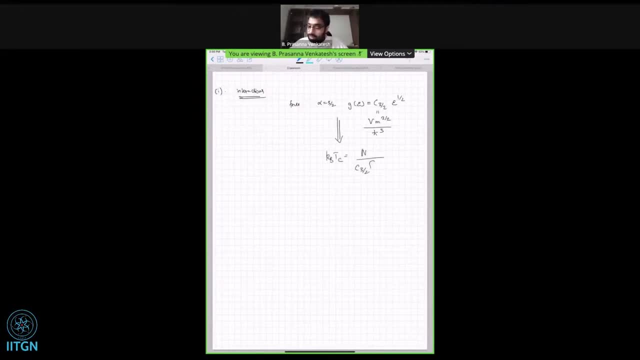 temperature and this transition temperature for a uniform gas of particles. we get this transition temperature, temperature n, c three by two, gamma of three by two, zeta of three by two, and, very nicely, if you plug in the constants for this, you really get h bar squared n to the two by. 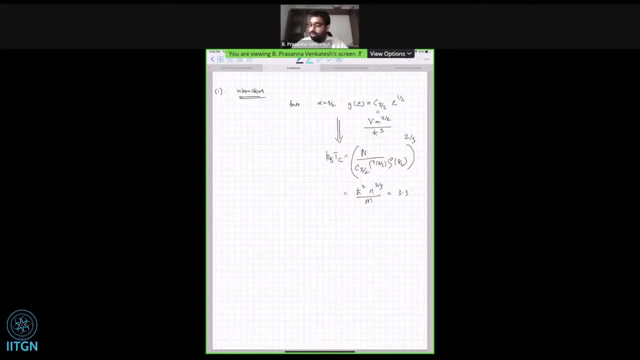 three over m times some constant of the order of one. this is very beautiful because really we got very close to this estimate by simply taking n lambda Tc cube equal to one earlier. okay, so we from from this very cartoonish argument of Bose-Einstein, condensate: And this works very well. 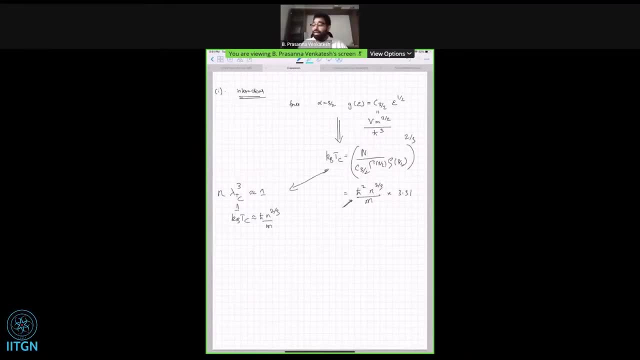 with a more sophisticated calculation of this KBTC. But the problem persists that as I keep making my interaction density- but any finite density- I will have interactions And, as a result, this TC calculation and in general, this whole the way that we've been thinking. 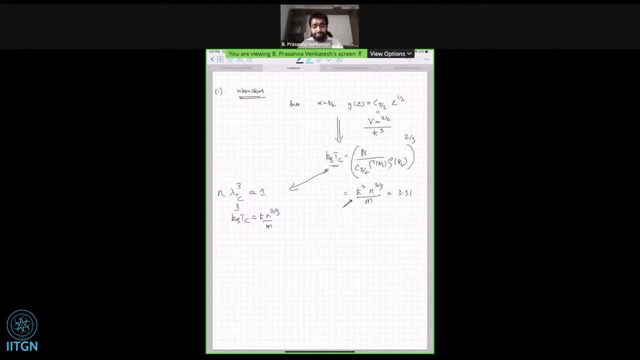 about Bose-Einstein condensate will not work with interacting systems. The second sort of drawback with what we just discussed as basically Bose-Einstein condensate of ideal gases, is that if we go to a lower dimension, so if we take a lower dimensional system, that is not really. 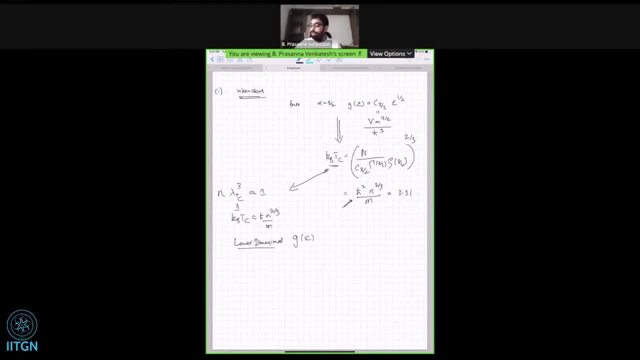 three dimensions and we look at G of E, for example. if you take three particles again, we will see that C, alpha, the density of states, goes as E to the zero, and G of E for even lower dimension. one dimension actually, that is it's. 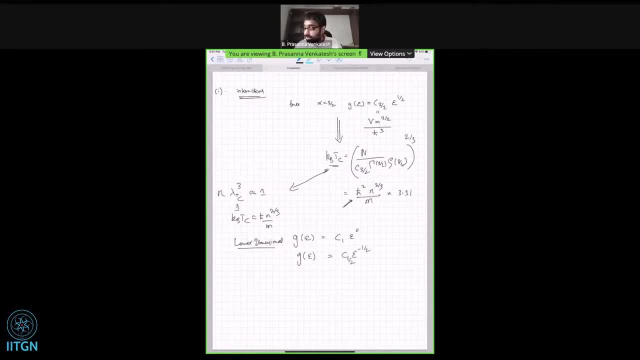 singular and it goes as: E to the minus half, C half, E to the minus half. okay, Now this is a problem because if you look at our excited fraction, this is always less than equal to the excited fraction at TC, which is given by this integral that we've been evaluating for alpha. 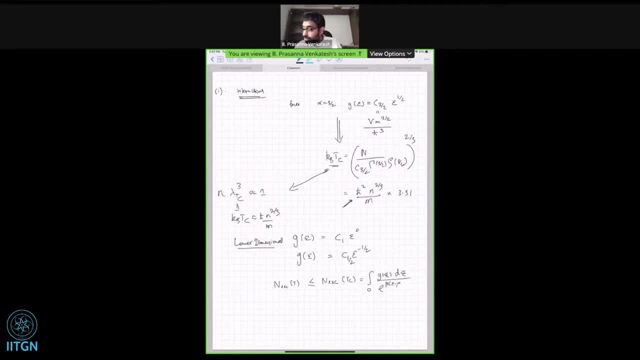 greater than two. right Now, the problem is this integral doesn't converge when here alpha is one, here alpha is zero. right, Alpha minus one is half one plus half, so this is alpha is three by two. So in these cases, if you plug this into this integral, this will diverge, okay, Which means 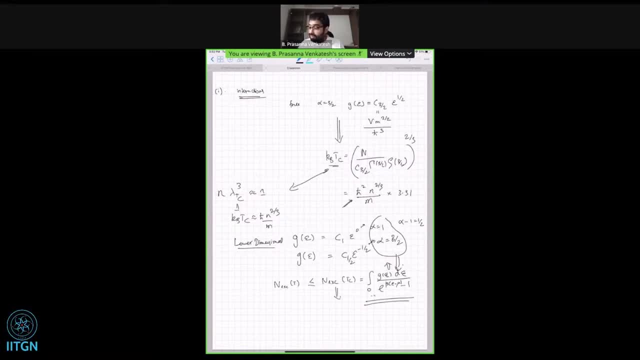 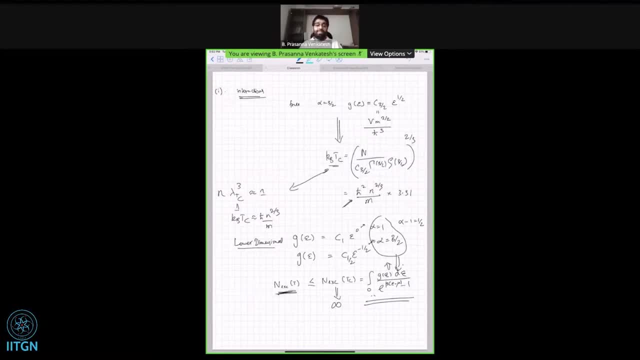 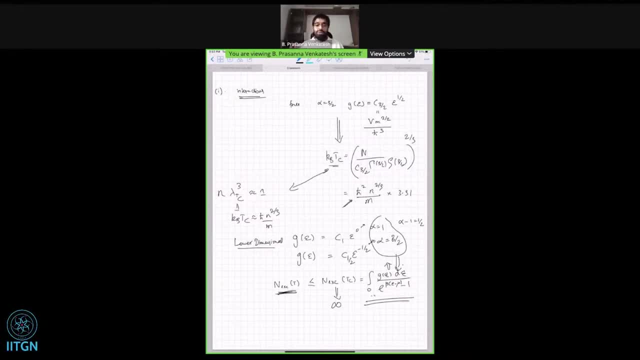 There are some general arguments in statistical mechanics that tell you that you cannot get such a phase transition at finite temperatures for a uniform system when you're in dimension two or lower. okay, And this is a very famous theorem called Mermin-Wagner-Ohenberg theorem. 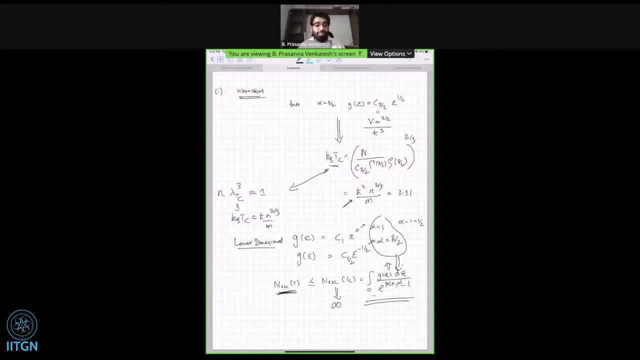 So I'm not going to go into the details, but our model doesn't capture that right. So that is the problem. That is another problem, And there are multiple other reasons that are given. One thing is: we need to study interacting system, because superfluidity, for example, typically only occurs. 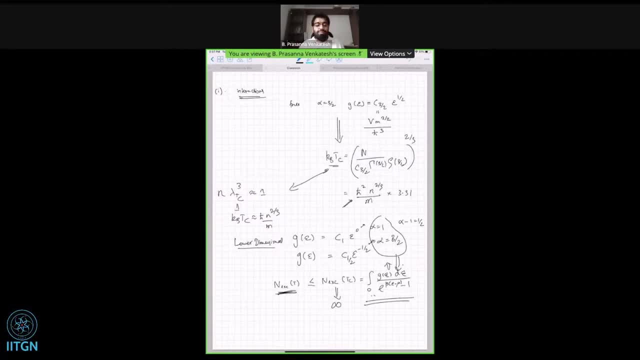 with interacting systems, And so it is very important to extend our idea and notion of Bose-Einstein condensates to interacting systems. That is what we will do next, using this very powerful mechanism or powerful way of treating Bose-Einstein condensate or defining Bose-Einstein. 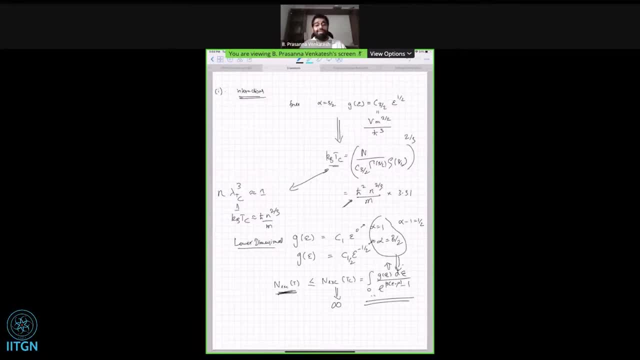 condensate using the idea of off-diagonal long-range order. That is the rest of the lecture, So I will stop now and I will take some questions. Hello, sir. Yeah, I have a question about the experimental data. So you said that the anisotropy is a clear indication of the Bose-Einstein condensate. 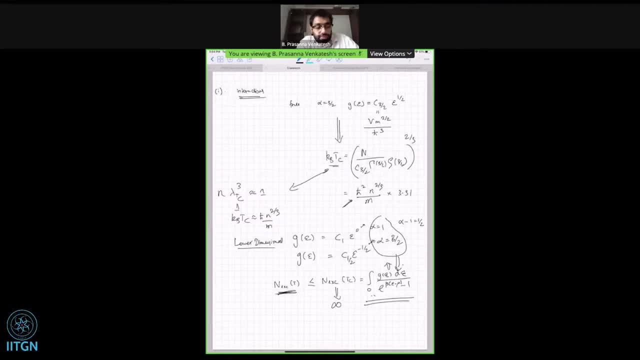 right, Correct. So yeah, that is not very clear to me because, in principle, any anisotropic harmonic trap or that would give me some anisotropy measurement, right. So how are we saying that? No, no, no, no, no, Look carefully, There is a very important feature. So, even so, 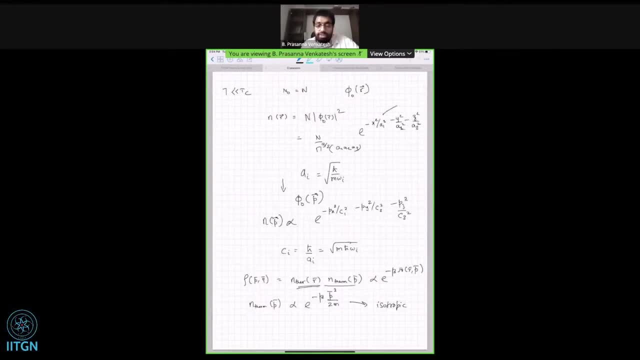 the momentum distribution and the position distribution for a classical gas in some harmonic oscillator. they are independent of each other. This is not a quantum mechanical thing. So, for example, what I am saying is: if you look at the higher states of, if you want, 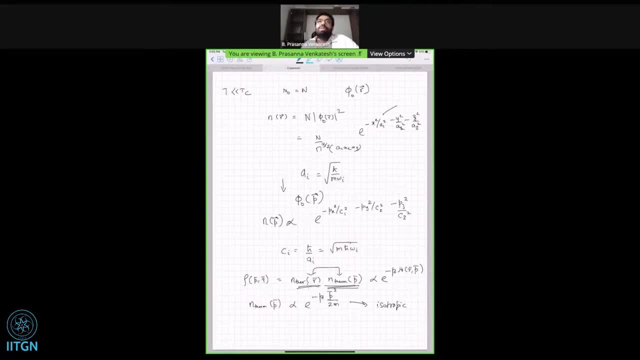 okay, you can say: well, all that is happening is my atoms are occupying higher states of my oscillator, So why are you using classical? I am using classical because once KBT is greater than H bar omega, I can just use a classical harmonic oscillator. Now, in a classical harmonic, 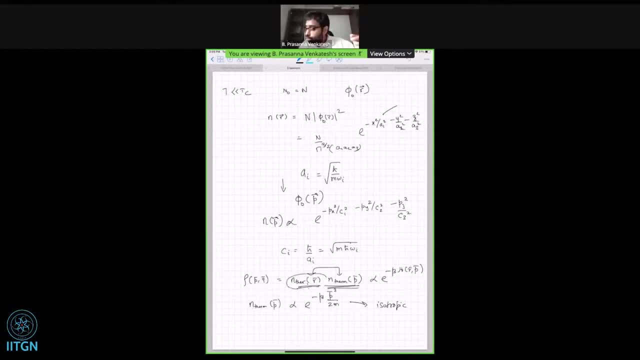 oscillator potential, independent of the. you basically have E to the minus beta position distribution, E to the minus beta P squared by 2L. So once you integrate out the position dependence, the momentum distribution is always isotropic in a classical gas. 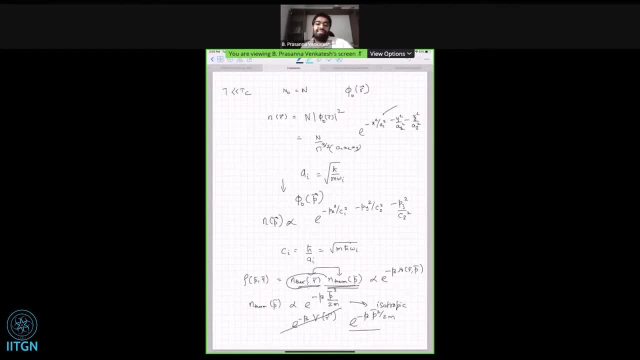 Yeah, I get that. I am saying that this, the anisotropy, it could be just a result of the anharmonicity of the trap itself. Okay, Right, How are we claiming that? that is, that all the items are in the ground state? 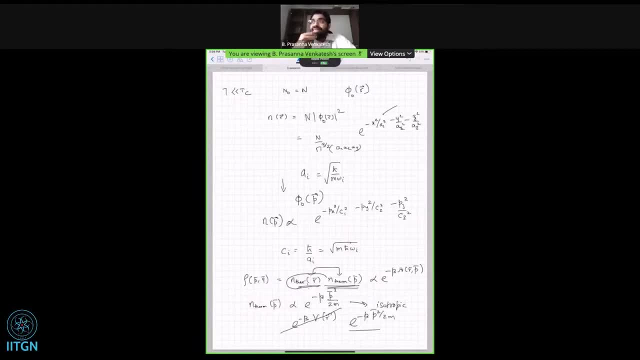 Okay, Okay, So there are two answers to it. The point is if you are occupying. the only way you see the anisotropy of the trap is if you occupy a certain quantum state of the trap macroscopically. Otherwise this large density peak. I will not even see, I will. 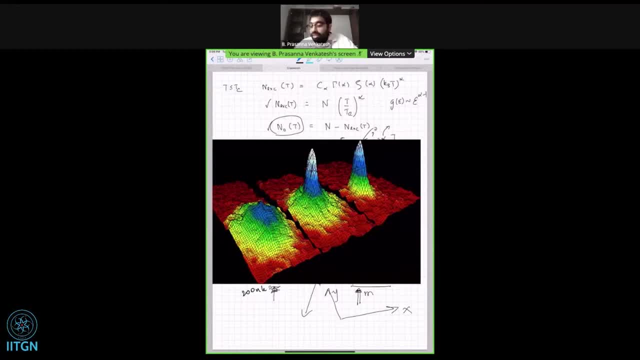 only see this Maxwell peak all the time the left peak. Okay, Now the second question as to how do you know it is the ground state. this we can measure, Because I can measure the widths of this. Just I can measure this n0.. These pictures. 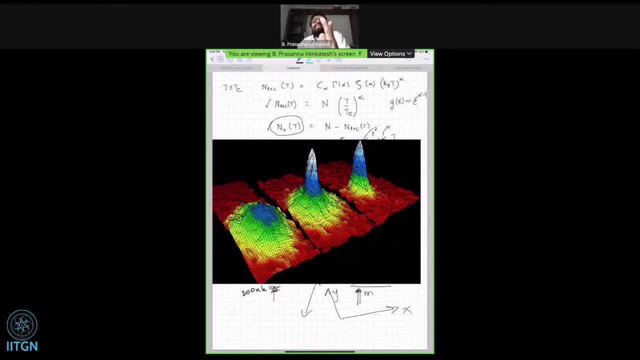 have position resolution. I can actually measure this width, I can change my trap and actually can check That. check has been done- That it is really this: a is actually square root of h, bar, m, omega. That you can really see. Okay, I get it. 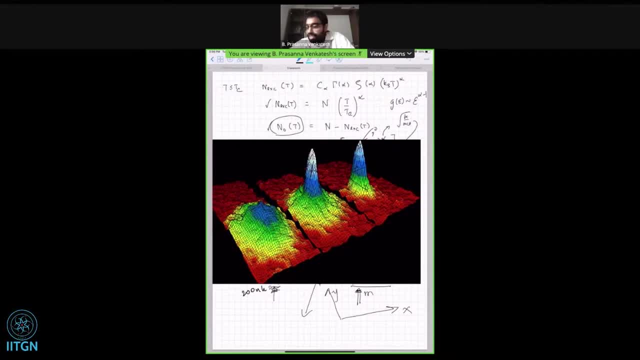 Okay, It is not. it is not. it is by no means a fluke that you get this, Okay. Okay, So there is. there are a couple of question, and let me see. The first question is about Riemann. 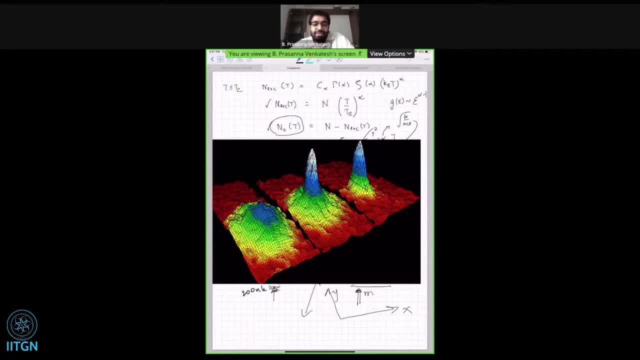 zeta function. Okay, So I using Bose-Einstein condensation to prove Riemann hypothesis is not very easy or it is not obvious, but there are some indications as to how could you not prove, or at least you can sort of physically see, the Riemann hypothesis. There are some. 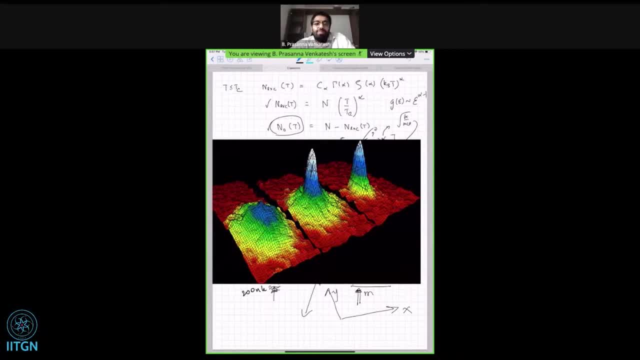 very cool works by many people, like Carl Bender. There is some by Michael Berry. I can maybe put together a bunch of references and tell you. rather, Swagata, I answered Kishore. I do not know if that was good enough or if you have any questions. 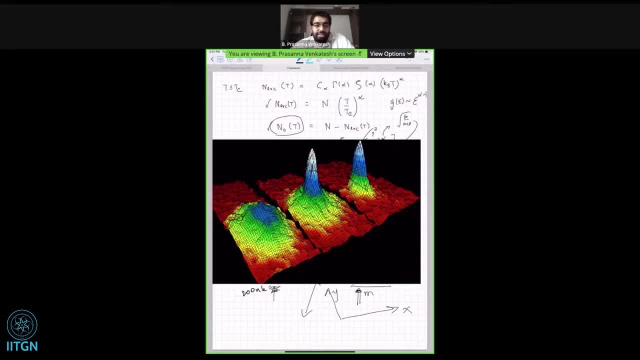 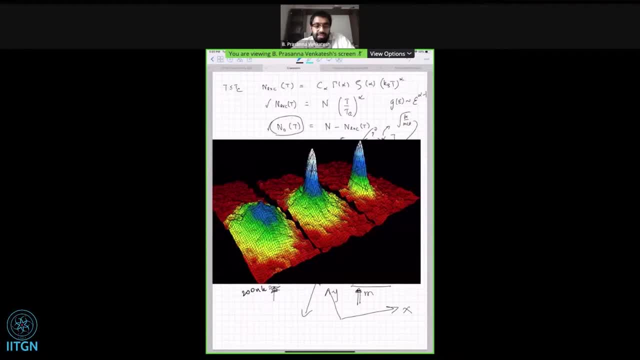 is another question from Norman. Does shining laser for imaging DCs disturb the metastable states? the bzs are in. Excellent question, Norman. Yes, This is again a very important thing, This measurement: when you actually shine lasers, what happens? 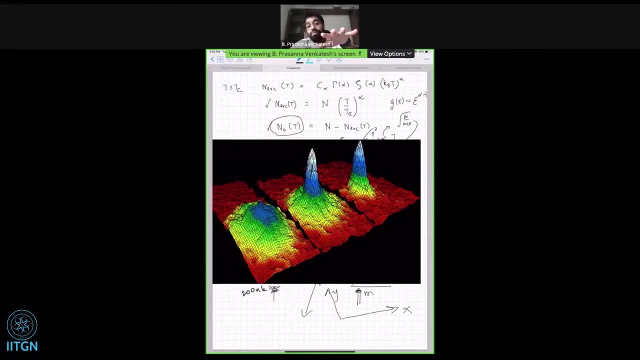 is basically the atoms absorb and make a shadow, but then they will emit. So when they emit spontaneously light, then because you're emitting light and light has momentum, you get a recoil kick and, as a result of this, you basically kill the condensate. the condensate atoms leave the trap. more importantly, 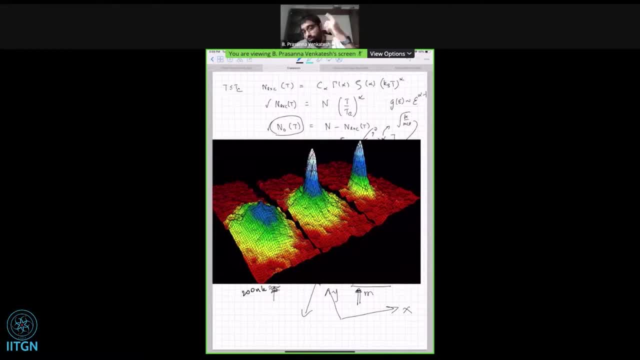 when these transitions are also such that sometimes you might go to the excited state and may not come back to the same ground state that you want, because the traps are also very sensitive to the internal state of the atoms. so you essentially in this process kill it. but the beauty, if at all, 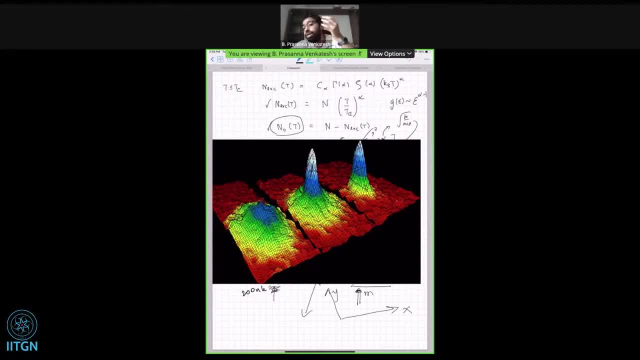 i have the time and i get to. it is now. you can do some cooler ways to image the atoms without killing them. for example, you can put them in a cavity and really see the atoms by looking at the cavity transmission light and this doesn't directly sort of kill the atoms. you use light. 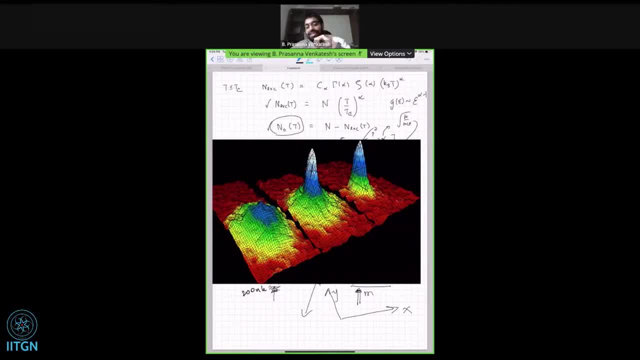 that is not precisely at the same frequency as the transition frequency of the atoms, and so that way you can also get basically an image that is is really, really non-destructive in that sense. okay, good, so if there are no further questions, you can go to the. 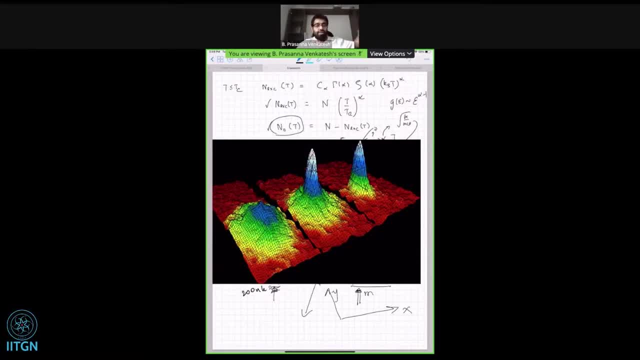 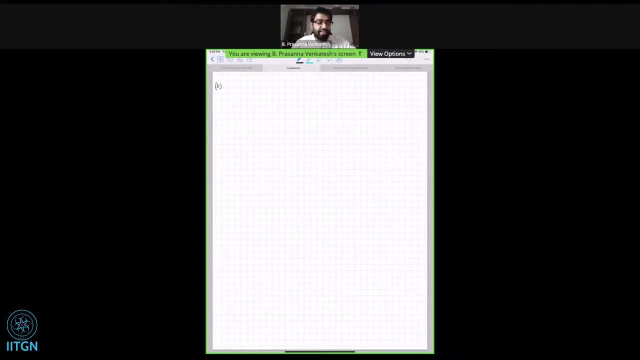 second part of our lecture. okay, so let me just get some water and then i'll keep that all right. so now let's look at, for, for all these reasons that i mentioned, i want to really define a boson strain condensate in a slightly more sophisticated way, and this will also set us up. 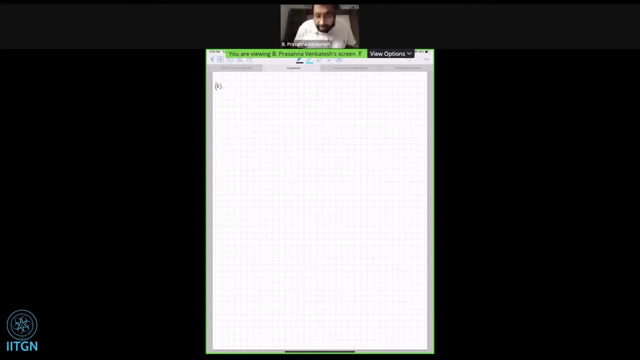 nicely for the kind of things we want to do in the future. so i'm going to go ahead and start with the first part of our lecture, which is what we're going to do next in terms of describing the condensate itself. okay, so this part is about off diagonal long range order and i'm just going to 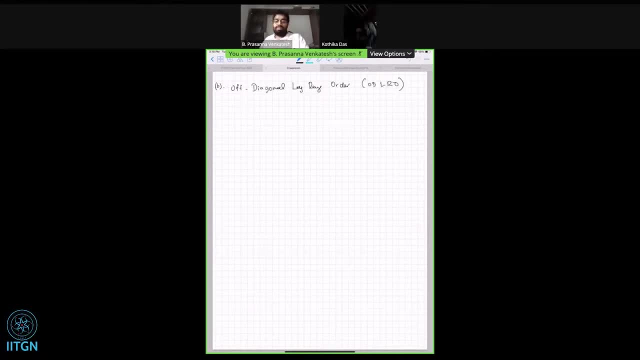 use this odl ro as this abbreviation, right, so apparently, long word, long phrase. okay. so now, uh, the idea is, if i want to talk to you about this, one needs a little bit of background on a few things. one is basically the idea of a density matrix. you need some idea of basic. 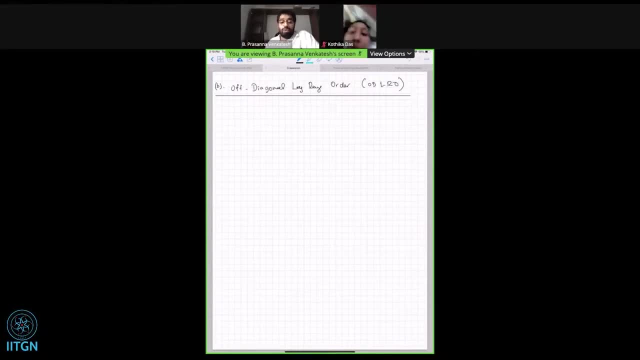 many body physics and a little bit of second quantization. what i thought was- i would try and give a very quick primer to it- this is by no means going to be an exhaustive thing. my notes are going to be somewhat more exhaustive than what i'm going to talk about and if you want, you can take a look. 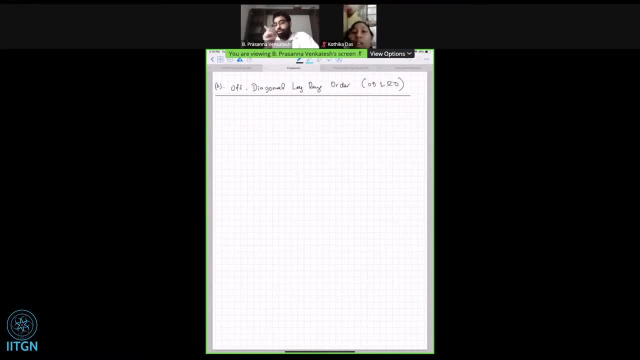 at the notes, and there are several excellent textbooks on this, including the one that i just brought up, because i just want to give you some idea of what you might be interested in. somebody can take this one because i'm interested in studying the um, i can, i can again give. 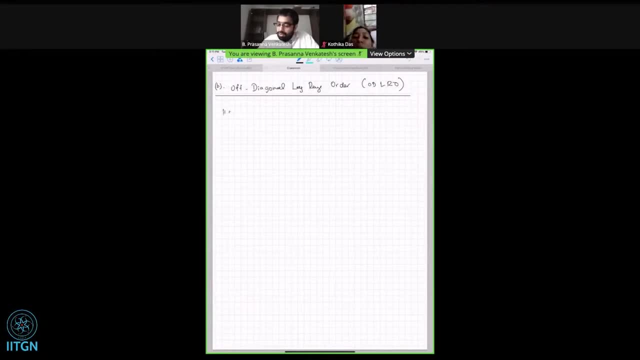 references, if you're interested, or this kind of physics. okay, this is just many body physics, right? okay? so now, what is the? what is a density matrix? because what i'm going to talk about is the off diagonal elements of intensity matrix describing a gas of bosons. so i have to first qualify and 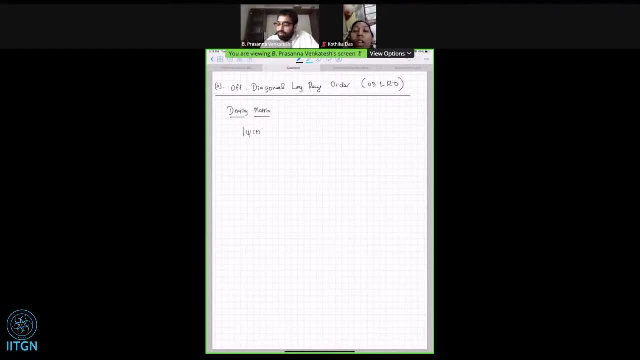 quickly point out to you what is the density matrix. typically, if you have a quantum system, the state of a quantum system is described by this state vector in the hilbert space and the delta. delta is what you have in this space and when you start doing this thing, you 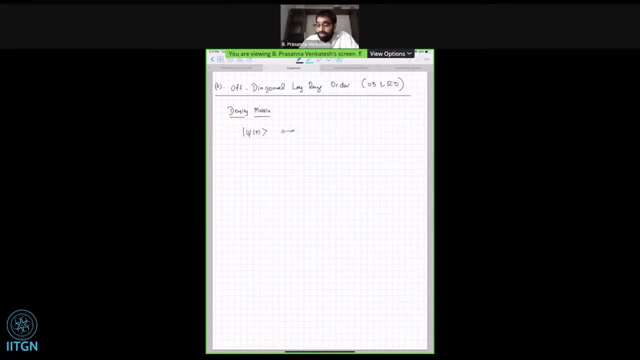 in for a single particle. you can either describe it by such a state or, if you want, you can also think of the positions based wave function. this is also completely fine. so this is again a equivalent description of the state of a quantum system. when, when you can, really when you know. 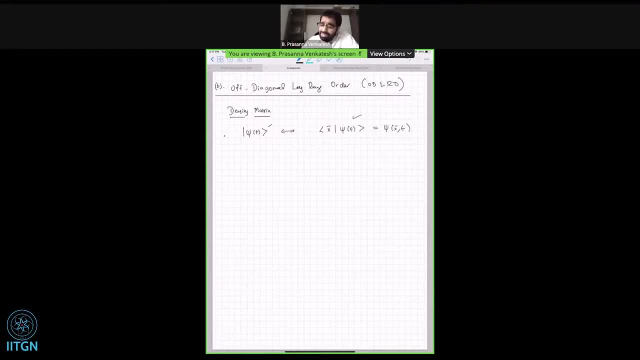 exactly what is the state that it is in. but sometimes you're not able to. you want descriptions of the state of a quantum system when you only know the description statistically okay. so in this case you do not know which wave function or which state vector represents the atom or the or the 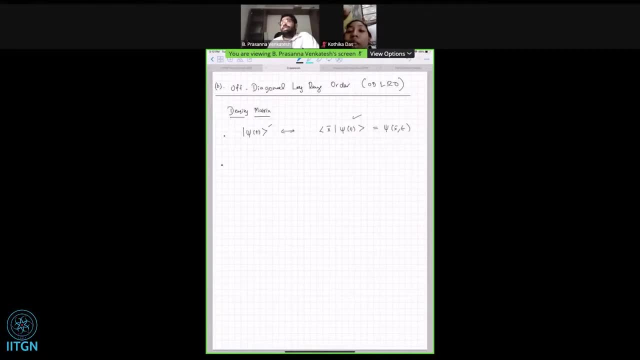 system and you only have statistical information about the probability to be in different state vectors. okay, and in this situation one needs to describe a quantum system by an object called the density matrix. okay, and there are many examples of how and when density matrices are useful in quantum mechanics. 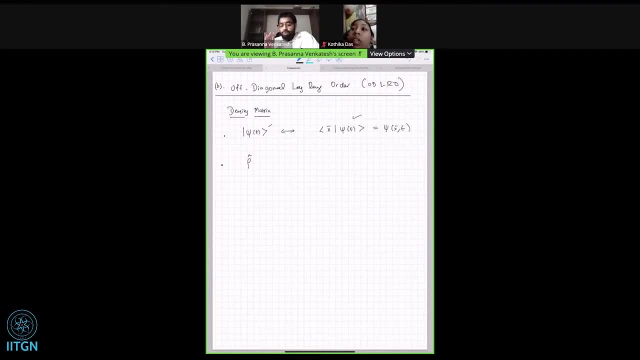 but in our lectures i'm interested in only one example of such a density matrix. such states like psi of t are sometimes called pure states, and the state that i'm going to describe now, which is not a pure state, which is a canonical thermal state of a system, this is basically 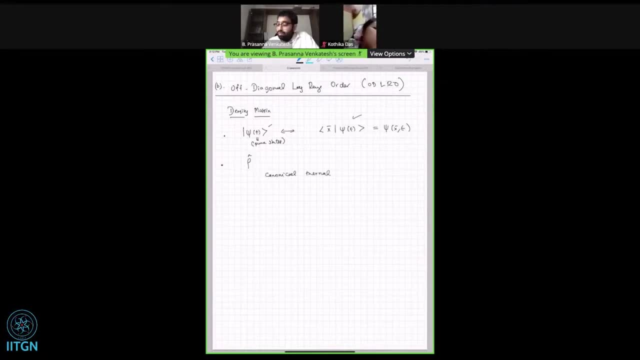 the system, the state of a quantum system that is in equilibrium with a bath at some temperature, t. okay, then the density matrix corresponding to that system is basically given by the following operator or matrix, whichever way you want to look at it, okay, where z is just sum over n, e to the minus beta, e, n, and which you know as the partition: 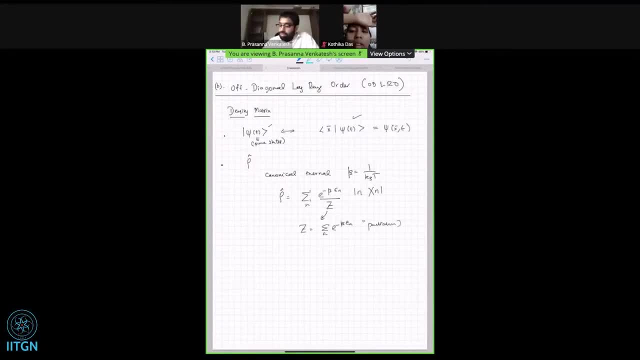 function right. so this is one example of a density matrix and this is the only example of density matrix i would need. and, of course, if you had a pure state, it also can be represented by a density matrix or a state vector, but it is just given by psi of t, psi of t and these n. 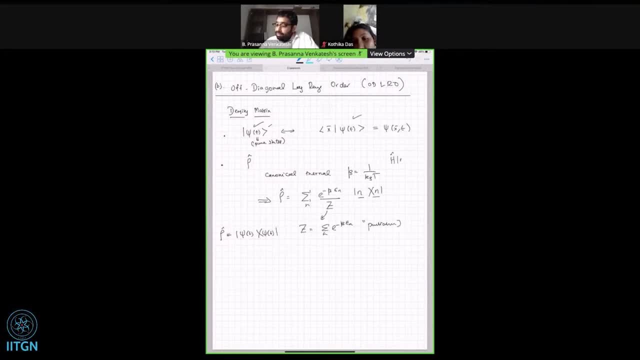 n is nothing, but they are the eigenstates of the hamiltonian. okay, i hope this is clear. so So this is true in general for a single particle system: n particle system, whatever it is, a quantum system, whose state when it is in some thermal equilibrium, you can always describe it via such density matrices. 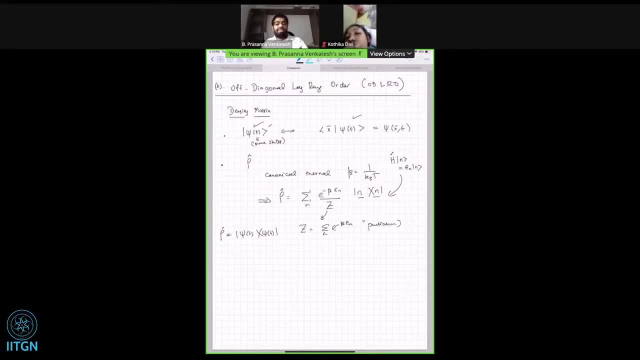 So this is the idea of a density matrix. But this density matrix has some very nice properties. For example, I'm just going to list these properties and you can try and do or think about them. So this is normalized as trace of rho is 1.. 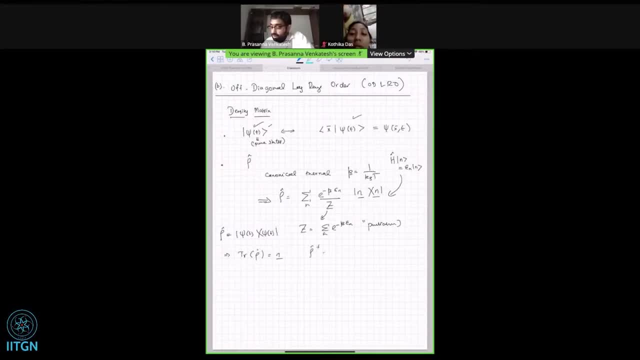 And this is Hermitian. It is positive definite: All eigenvalues are greater than or equal to 0. And because of this trace property, the eigenvalues have to be, and positive definite eigenvalues have to be between 0 and 1.. 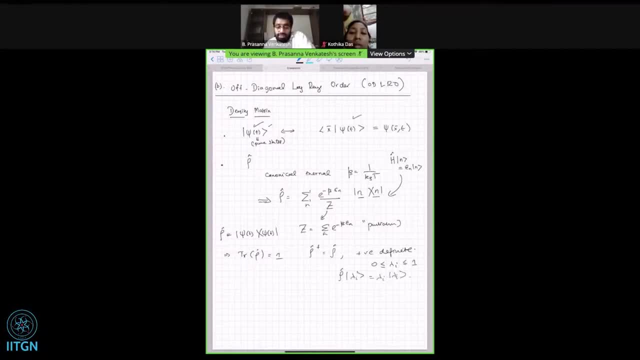 These are important properties of density matrices. So now our whole point with this off-density. So we're going to look at the. So we'll be interested in the low temperature behavior of an effective or reduced density matrix of an interacting bosonic system. That's where we are going. Okay, that's the path. But as a precursor to that, let's look at a single particle. 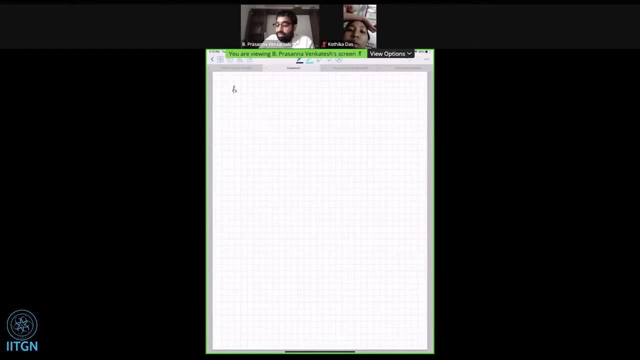 A single free particle, just as to see what are we going to discover. consider just a single free particle in a box of size L, right, and the Hamiltonian is just p squared by 2m, And you can easily solve the energy eigenvalues. and we want to write down the density matrix for this object. 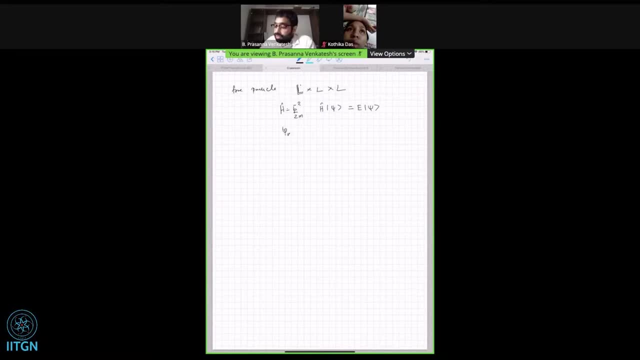 Okay, so now the eigenfunctions are precisely: E, k is just h bar squared, k squared by 2m. We've seen this a few times now, and this is just 1 over. the volume e to the i, k, dot, x right and k, of course, is quantized in units of 2 pi over l. 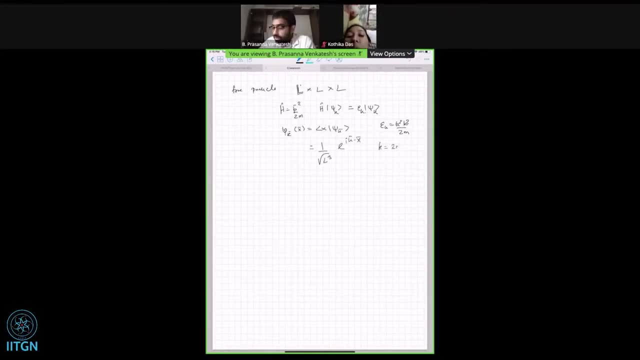 This is the boundary condition induced effect, right? Okay, so now what is the density matrix? It's very simple, So it is just rho t sum over k, e to the minus beta, e k, psi k, psi k over the partition function. Okay, so now let's look at this thermal density matrix in the position basis, right? 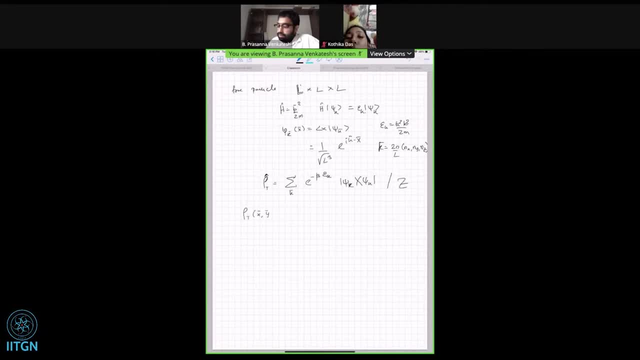 So I want to look at the matrix element of this density matrix in the position basis. Okay, you can see that the density matrix is just just 1 over the volume e to the i, k, dot, xy. Okay, So if I plug that in and use the property of my wave functions, after a little bit of algebra I'll see that this goes to something very familiar and neat. 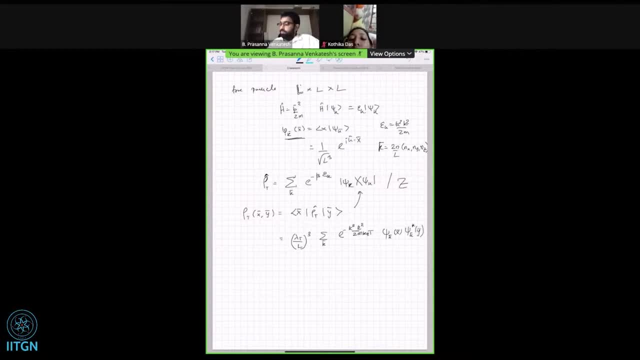 Okay now, these are just momentum wave functions. So this just becomes e to the i, k, dot, x, Okay, y, okay. now if you take the thermodynamic limit- i mean here it's not you shouldn't call it the thermodynamic- but just l becomes very large, it's just a single particle. then you can convert this. 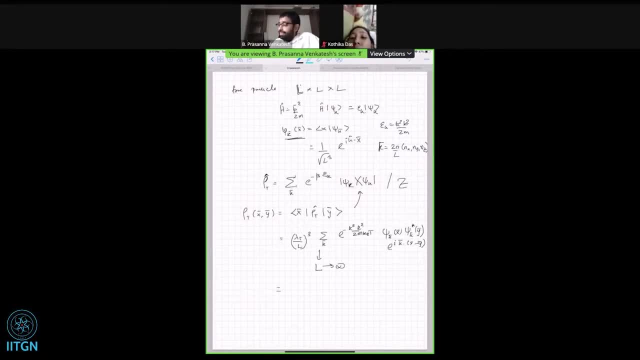 sum into an integral, and once you do that, this is nothing but the fourier transform of a gaussian centered at k, equal to zero with respect to this position, x minus y variable. so fourier transform for gaussian is a gaussian right. so rho t of x- y very nicely becomes this: 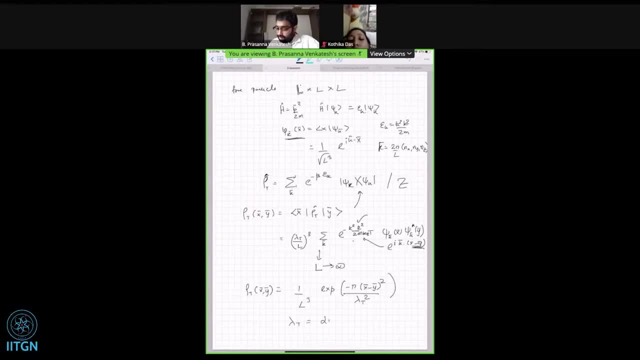 this lambda t is our old friend the thermal de broglie wave. now if you plot basically this, this roti is just depending on you, magnitude of x minus y, whole squared. so if you plot this off diagonal element of this single particle density matrix, this, what you see is a gaussian dq right the dk length scale, as you. 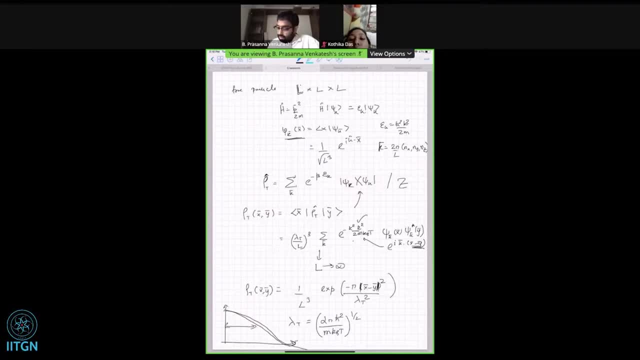 this is basically rho t of x- y as a function of x minus y. the dk length scale is basically given by the thermal de broglie wavelength factor. in the limit t goes to zero, you essentially get something interesting, which is this lambda t basically becomes extremely large. 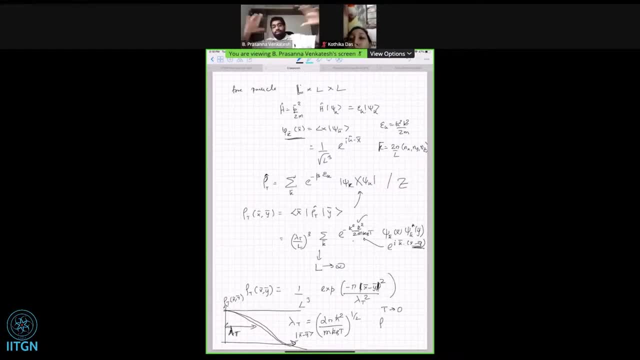 and rho t of x- y remains non-zero up to very large separations. this is nothing but the mathematical, uh, or the more sort of rigorous way of talking about this cartoon picture we saw in the beginning of the class right, so we saw as the temperature became smaller. 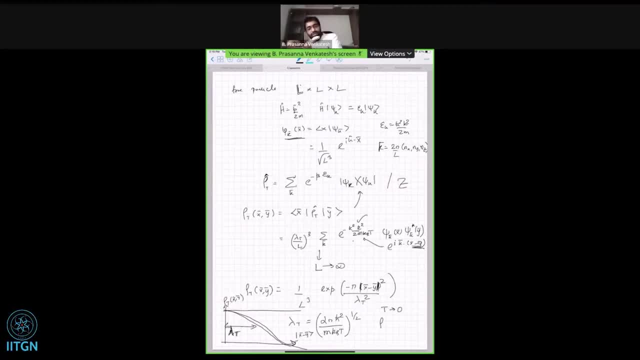 each of these single particles that are bouncing around, their de broglie wave then became larger. a quantum mechanical consequence of that is that if you look at the density matrix and look at the off diagonal elements, the off diagonal correlations of the density matrix increases as temperature goes down. this happens for a single density matrix. now we will see. 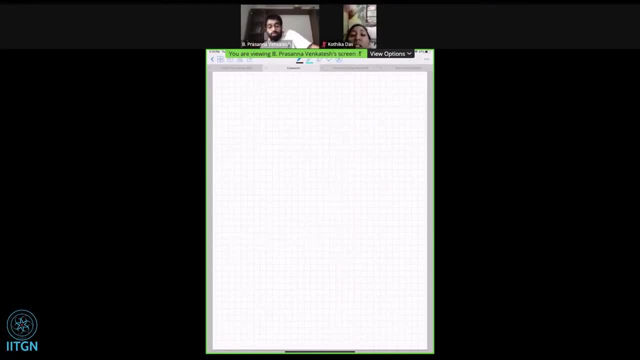 when we look at multiple particles now, starting with a two particle to warm up ourselves. that is a that. this same effect is enhanced when you add statistics, when you add the fact that you have to have wave functions that are symmetric under permutation of labels of particles, when you 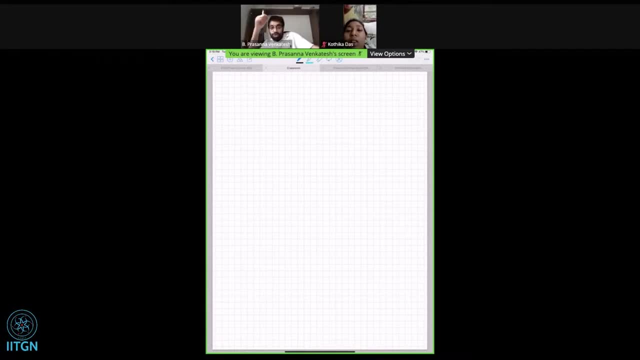 add this identical particle nature and the statistics- bosonic, statistical nature, the symmetry of this wave function. this enhancement is, if it is, if the particles are bosons, they have to satisfy this. i'm just mentioning for completeness: if they are fermions, they should be anti-symmetric, right, and they have to be symmetric if they are bosons, okay. so now. 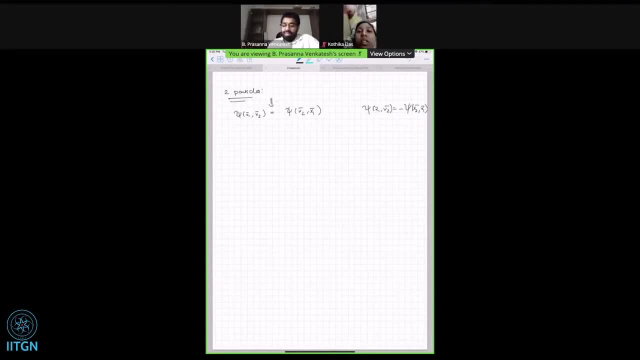 let's consider two non-interacting bosons, free particles, and write down their thermal density matrix, right? so my hamiltonian now is h1 plus h2, right? and so this is p1 squared by 2m plus p2 squared by 2m. incidentally, remember that whenever i have a hamiltonian of a bosonic system of 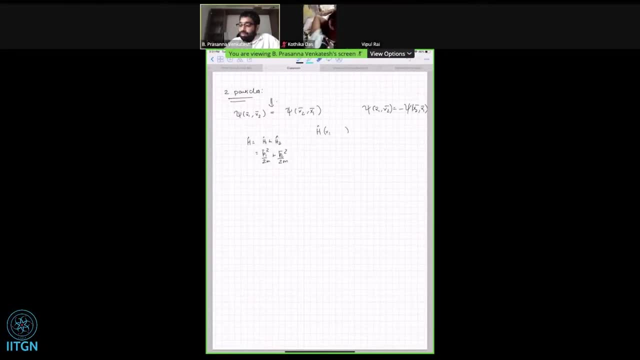 particles with x. uh, let's say x1, x2 to x, and and you have psi 1 of x1, psi 2 of x2. okay, so now if i consider energies, uh, the total, this is the individual energies. so the total energy eigenstates, psi of x1- x2 satisfy e1 plus e2. psi of x1- x2. 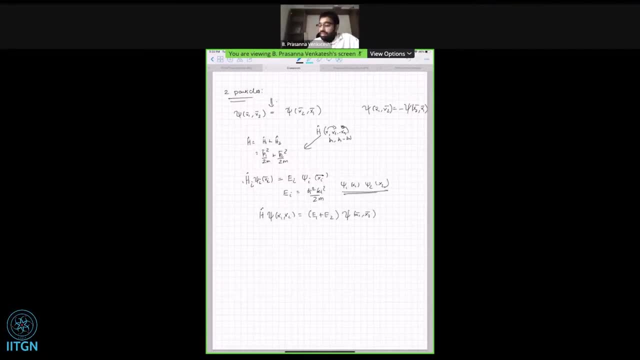 these can be products of these two wave functions, obviously, but we have to account for the symmetrization. so the right eigenstate in this case, as you know, is just psi e1 x1, psi e2- x2 plus psi e1 x2, psi e2 x1, right. So this symmetrization is needed for the correct. 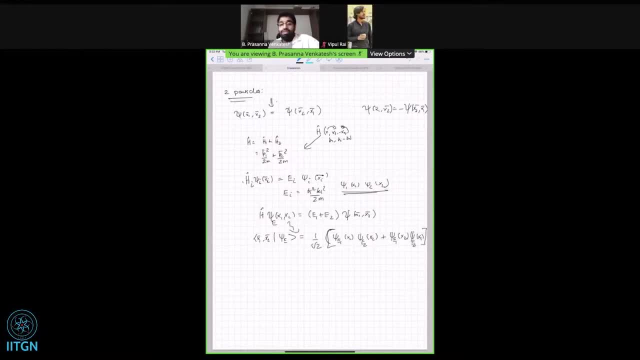 two-particle wave function. okay, So that is our two-particle energy eigenstates, eigenwave functions, which means now I can actually write down the thermal density matrix for two particles as 1 over z, sum over e, e to the minus beta, e, which is e1 plus e2, psi e. 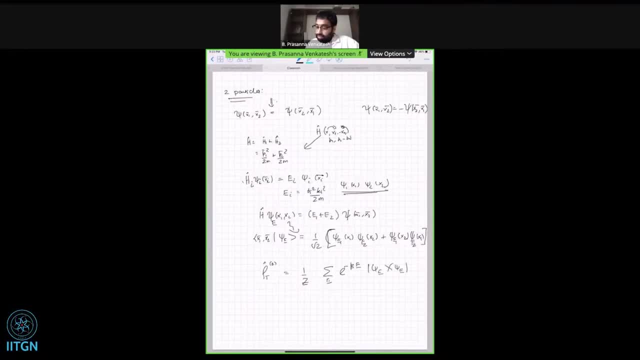 psi e. Now I can look at the full two-particle density matrix. right, Of course I will have to supply x1, x2, rho, t2, y1, y2.. This is not like a single-particle density matrix. This is 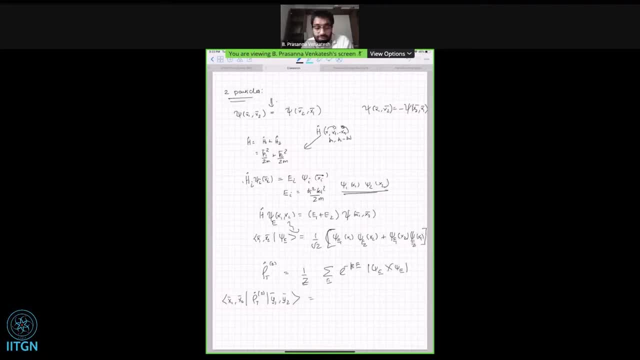 the two-particle density matrix. Right So now, but that's no big deal. I can easily still write it in this two-particle way as: sum over e, psi, e, star, x1, x2, psi, e of y1, y2, e to the minus beta, e1 plus. 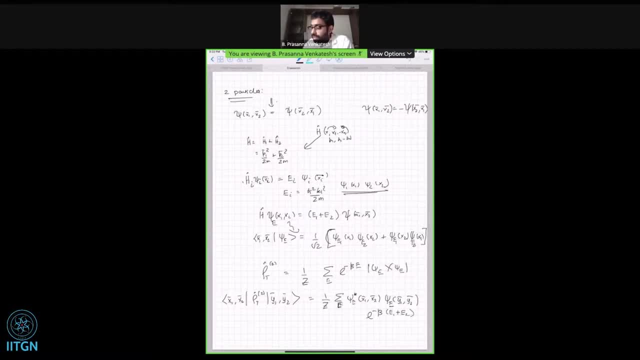 e2.. That is sum over e, is just sum over e1 and e2,. okay, So once I do this I can plug in the two-particle density matrix right. So now I can easily still write it in this. 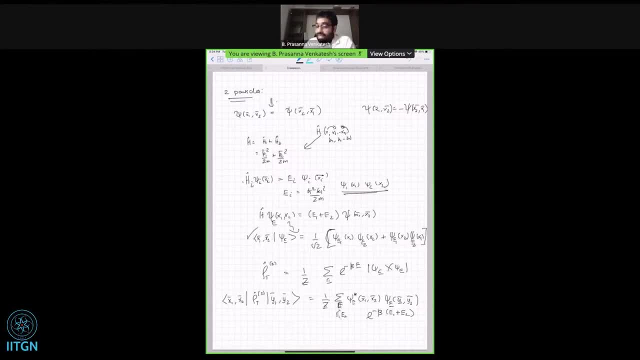 two-particle density matrix, right. So once I do this, I can easily still write it in this, my symmetrized form of the wave function, and after a little bit of algebra. so let's call this rho t. let's call this function matrix element x1, x2, y1, y2.. This object 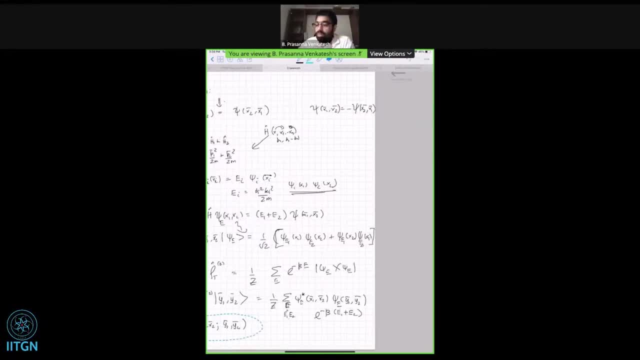 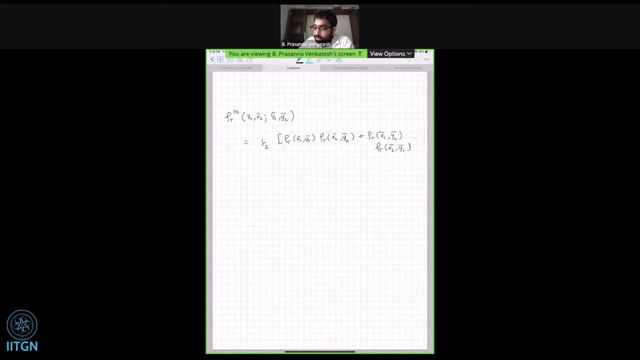 once I plug in my form of the wave, function becomes very neatly into the following object: It just becomes half rho t x1, y1, rho t x2, y1, y2.. It just becomes half rho t x2, y2, plus rho t x1, y2, rho t x2, y1, rho t x1, y2.. 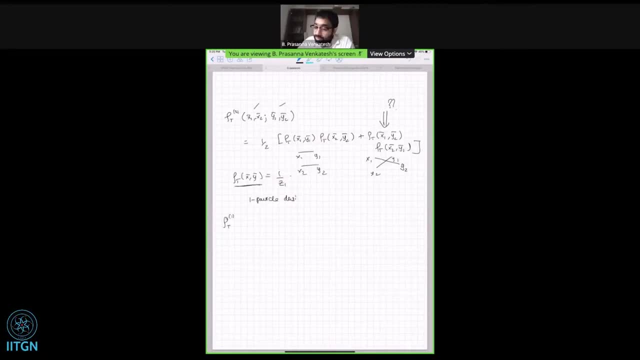 are just the regular one variable and take the diagonal of this two so we can write it as rho t2, x, x2, y, x2. okay, so if you know a little bit of quantum, uh, quantum optics or quantum information, this is somewhat similar to taking a reduced density matrix, where we are removing one of the particles. okay, and when? 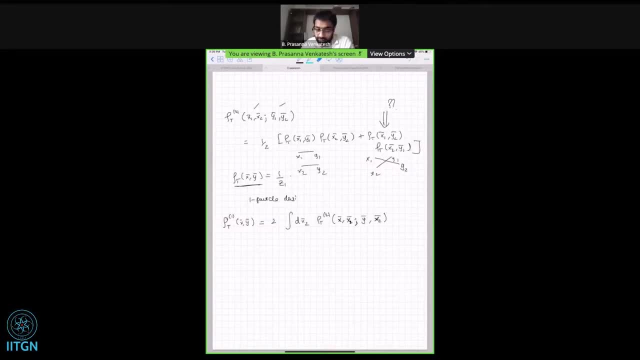 you do that. you see, after a little bit of algebra, you will be able to write this precisely as the sum of your ordinary one particle density matrix plus an additional term from x, x2 rho t of x2- y. remember that we evaluated how this object looks. this basically: 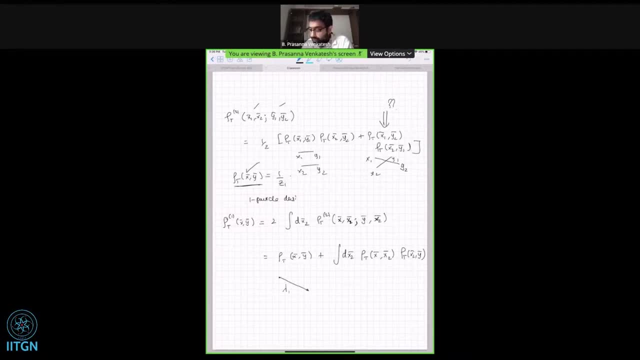 tells you that there is off diagonal elements have some correlation. the correlation length x and y should be less than or equal to lambda t. up to lambda t, you have correlations. now, in addition to that, due to the, precisely due to this symmetrization or statistic, 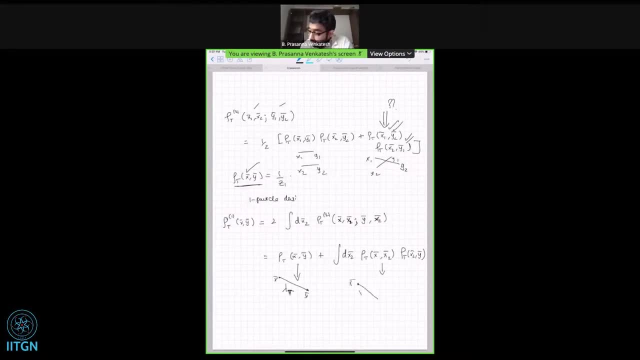 you get an extra correlation that is elongated. the correlation becomes more collective in this sense. so you can x and y, can be even two lambda t separated. even then you will get some finite correlation. so essentially there is uh, the press, the symmetrization of your wave function. 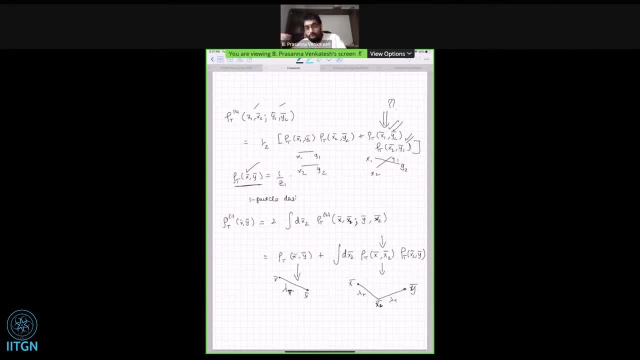 or statistics, really leads to a more, larger correlation, and this correlation length becomes larger and larger and larger as temperature goes down. we've shown this in a toy way for a single particle, and we now want to go on and describe the behavior of such the: the analog. 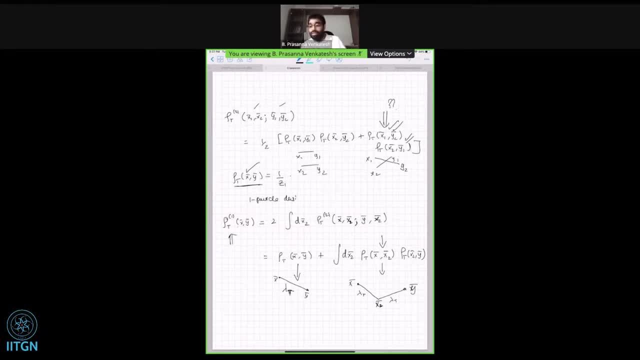 of this single particle density matrix for n particles. that is what we want to do and that is where this off diagonal long range order will come. okay, so that's let me go to that, and in order to do that, it is going to be very painful to. 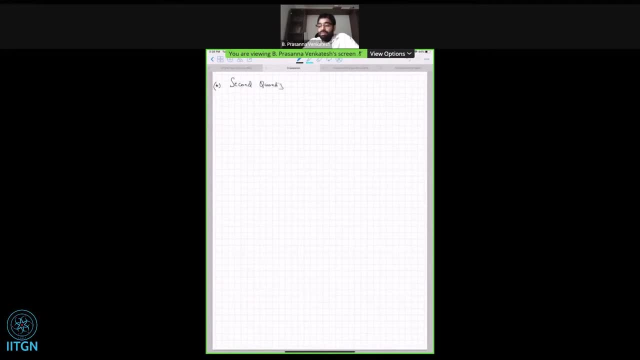 continue to symmetrize it, which is the language in which one formulates many body physics of identical particles. okay, and i want to talk about that next. okay, maybe i can have a very short break here and if there are any questions about this part, the next part is going to be the formalism of second quantization, which will be useful. 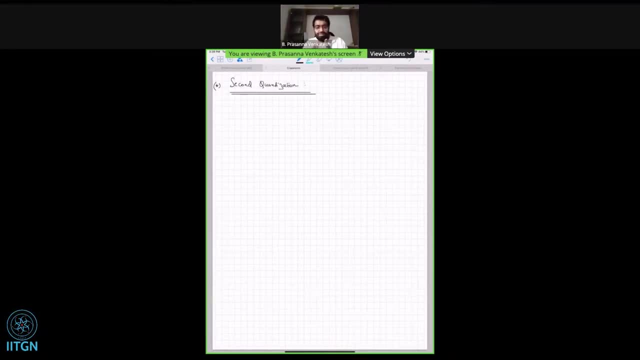 for the rest of the lectures, but very briefly. so any questions. okay, so there's one which says temperature of the heat path starts fluctuating. will we still get a boson strength condensate? hmm, learning with holger camping. so that is the basic, basic question. 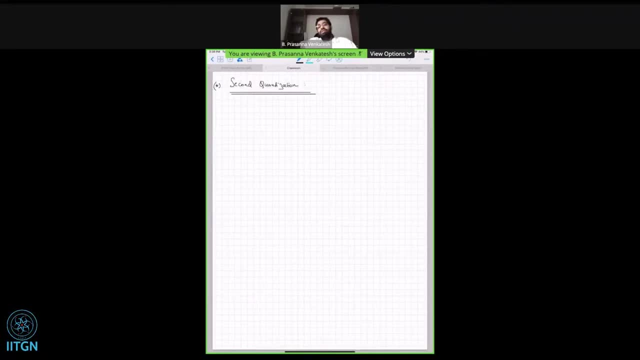 it depends. so i do not understand what it means for the temperature of a heat path to fluctuate. so the idea is that heat paths in thermodynamics are very huge objects which have very fixed, uh unfluctuating temperature as such. so if you have a bath that is finite sized, 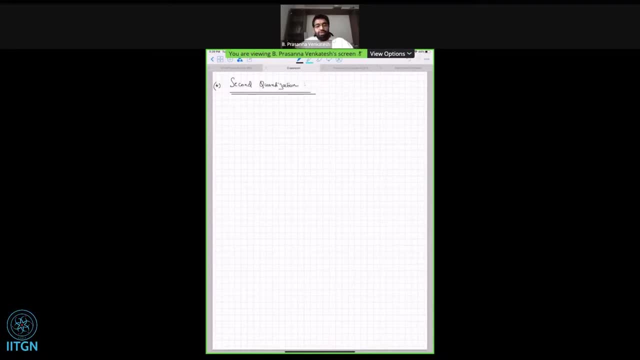 or some small system, then its temperature fluctuates咨A-Êiz. Our heat path is essentially no longer a heat path. 咨A-Êiz. Our heat path is essentially no longer a heat path. So I think this question is not very clear to me. but we can have a discussion. 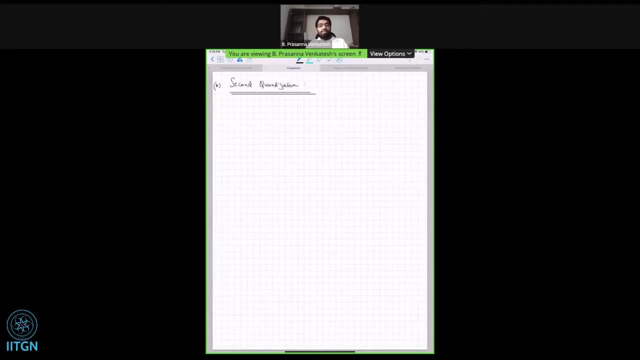 What does the dimension of 3 by 2 mean? You mean this alpha being 3 by 2, right, So it's not dimension 3 by 2.. What it is is it is telling us about, basically, the density of states. 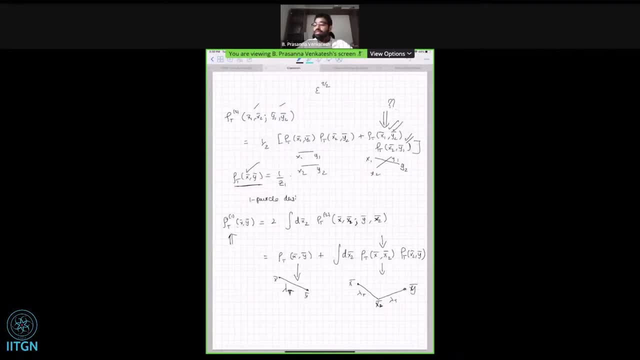 So we worked out the density of states for a free particle, last class. You can go back and look at it. It goes as: g of e is e to the 3 by 2 minus 1.. So the 3 by 2 is very physically easy to explain. 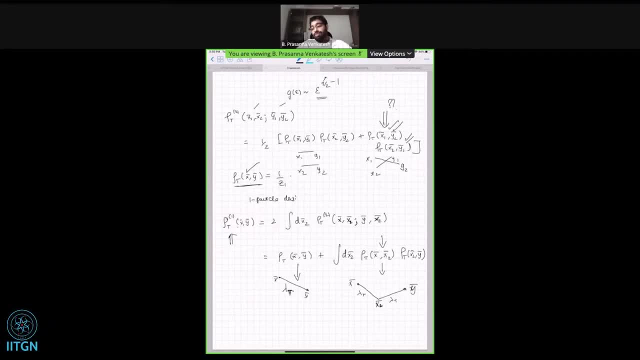 This 3 comes from actually the spatial dimension of the system, That is, three dimensions, And this half comes from the fact that the energy and the momentum for a free particle are related by a p squared. So if you have a relativistic gas, for example, this would be like some Cp- massless, relativistic gas. 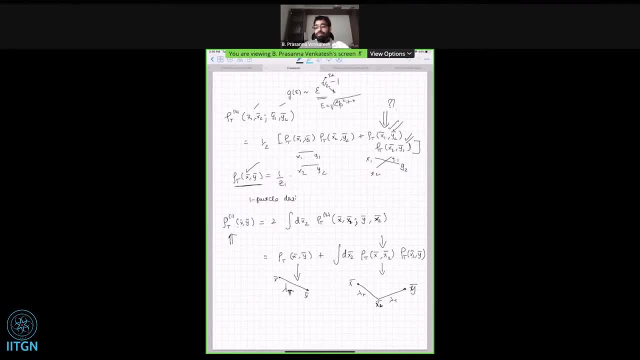 Or it could be Cp, Or it could be something more complicated if you have an actual relativistic particle and so on. So it really depends. So it gives us both the dispersion relation and the dimensionality of your system. decide what your density of states is. 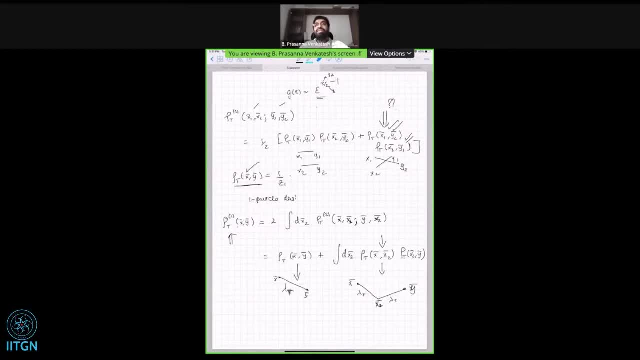 That is all. that is That 3 by 2 doesn't always have to do anything with dimension. That factor, this alpha, of course changes when you go to different dimensions. It is not directly the dimension. Okay, Good, Since there are no questions, let me move on. 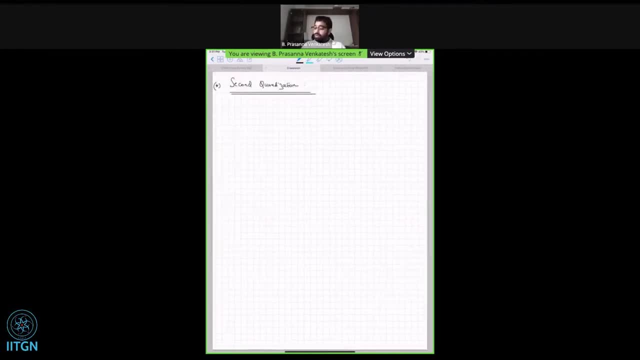 And we want to now write down the equivalent of this single particle density matrix for a very large collection of particles, n particles. Okay, So in order to do that, let's first understand a little bit. how does the Hilbert space, or how do you describe mathematically in quantum mechanics many particle systems? 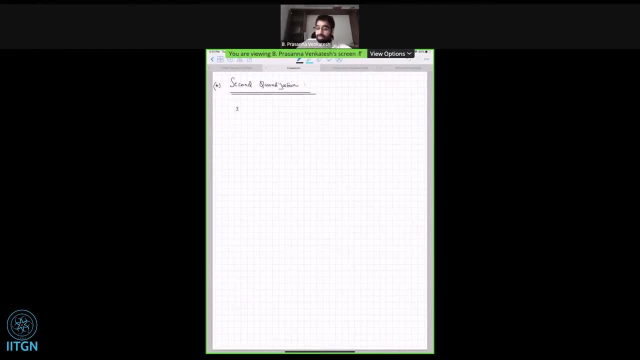 Okay, So a single particle Hilbert space is very simple. Single particle states: you already know very well. We've talked about them just now. We were talking about three particle and so on. So what are single particle quantum states? You can define them in many ways. 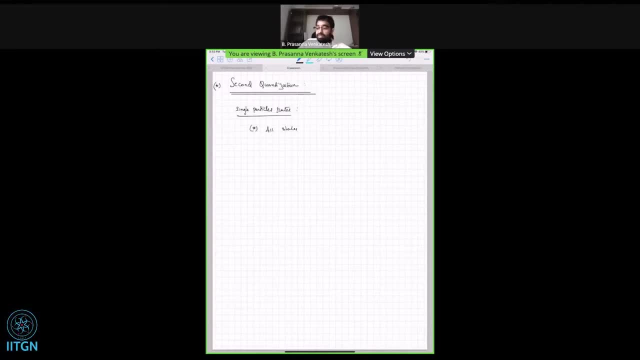 All states that are spanned right, for example, by the eigenstates of a position operator right in three dimensions. These are all single particle states. Similarly, eigenstates of momentum operators span the state of single particles. Or if you have some single particle Hamiltonian right, p squared by 2m plus some v of x, all the eigenstates of this system right, the span of all the eigenstates of this system. that is also called a single particle Hilbert space or a single particle Hamiltonian. 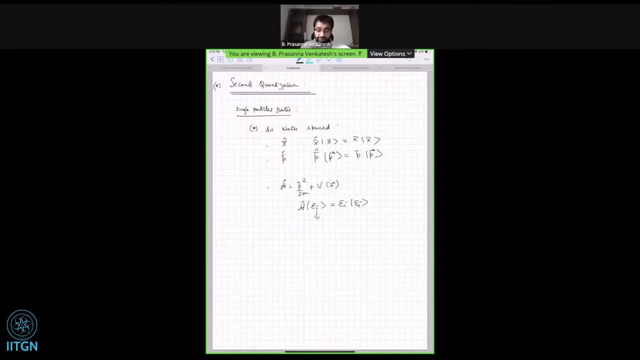 Okay, So we are not going to specify which we are going to look at, But let me denote by lambda i some general orthonormal means. lambda i, lambda j is delta ij. Of course this will be different if you have a continuous basis. 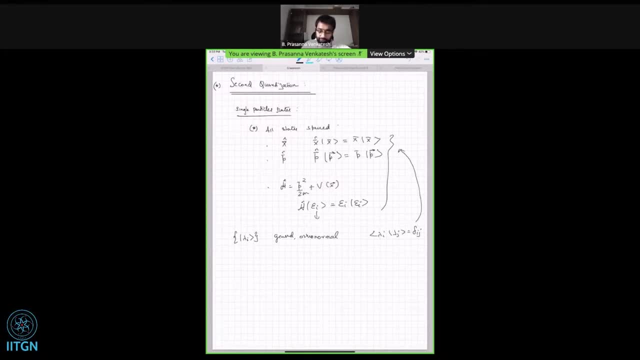 They will be delta normalized and so on. Then this is basically a general set of single particle eigenfunctions or single particle states. Let's consider such a single particle states And, of course, corresponding to each of these single particle states, you can also write down a wave function. 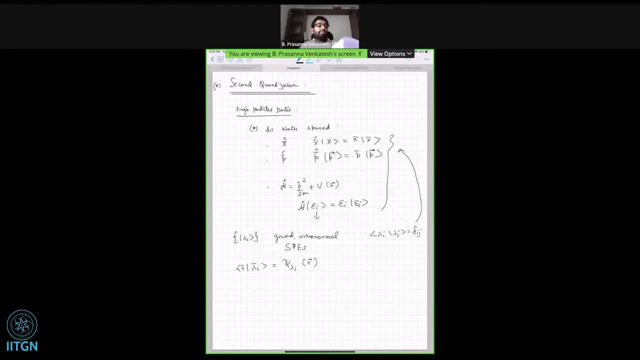 It's just the position representation of these single particle states. Now this is all for one quantum particle. So now how do things look when you have many particles? We already started discussing that for two particles. One way to do it is: I can basically consider: I'm just going to focus on many particles that are indistinguishable- bonons. 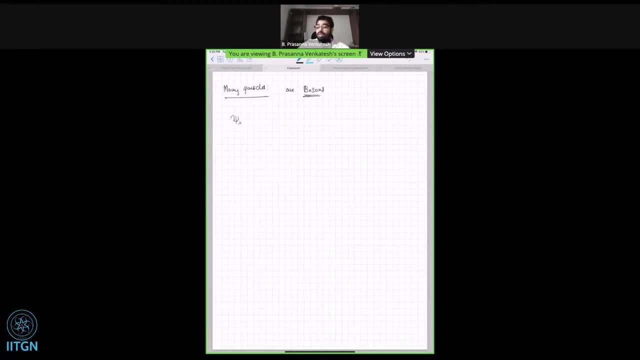 In this case, my many particle wave function, as we just discussed, is completely symmetric And that Particle label exchange. So in this case I have a system where my i particle is in state lambda one. Sorry, i particle is in state lambda i. 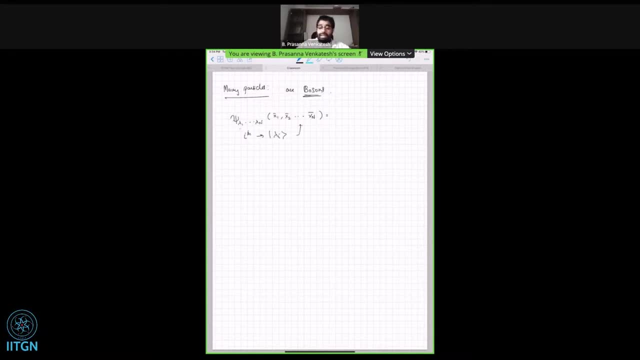 And this is the wave function corresponding to that, And I have to write it In this manner. Right, This is a product Form, But what am I changing? P, Basically is a permutation of X1, X2, Xn. 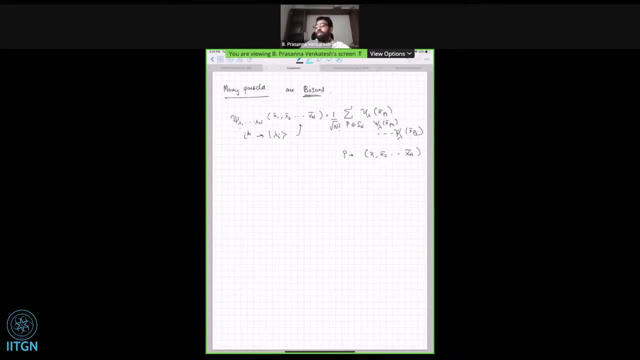 So I have to sum over every possible permutation and factor permutations possible of X1, X2, Xn. Of course I have to add another factor here. if basically different lambda i's can also be the same, because it's boson, I can have particles occupying many particles occupying the same single particle state. 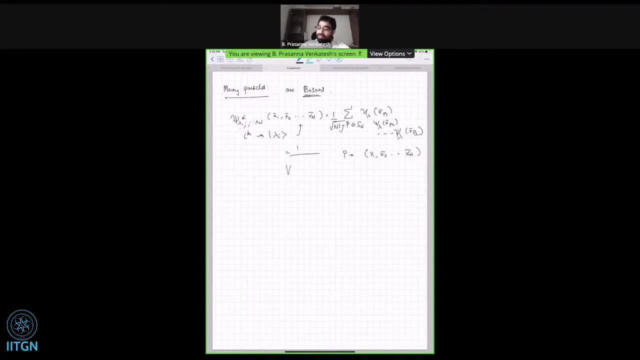 So, in principle, This normalization factor- I have written it wrongly in the notes- It will have a product of n i, factorial, where n? i is the number of repeated indices in this lambda one to lambda i. Okay, But anyway, forgetting the normalization. basically you'll have to sum over all permutation of the labels. 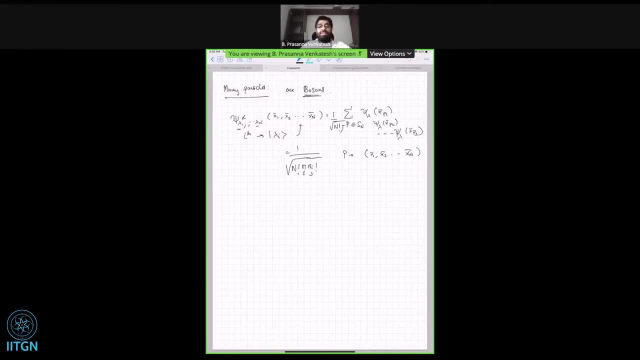 So this, the collection of all such wave functions on the collection of all such symmetrized states made up of single product, of direct product, of single particle states. This is, This is what is going to give you and Hilbert, space of many particles. 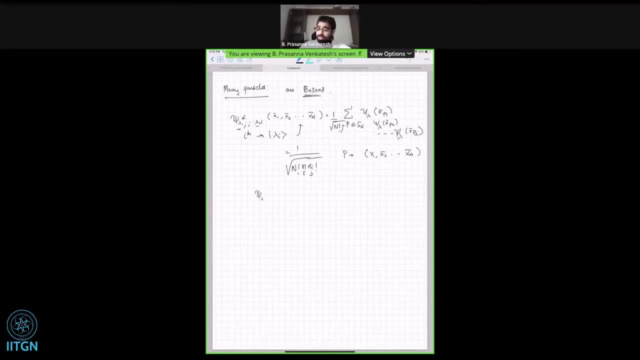 Okay, So now the key property of this, as we just saw, is that if I look at any permutation of the labels, I get back the same wave function, right. So this is the defining important feature of a many particle bosonic wave function. 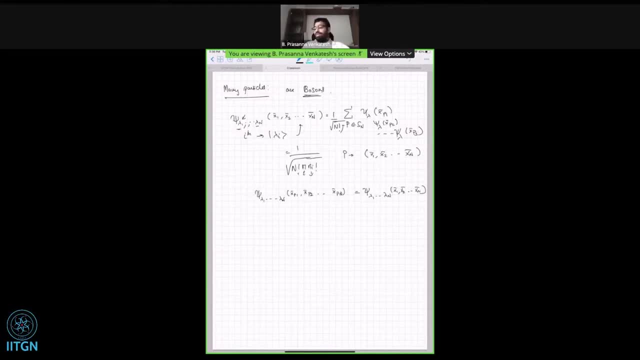 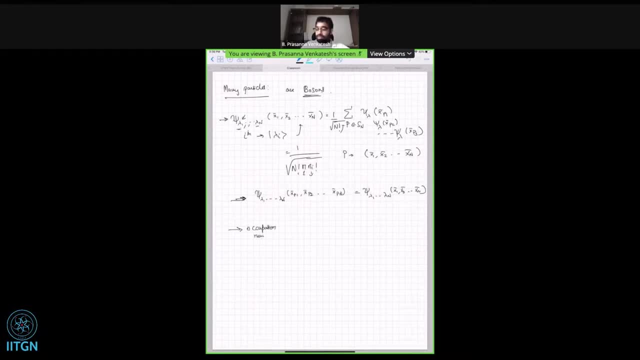 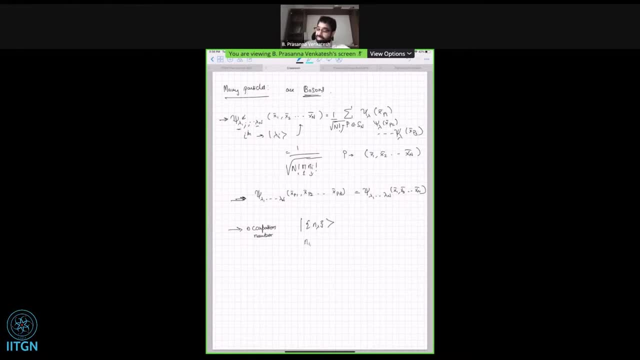 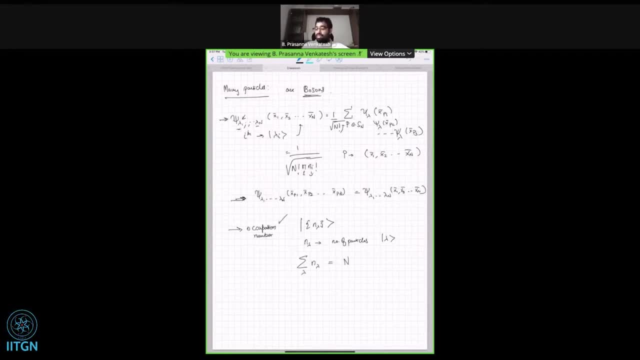 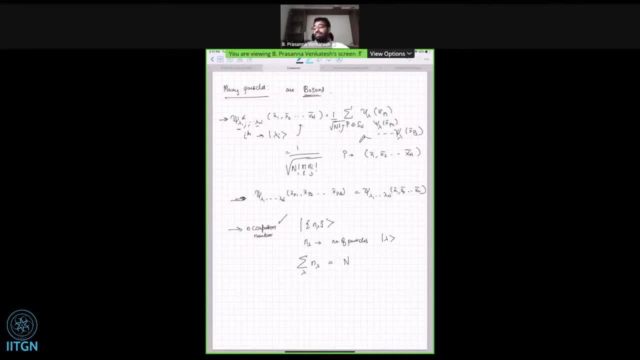 make a symmetrized wave function with the correct distribution of particles in the single particle states. Okay, And so such a basis of writing things is called occupation number basis and it's sometimes given the label fn. Okay, This is basically n particle space of bosons. 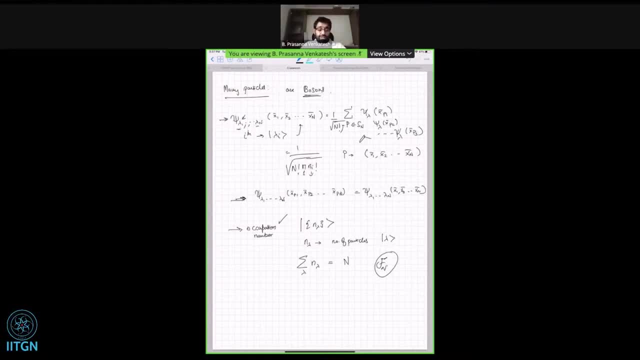 Okay. So now that's good, but that's still not enough for us. Okay, So we want to do a little better, which is- let me just connect this state and this wave function- What the usefulness of this state, as I just mentioned, is. as soon as you give me this, 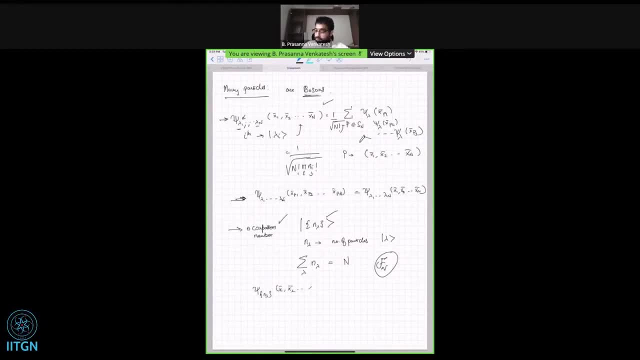 n lambda. I can write down a symmetrized wave function in this manner. Okay, And this wave function already has this property built in. That is what I'm trying to say. Okay, So in the notes I give an example of such a symmetrized wave function for three particles. 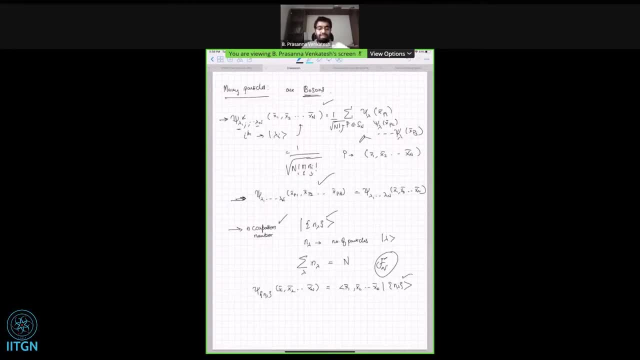 which is very simple. you can also play with it. Okay, So now this is good. This is a little bit of a simplification from this cumbersome many particle symmetrized wave function, But can we do a little better? Yes, 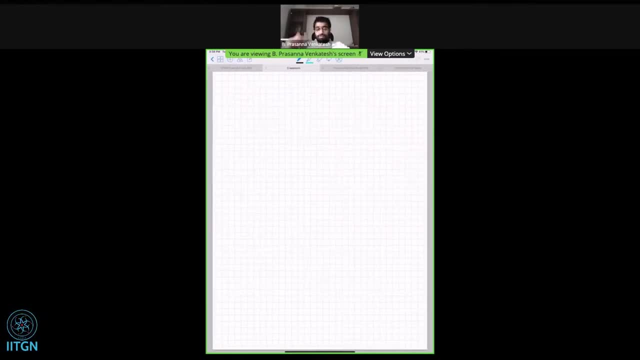 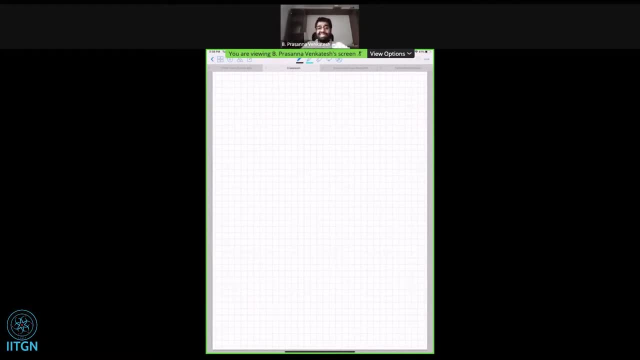 canonical and grand canonical ensemble, for example, the ease with which you can evaluate the grand canonical partition function for bosons as opposed to the canonical partition function, you might have a little bit of motivation that if you sort of release this constraint, that sum over lambda n- lambda should be a fixed n- you might actually end up gaining. 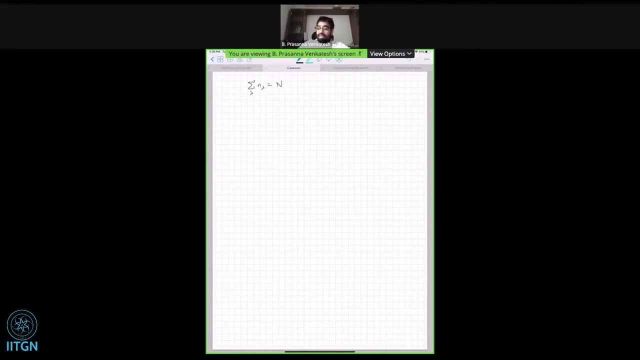 a lot. Hence we now consider an enlarged Hilbert space which contains states with different particle numbers. So this is basically called the POC Hilbert space, And this is the sum of systems with different number of particles. So for a kind of system that I'm looking at, this introduction is not- it is- very convenient. 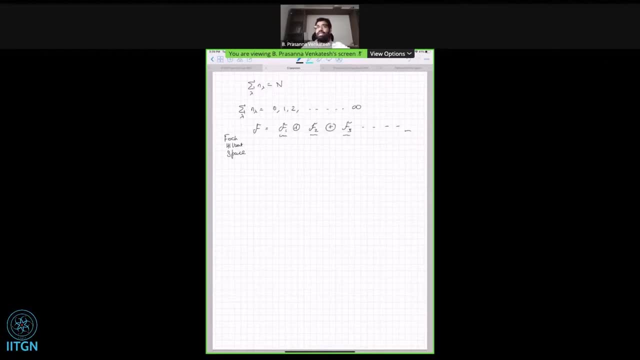 and it makes my formalism easy. but it is not fundamentally required because I'm not going to produce an atom or add an atom out of TINYAR. But, as some of you are listening to more deeper lectures since the morning with GR, or even 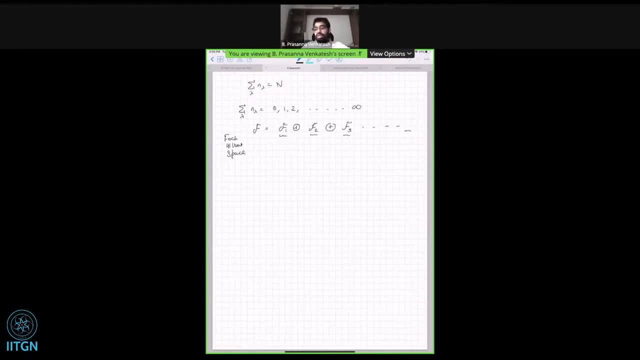 more importantly in Arquan's lecture, with field theory and so on. This is indispensable. if you have a relativistic system, you do not conserve particle number for fundamental particles and you can produce them from vacuum. So then this kind of a POC space is essentially the space in which quantum field theories 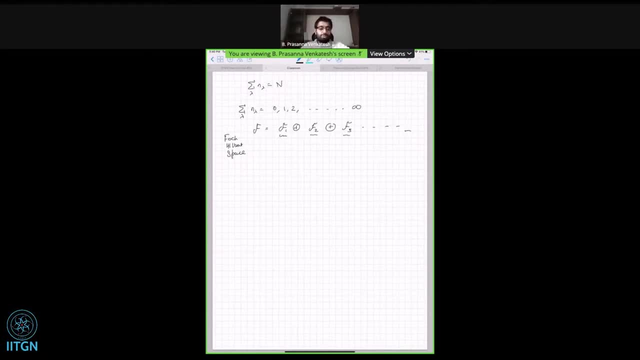 live. So just as a side note to people who are also attending those lectures. But here this is going to simplify our life a lot- I forgot the all important F0. Which is basically the quantum field theory. It basically has only one state, which is this very important vacuum state. 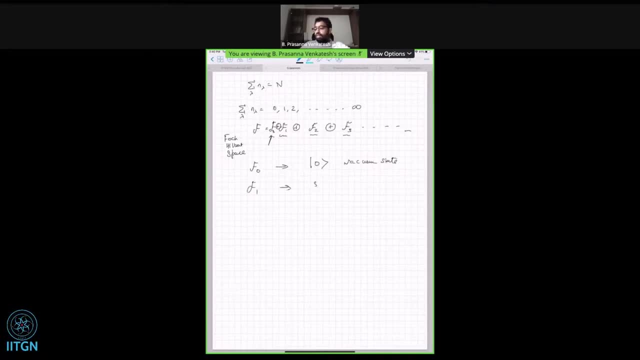 And F1 is our familiar textbook quantum mechanics case, where there is just a single particle space. Now why does this help? Why does introducing this help? The basic idea is that, in order to take advantage of this POC space, I have to introduce a very 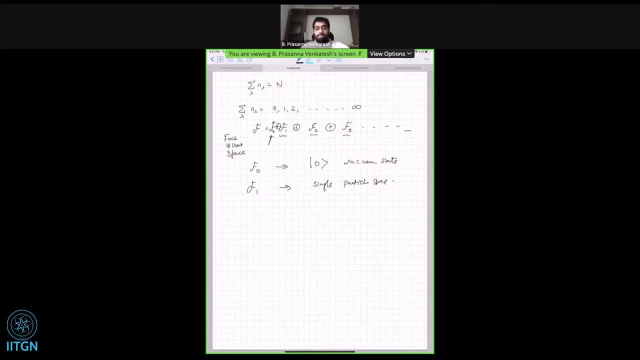 nice space, A set of operators. My life on this POC space becomes very easy once I introduce these operators that are called the creation and the annihilation operators, which you might have seen. This is a single particle: creation and annihilation operators. 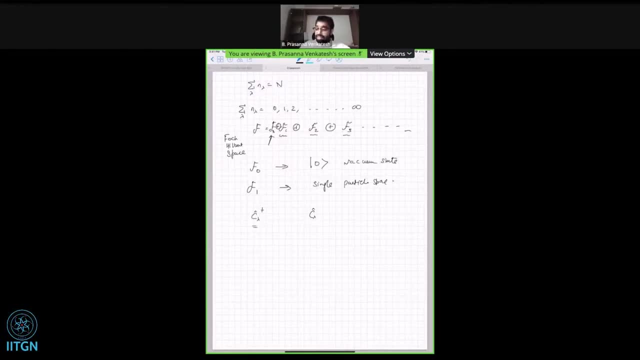 And these. you might have seen them in harmonic oscillators. This, basically: this operator creates a particle in the single particle state lambda. This destroys a particle that is already in the single particle state lambda. OK, So that Is going to make our life super simple. 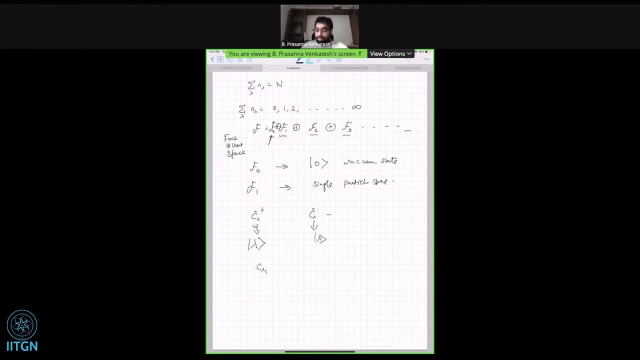 So if I start, for example, with an n-particle state- c lambda i, with n lambda 1, n lambda 2, n lambda i right, Some symmetrized n-particle state, So this is in this occupation number basis. 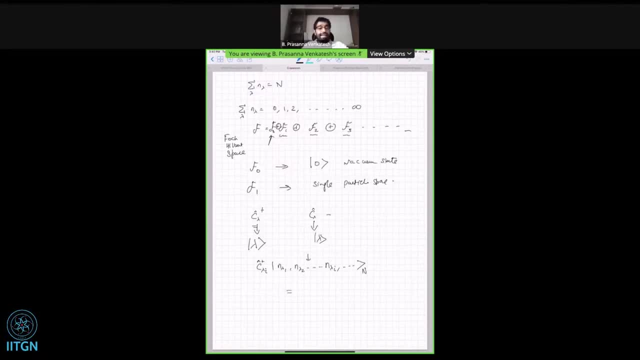 So then, if I apply this creation operator, I basically end up with n lambda i plus one factor, n lambda 1, n lambda 2, n lambda i plus one, blah, blah, blah, And now I am in the n plus one particle space. 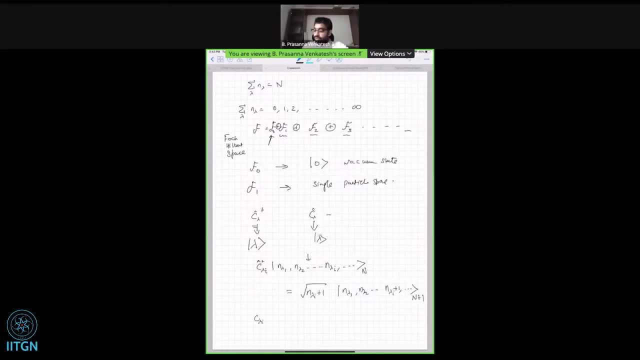 OK. Similarly, the reverse of it works for c lambda i. Then I get square root, n lambda i and then n minus one particle space. OK. Now The whole beauty of this Fox space and the whole beauty of this picture Is that, instead of worrying about this occupation, number representation, symmetrizing wave functions, 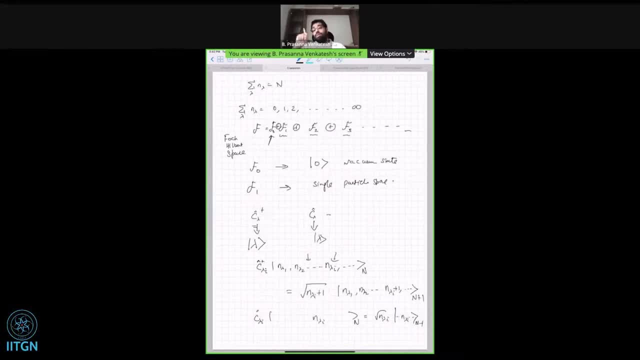 and so on and so forth, The fact that I should always get, I should always stick to states that have particular symmetry properties, even under exchange of labels. I can really beautifully encode them into the properties of these operators. more precisely, For bosonic systems, these creation and relation operators obey this very nice, important property. 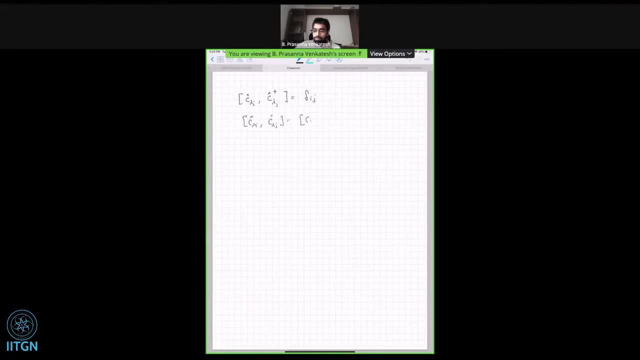 Right Equal to zero. These are called the bosonic commutator relations, And as soon as you take these relations to be true, Any n-particle space, Any n-particle space, Any n-particle space, Any n-particle state. 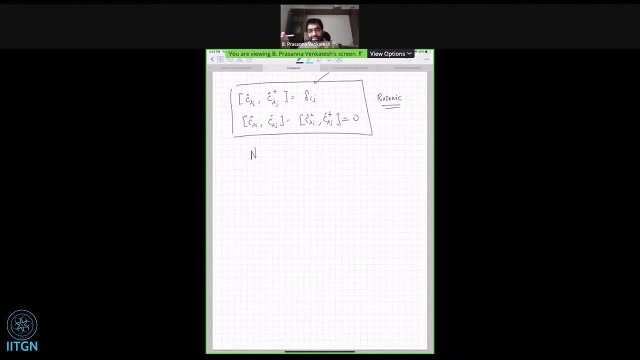 Any capital n-particle state that you produce by repeatedly applying these creation operators will, by definition, be symmetrized properly. OK, And that is the beauty of this. I'm not going to show that this is the case. I hope you can play with this apparatus and try it out yourself. 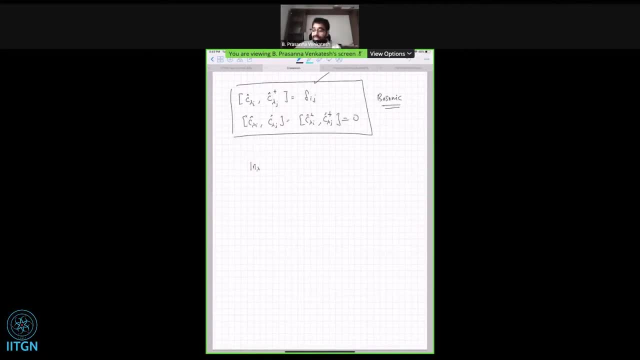 So with this I can really write a general occupation number state with n particles. So this is sum over i, n over i. This is sum over i n lambda i equal to n By simply in this form. So you act on vacuum repeatedly with these creation operators. 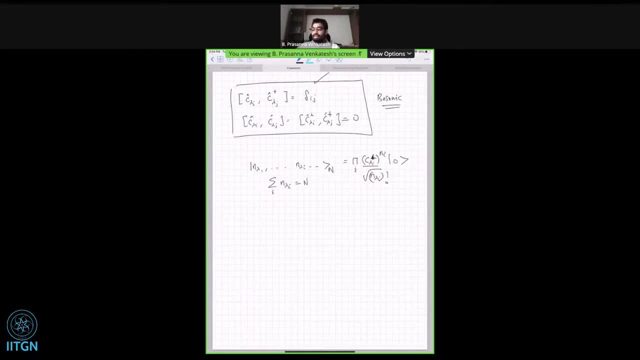 If you want to put n i atoms in c lambda in the single particle state, lambda i, you act c lambda i dagger n i times. OK, That's it. So now we have defined our Operators. Creation and relation operator, defined our space of many particles. 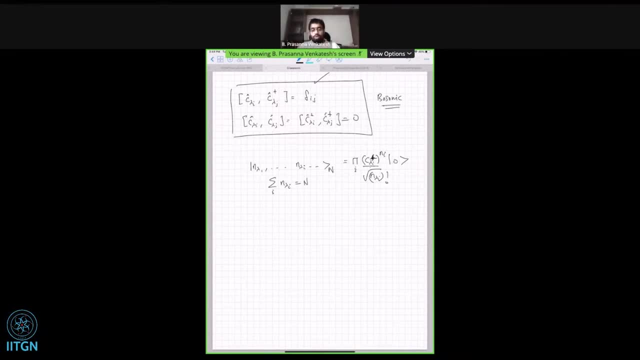 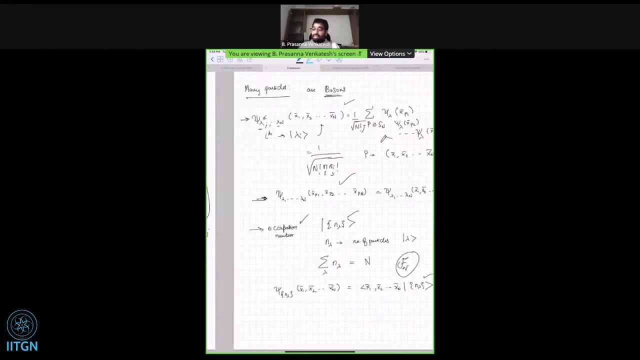 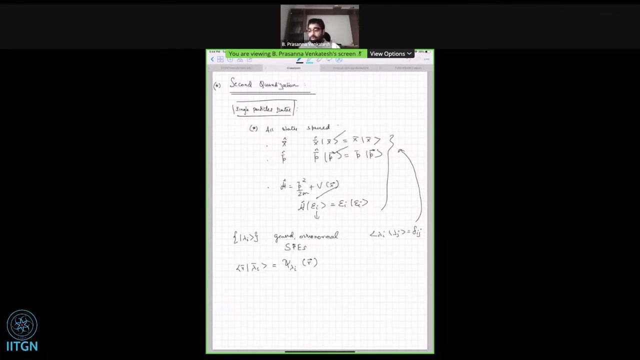 Now let's quickly go through some of these very important properties. of this, One very important property is that when I introduce single particle states, I said there are many different single particle states, So I can have x states, p states, eigenstates of some single particle Hamiltonian. 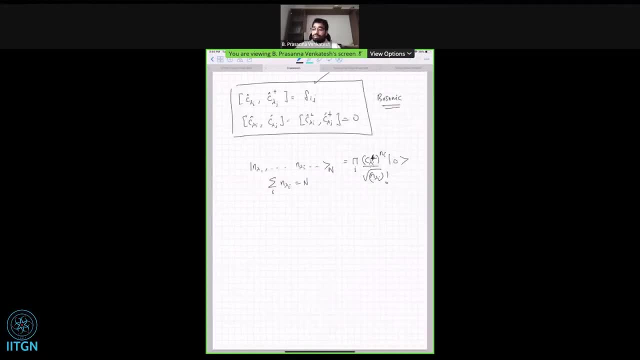 But I have introduced c lambda for only a particular set of lambda. Now what happens to my creation operators if I make a basis change in the single particle states? That is very simple. So let's consider c lambda i as the set of any creation operators or annihilation operators in for the basis lambda. 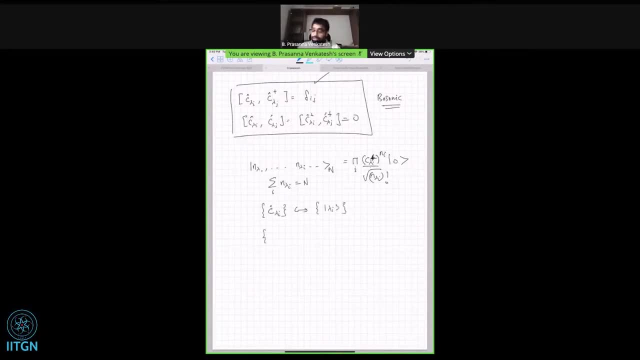 So this creates a particle in lambda And let's call c, alpha i, As the set of annihilation operators For another basis, alpha i. So this is some basis one, This is basis two. How do you connect the two? Very simple. 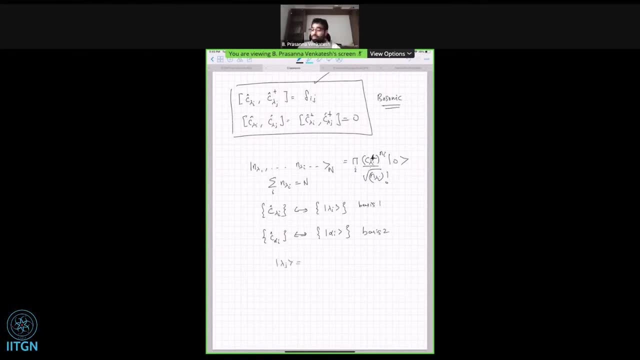 All that you need to know is lambda j is a single particle state, That is c, lambda j, dagger, zero, Right. But lambda j is also sum over k, alpha k, lambda j, alpha k. OK, So any single particle state. I can write it in another orthonormal basis. 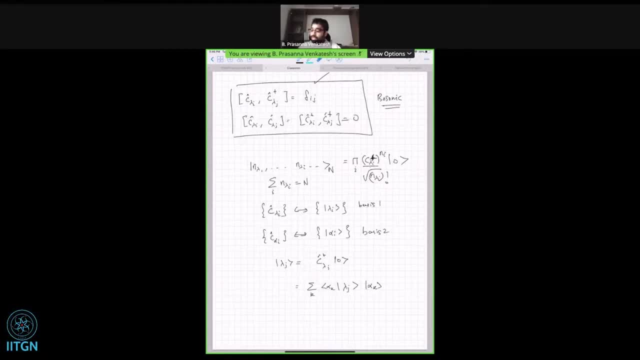 I'm allowed to expand it in that basis. Now, if I write this alpha k as just c dagger, alpha k, zero, Right, My life is set And I can basically compare this object to this object. Right, And I can get basis change relations. 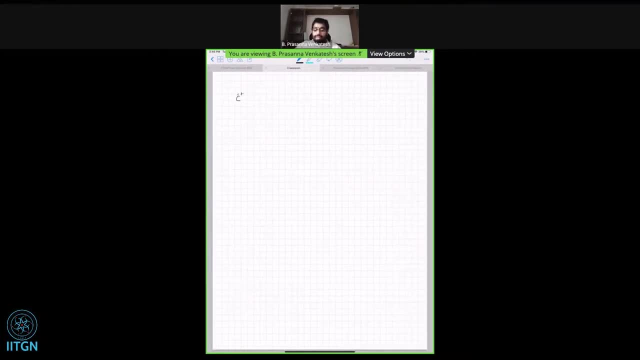 So basis change relation for creation operators c dagger- lambda j is sum over k alpha k, lambda j, c dagger alpha k. This is for two sets of orthonormal basis, alpha k and lambda, And from this you can also invert and write c dagger alpha in terms of c dagger lambda. 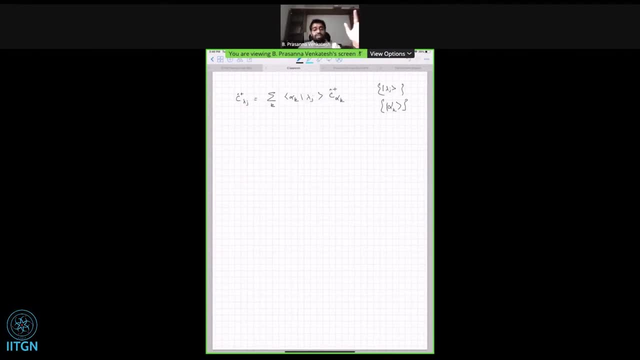 OK, So in this way creation of one can actually write creation annihilation operators. You can write creation annihilation operators in any basis that you want. Now, creation annihilation operators in the continuous position basis: OK, They are extremely important because, especially from a field theory point of view, think of 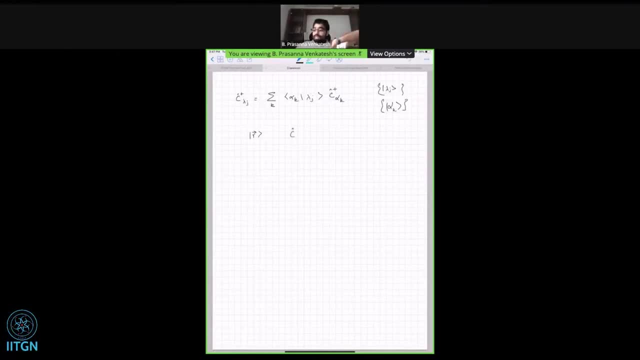 what they are. So if I write basically, and creation operator at position r, this operator actually creates a particle at some position r. So these are somehow have a slightly more special status And they are given their own symbol And they are basically called field operators, as you might have heard, of psi, of r and psi. 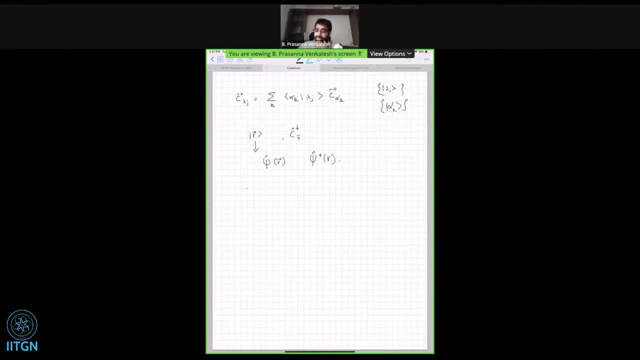 dagger of r And very quickly you can write in some any arbitrary orthonormal basis. Psi of r is precisely sum over k? r lambda k, c lambda k Right. Similarly, psi dagger of r, sum over k r lambda k r, c dagger, lambda k. 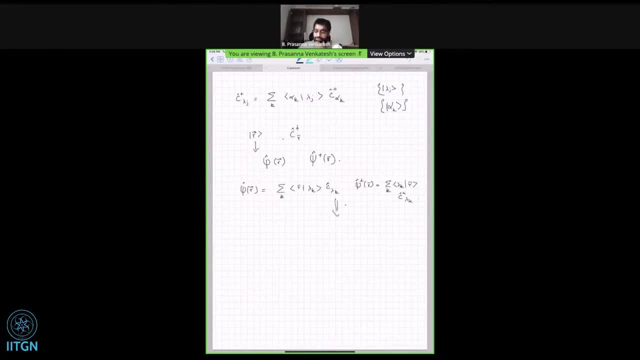 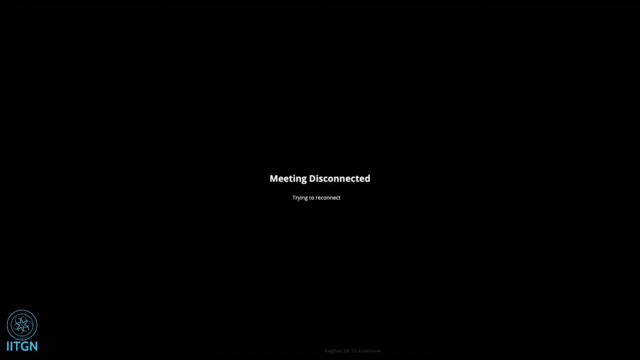 OK. So now, as a result of these definitions and the fact that this r basis is a non normalizable or delta normalized basis with continuous elements, We can write down Form For the field operators And it is written in this form. OK, 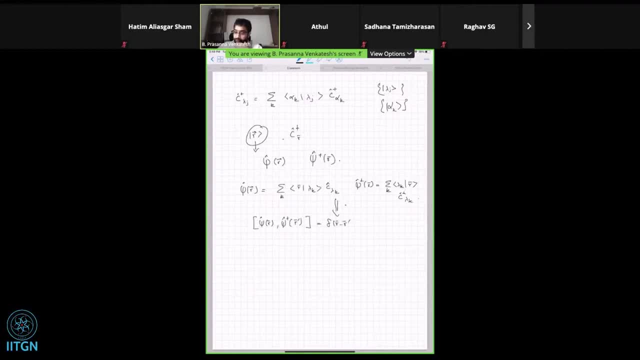 So this is a very important relation that tells you about the both of these fields. OK, So with this let us get a little bit of sense for really what this single particle field operator is. Very, That is, it has an intimate relation in some sense to the position space or single particle. 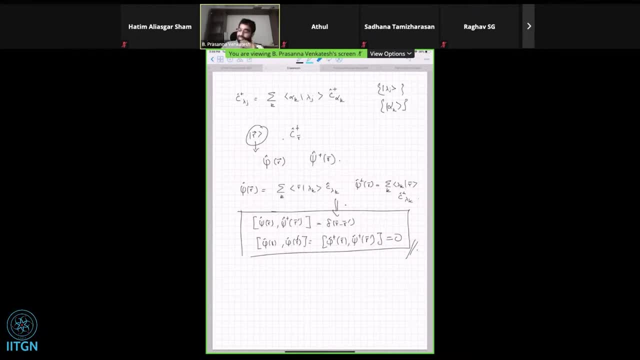 wave function. So let's actually see this relation. So now r lambda, If you remember, is the wave function of a single particle In the single particle state lambda? OK, Now remember that r is nothing but psi dagger of r applied to the vacuum. 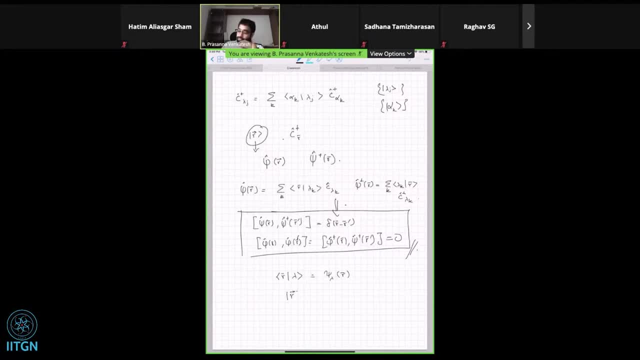 Right. So now, if I use this relation, one sees this very interesting connection between the wave function and the field operator. OK, In some sense, This sort of relation, This is a very interesting relation. OK, So So So. 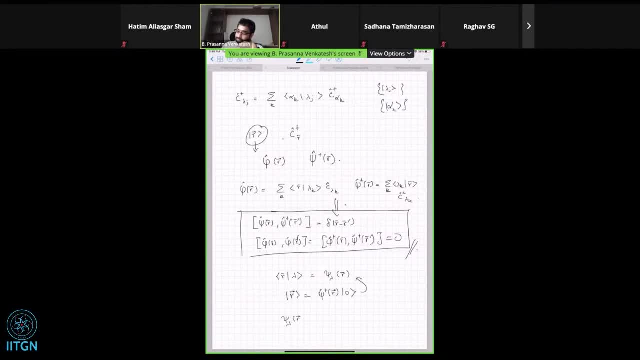 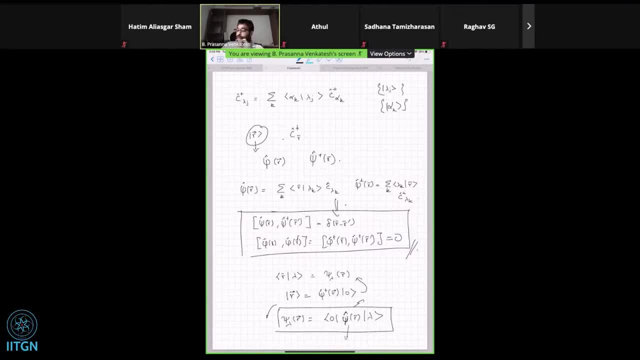 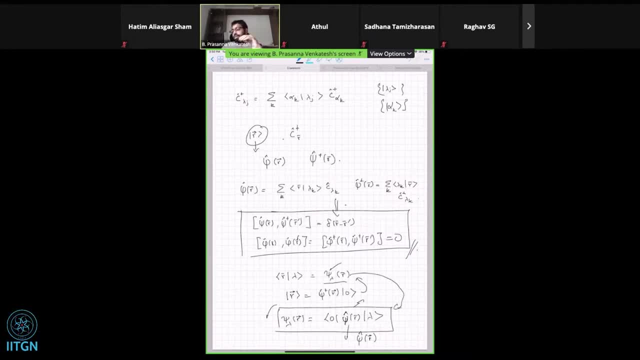 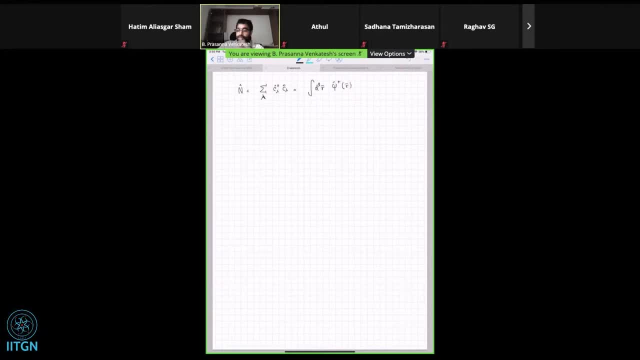 field operators. it is precisely psi, dagger of r, psi of r, integrated over all position. so this is like an operator for local density of a gas of atoms. okay, so now, in principle, we will always work in some space that has a fixed number of particles, eventually but but which means we are in an eigen. 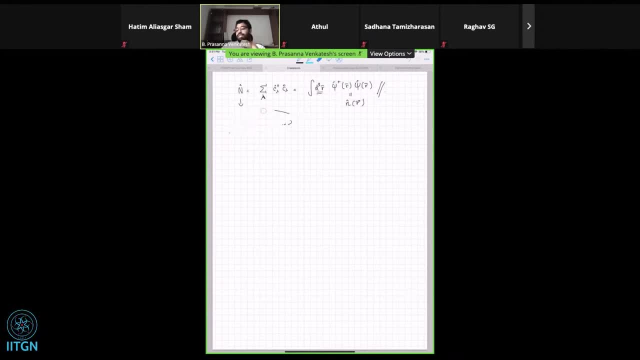 state of the number operator. for all states that are a fixed particle number are eigen states of the number operator. okay, good, so we've explained now what is second quantization. in order to just finish up here, i want to very quickly write down: how do single and many particle operators in an 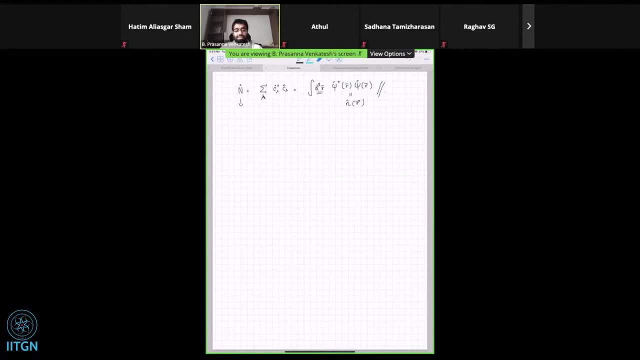 n particle system. look like in this second quantized representation. for example, a very important single particle operator of an n body system are operators of the form: sum over i runs from 1 to n. small o i. small o i is a ordinary single particle operator and it acts on the ith particle in your system. 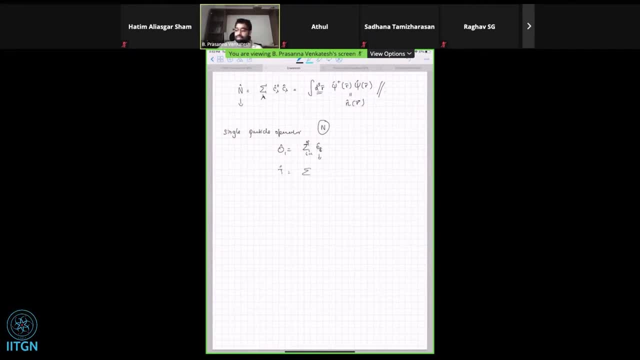 with n particles, for example, k kinetic energy is one such operator. right, this is the kinetic energy operator for n particles. similarly, potential energy is precisely one such n particle. uh, one such one body operator. these are all called one body operators. they are just operating particle by particle. okay, now i'm not going to prove this. 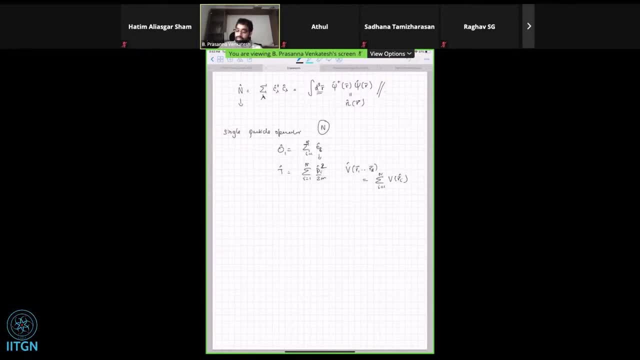 one can show that in this second quantized representation you can always write a one body operator in this manner: sum over j a a dagger, lambda k, a lambda j, lambda k, o, lambda j, lot here. here is theонь. OK, Now of course you're not referring to individual particle labels, because we are. 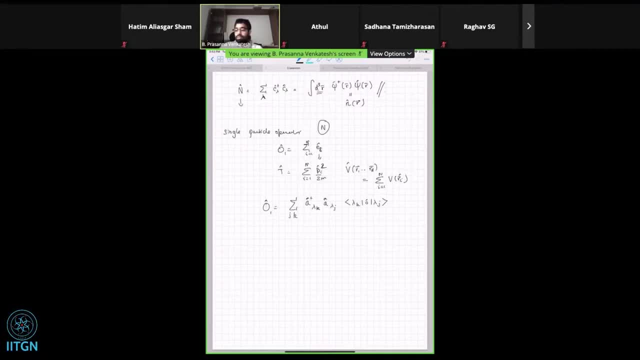 interested in writing them in this Fock basis or in terms of this creation and annihilation operators. So lambda k is some arbitrary single particle basis. This O is precisely the single particle operator whose sum gives the total operator O, And this is how one writes it out. 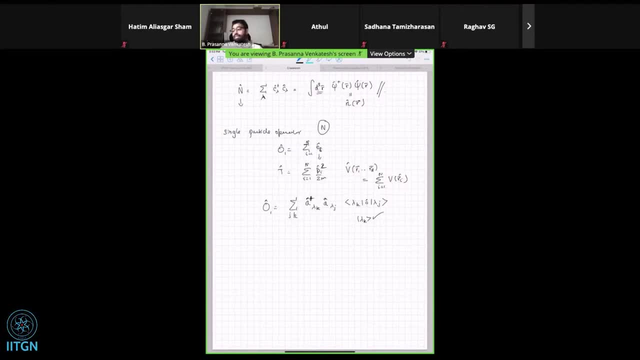 So this is a dagger, and a are the creation and annihilation operators in lambda k, lambda j. OK, And for the case when your operators are the field operators, when your creation and annihilation operators are field operators, one can write a continuous version of this. 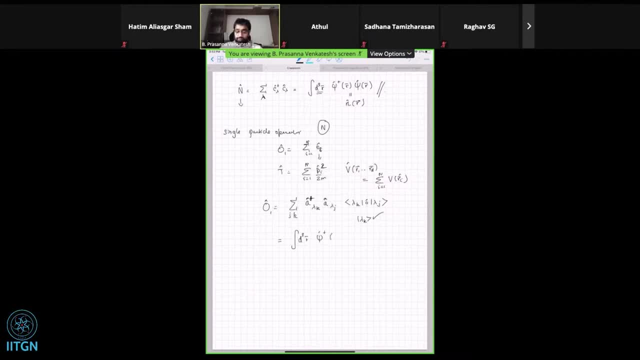 as psi dagger of r, So so so. so I mean this is the general case. Now let's consider two most important operators that you're interested in. Let's take the kinetic energy operator and some potential energy operator. When you write it in the field annihilation, creation, operator approach.